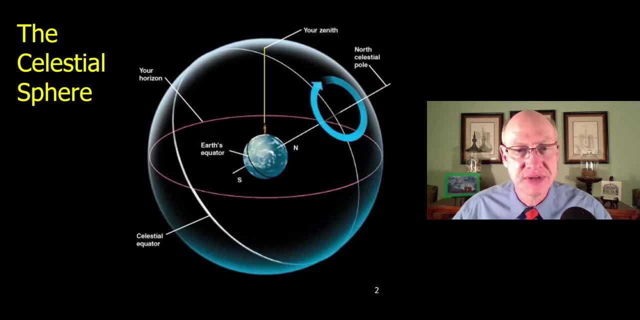 we get the north celestial pole up there in the celestial sphere. If we extend the south pole out into space, we get the south celestial pole, And if we extend the Earth's equator out into space, we get the celestial equator right there. 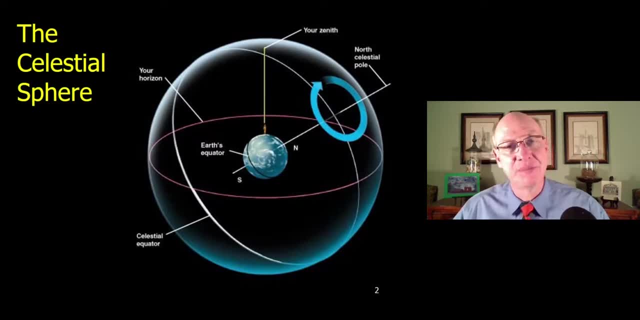 So this outcome, with the celestial spin on the Earth, is part of our расскlxico study of the sphere, represents the celestial sphere, this artificial construct that you can imagine, all of the stars and the planets and the Sun and the moon and everything being sort of painted on the inside of this sphere and what we usually depict. 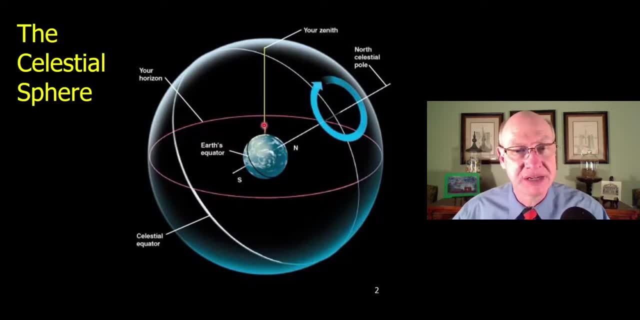 is, even though we know it's not true, is we usually depict ourselves standing straight up and down, perfectly still, and that it is the celestial sphere that is rotating over our heads, rather than what's truly going on, which is the stars being in various distances and and sitting, for the most part, still as the 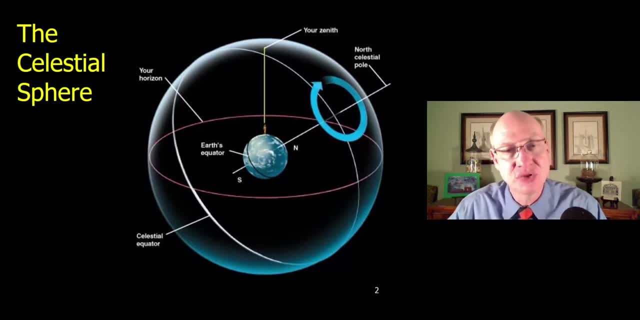 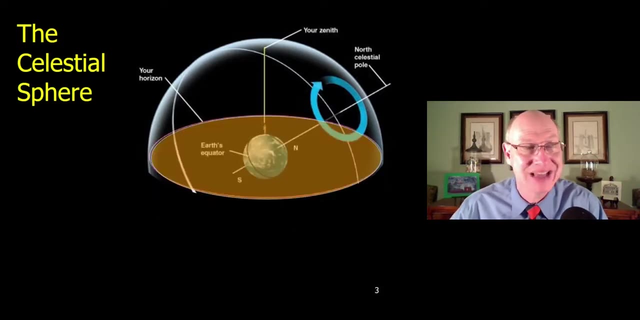 earth rotates around from west to east. so this is the celestial sphere, the idea of the celestial sphere. now, you can't see the whole celestial sphere at one time. in fact, the earth blocks half of the celestial sphere from view. so what you can see at any one time is just the head, the top half of the celestial. 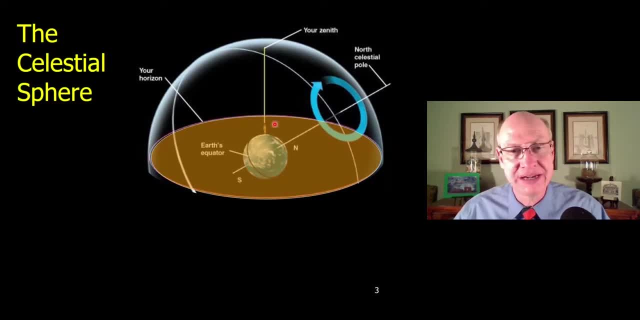 sphere. this orange circle that I've drawn in here represents your horizon. you can see everything above your horizon, but you can't see anything below your horizon. so let's talk about those points here for a second. the north and south celestial poles, the celestial equator. the north celestial pole is 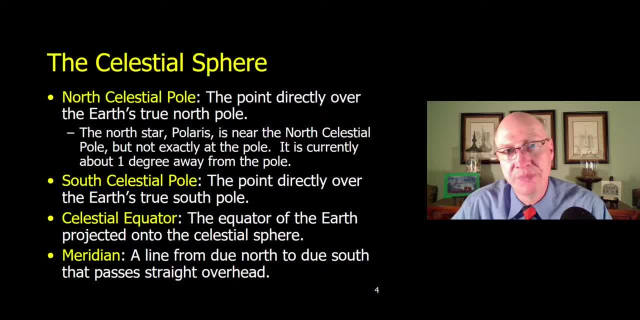 simply the point directly above the Earth's true North Pole and, as we've seen before when we were talking about the night sky, the north celestial pole is marked by a model, moderately bright star. its name is Polaris, the North Star or the pole star, and Polaris is not exactly at the North Pole. it's about a degree away from the 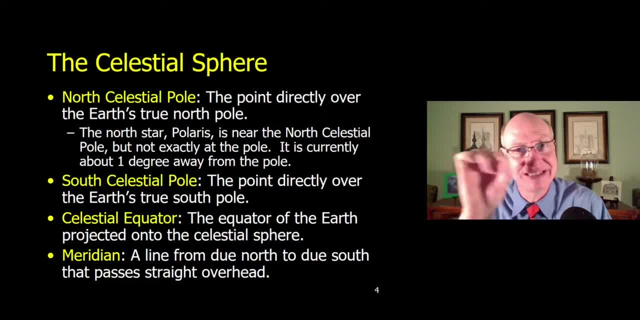 North Pole, which means, as the night goes on, Polaris makes a little tiny circle in the sky as it circles around the pole up there. the south celestial pole is is is the point directly above the Earth's South Pole and, as we saw in a previous lecture, that does not have a bright star marking the south celestial pole. and 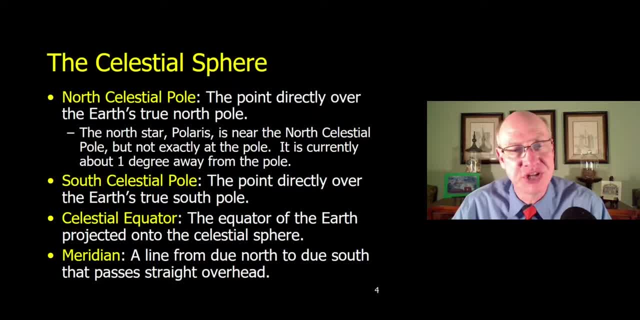 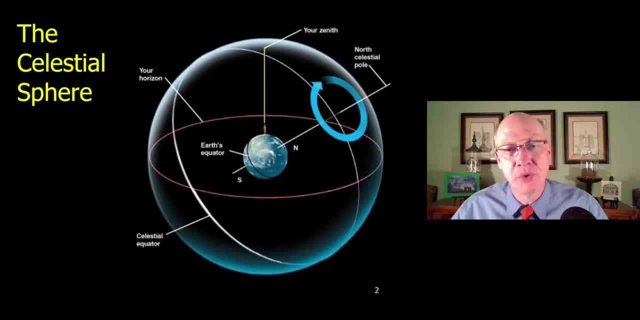 the Englishuguadra alchemy Network. The blue square on the left is the polar light Sesh, the Crane ako na, and then the celestial equator is simply the equator of the earth projected out onto the celestial sphere. one last line that we want to draw is your meridian. 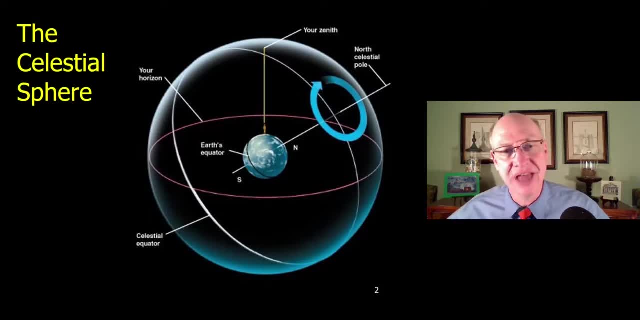 your meridian is a line that goes from do north to do south and it passes through your zenith. right here in your meridian is a line that cuts the sky half and a northern half, and your meridian, which is running north to south through your zenith. 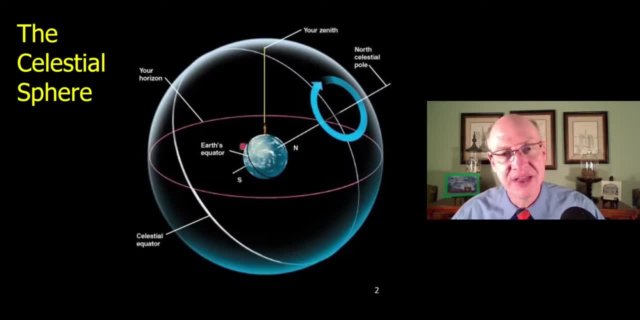 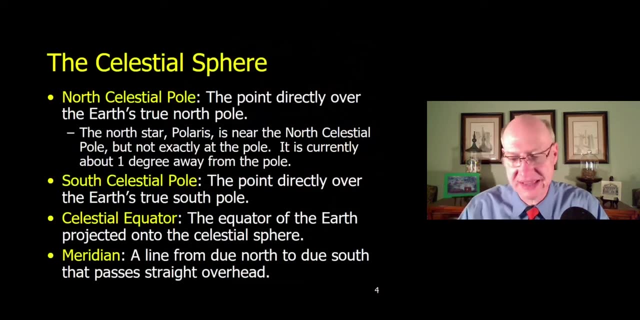 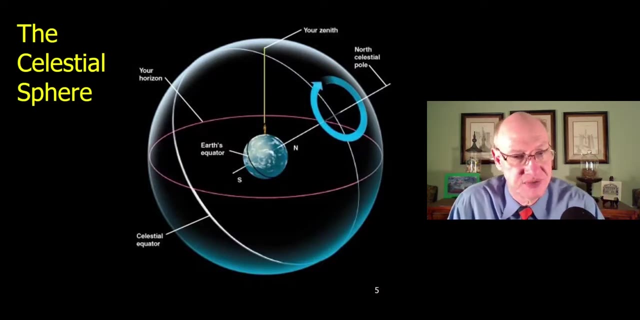 is cutting the sky into an eastern half and a western half over there. so that is the your meridian up there in the sky. so those are some of the key features of the celestial sphere. now, i'm not very good at drawing three-dimensional celestial spheres like this. 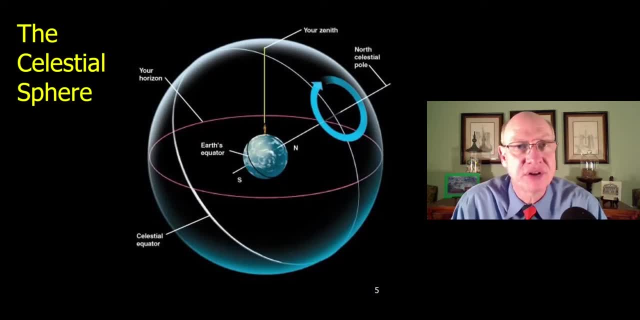 uh, i think, uh, but i think, in order to understand what's going on in the night sky, how the sky appears to us, how that appearance changes as we change our place on the location of the earth, change our latitude on the surface of the earth, how the objects move through the sky, in order to 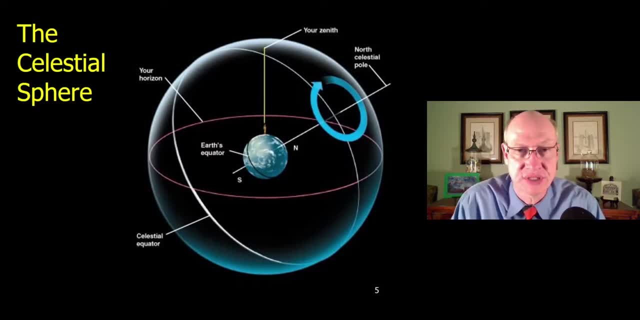 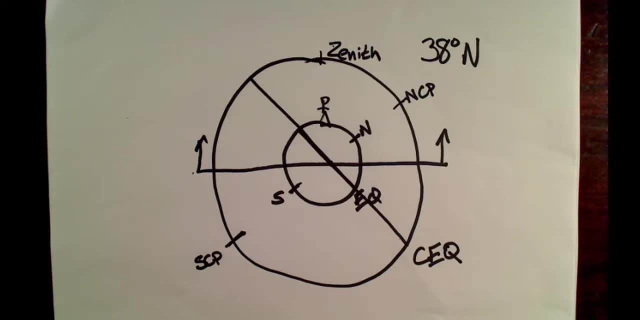 understand all of those, we have to draw some celestial spheres- so the celestial sphere is a depiction of the sky above our heads- and to understand why the celestial sphere appears the way it does and how our view of the celestial sphere varies as we move on the earth and change our latitudes. 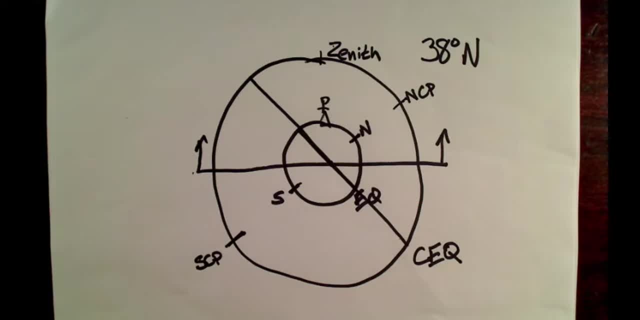 we need to be able to draw celestial spheres for observers at different latitudes. now, i'm not very good at drawing three-dimensional celestial spheres like the artwork that you've seen in the lectures, so what i'm going to teach you today is a technique for drawing a very simple 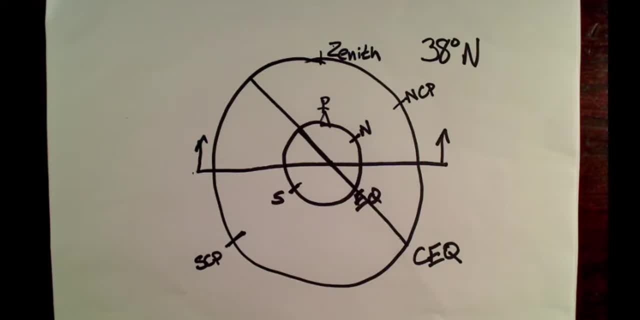 two-dimensional celestial sphere, and what i mean by a two-dimensional celestial sphere is we're seeing the celestial sphere edge on. Instead of the equator being a curved circle that goes around the sky, we're going to see the equator edge on like this. So, instead of seeing it in perspective, we're going to see it. 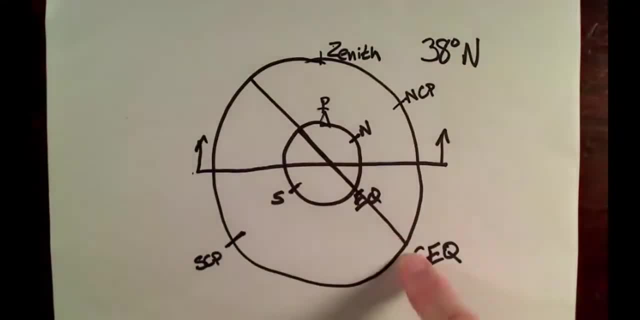 edge on so that that circle looks like a line cutting across the sky. Now, these two-dimensional celestial spheres have a lot of great uses. We can not only use them to determine, for example, where the pole appears in our sky and where the celestial equator appears in our sky. 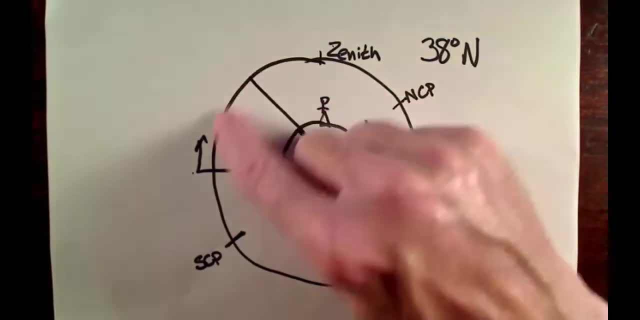 but later in the semester we will use them to determine where the sun appears at different times of the year, how the stars move across the sky, depending on how far north or south they are of the celestial equator. So these celestial spheres are very, very useful for understanding. 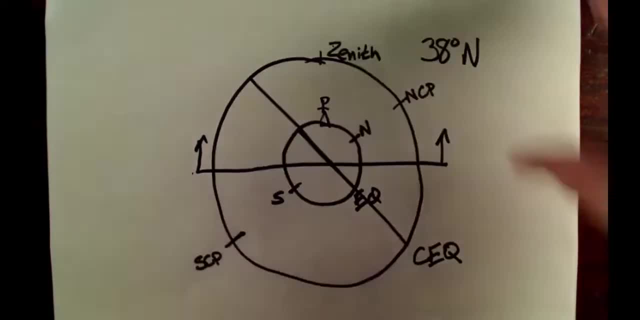 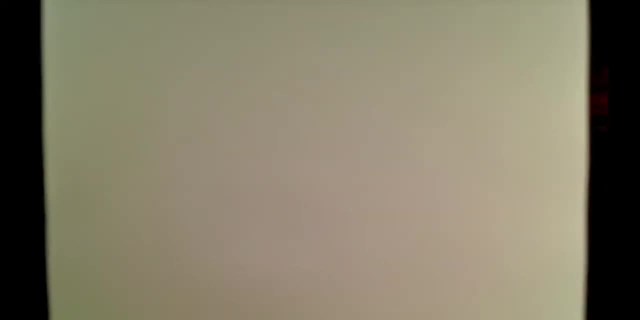 our view of the sky, And in order to do them, we need to learn how to draw them. So let's go ahead and get started, And let's start with a simple celestial sphere, where we start with the basic orientation of the earth. 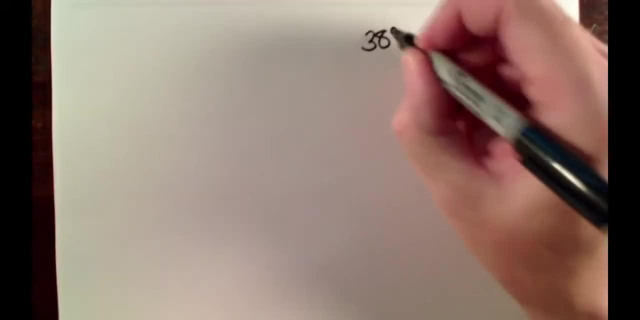 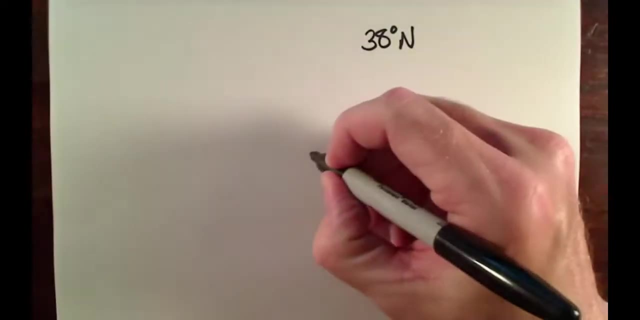 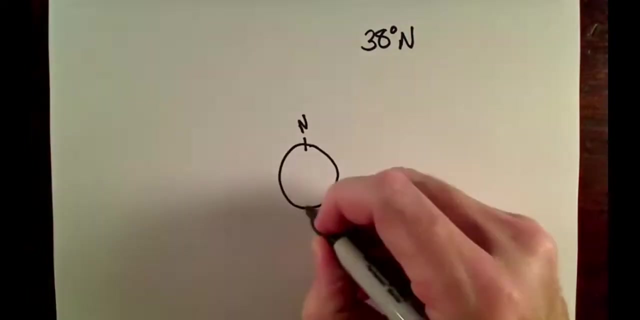 So let's draw a celestial sphere for an observer at 38 degrees north latitude. That is the latitude that we have here in Charlottesville, Virginia. So I'm going to start by drawing the earth, And now that I have the earth on there, let me draw the north pole, let me draw the south. 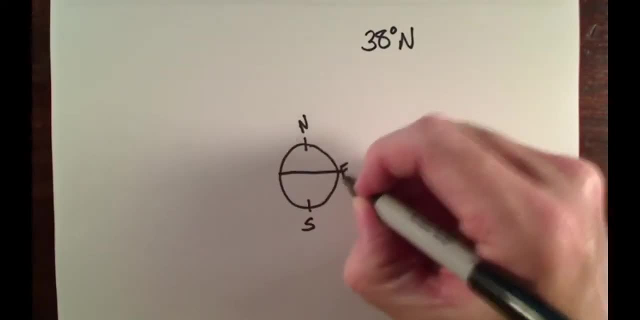 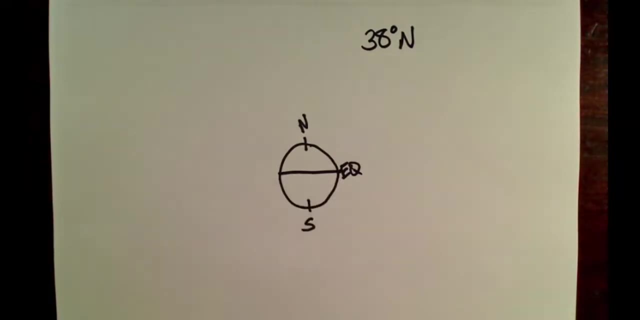 pole and let me draw the earth's equator. Of course, whenever we draw the earth, we're going to draw the north and the south poles opposite one another and the equator runs across the middle at a right angle. So I'm going to draw the north pole at a right angle to them. I typically like to depict poles using little. 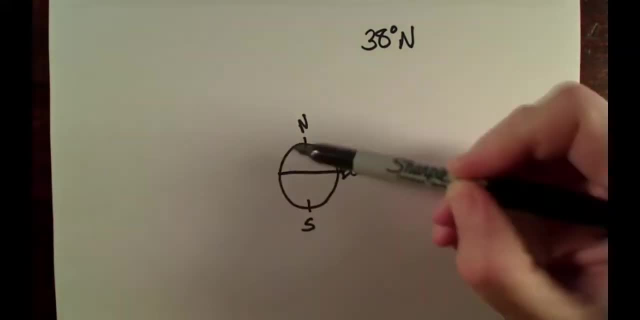 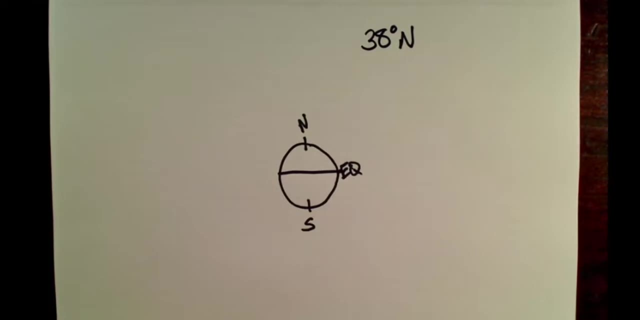 marks like this and something like the equator as a full line. You're welcome to draw a full line for the north and south poles. Whatever you want to do is fine with me, But this is the technique that I like to use Now for our observer at 38 degrees north. we need to locate them on this globe. 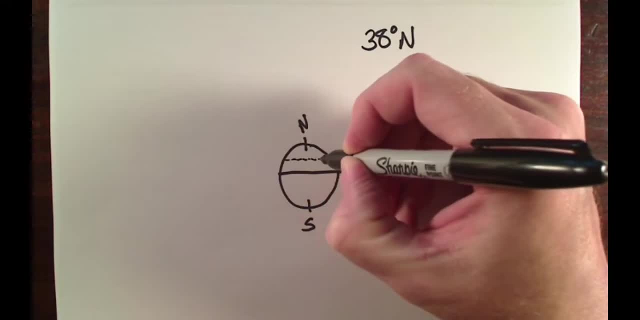 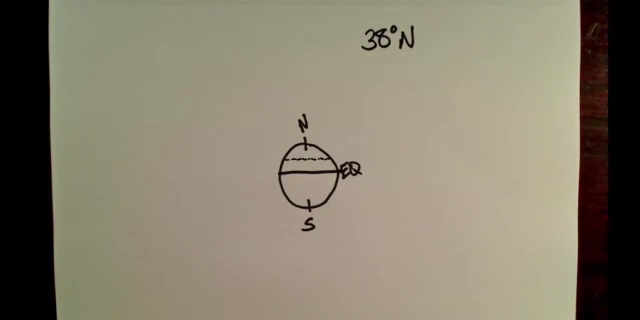 And a latitude of 38 degrees north is about here on the globe, That is, anywhere along this dashed line, at a latitude of 38 degrees. So we could put our observer anywhere along that dashed line, And the reason it doesn't make a difference where we put them is because of the rotation of the 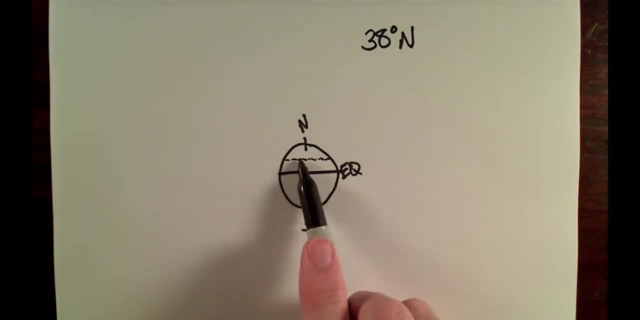 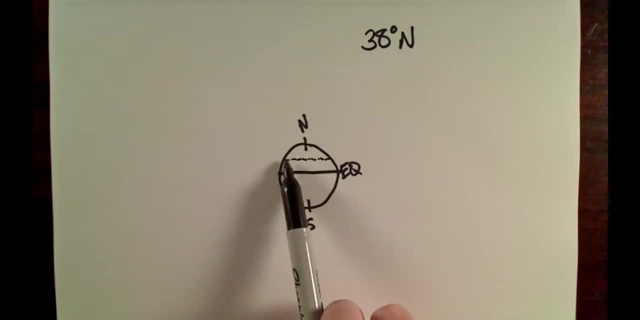 but it does not change with longitude As the Earth spins like this, as the earth rotates, they're just carried around, So I can put my observer anywhere on this line of latitude. I'm going to go ahead and put them over here on the. 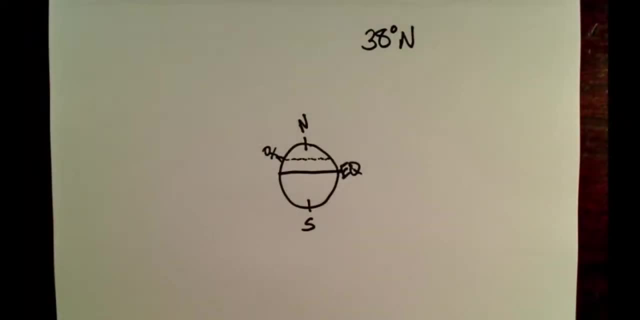 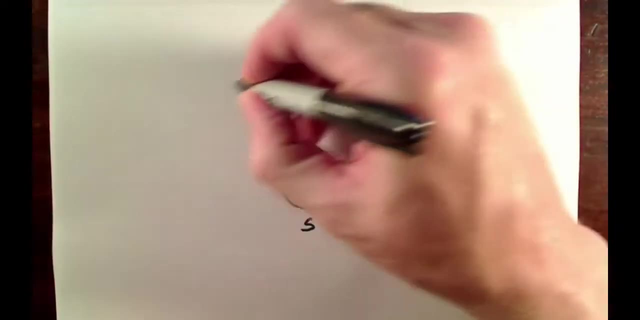 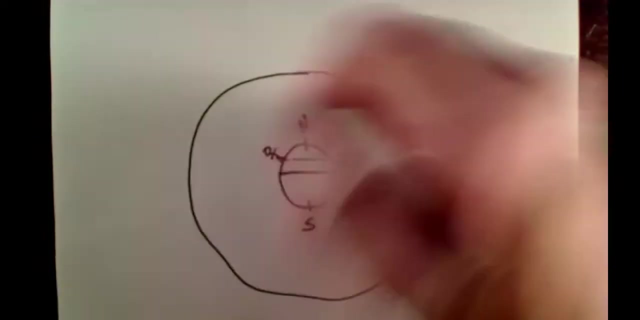 edge, Looking like that right now. So that's where our observer is, at 38 degrees north latitude. Now I need to draw the celestial sphere. So now let me draw the celestial sphere around the earth like that. and the celestial sphere- of course it should be round. Sorry, I'm not. 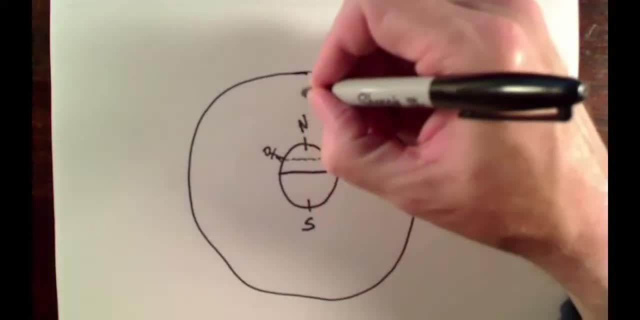 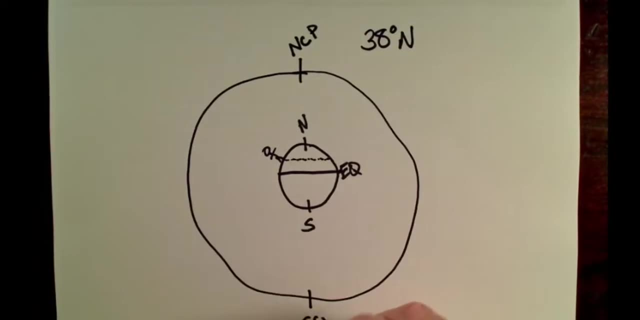 good at drawing a circle. Now we can extend the Earth's North Pole out into space to get the North Celestial Pole. We can extend the South Pole into space to get the South Celestial Pole. We can extend the Earth's equator out into. 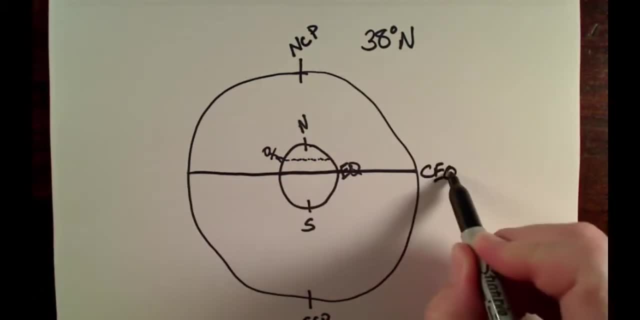 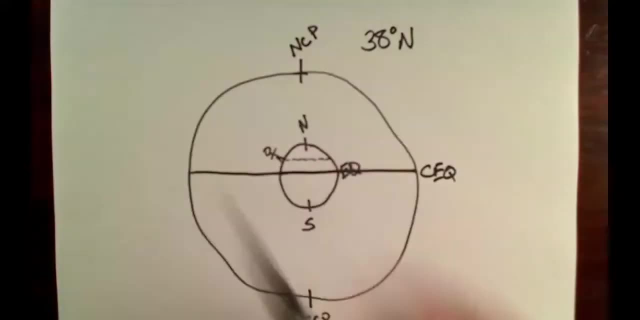 space to get the Celestial Equator. And then, finally, for my observer right here, they can't see the whole celestial sphere. They can only see the part of the celestial sphere that is above their horizon. So let me go ahead and draw in. 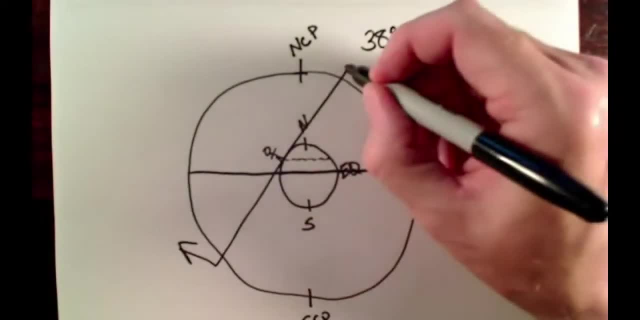 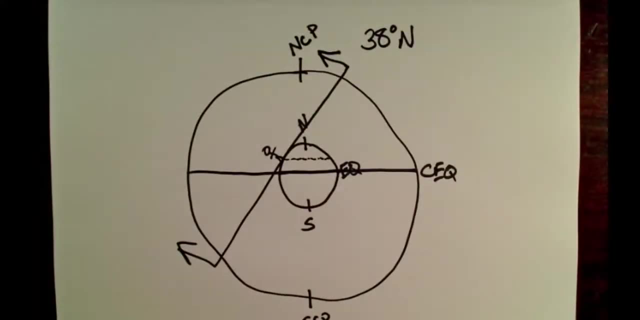 their horizon And they can see everything above this horizon, but they can't see anything below the horizon. That is, everything below the horizon is hidden from view. Now, the problem with drawing the celestial sphere like this is that our observer is tilted over And nobody views themselves as living on the 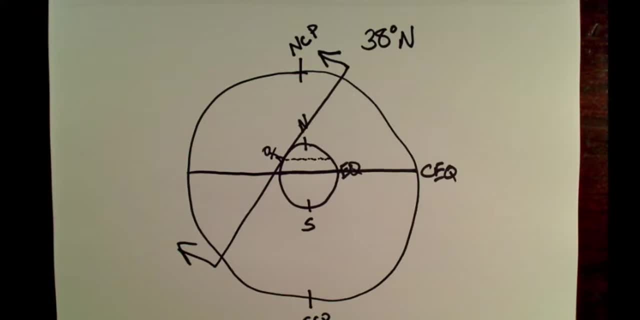 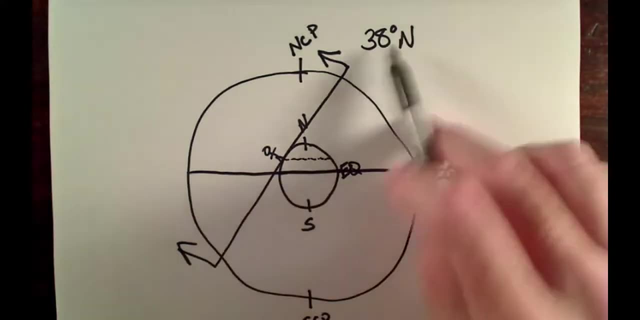 Earth tilted over like that. When you talk to somebody that lives in Australia, they don't see themselves as standing upside down on the Earth, They see themselves as standing straight up and down Here at 38 degrees north. I don't picture myself living my life tilted over like. 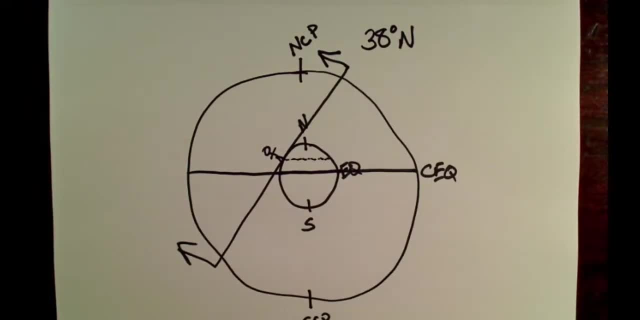 that I picture myself standing straight up and down. So if I want to understand how the celestial sphere is going to look to me, I need to rotate my celestial sphere so that my person is straight up and down, Because now that the person is, 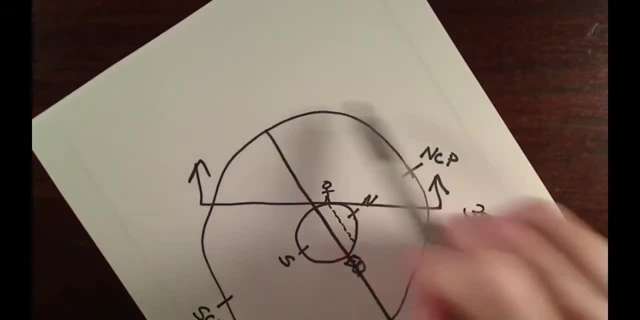 straight up and down. this is how we view the world. This is how we view the sky as a dome over our heads. Now the horizon is horizontal, just like the real horizon is, is, And now we can understand how the equator appears in the sky, where the 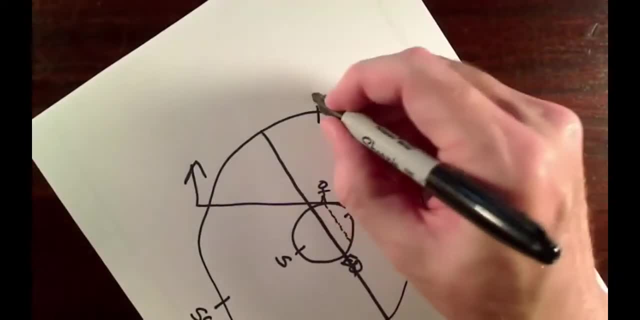 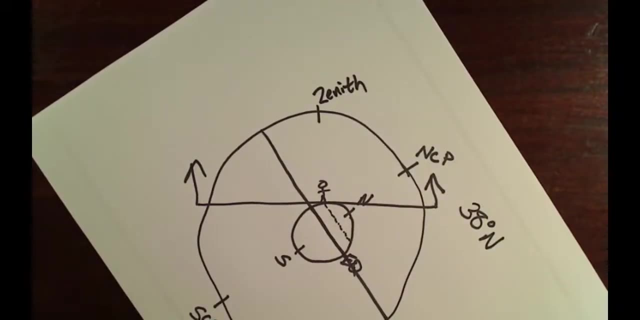 North Celestial Pole is in the sky where our zenith, the point straight overhead, appears in our sky, And it is much easier to picture the sky when it's tilted over like this than it is when we use the basic orientation of the Earth. The 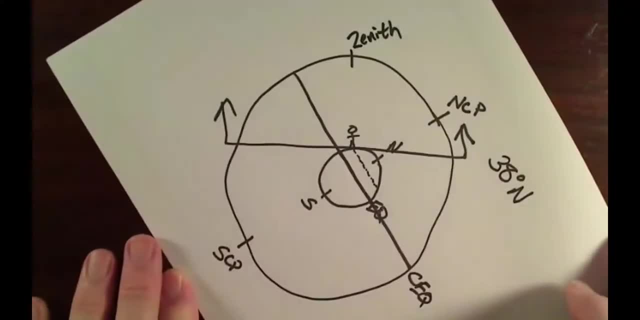 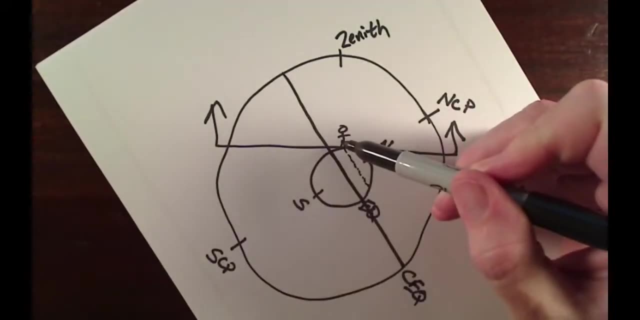 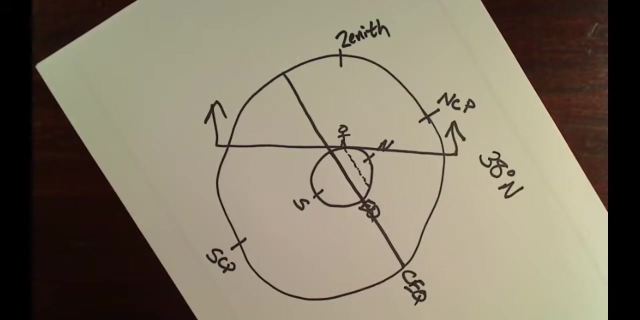 problem with drawing the celestial sphere like this is that we have to orient the Earth underneath our observer. That is, we're always going to draw the celestial sphere with the observer on top, and that makes it difficult to think about the orientation of the Earth underneath the observer. So before we get, 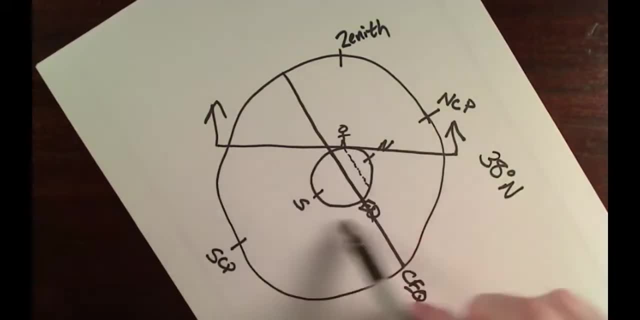 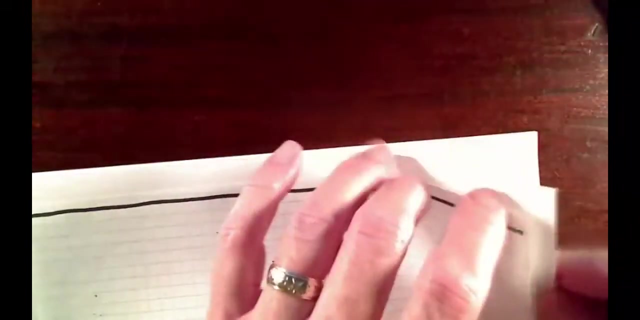 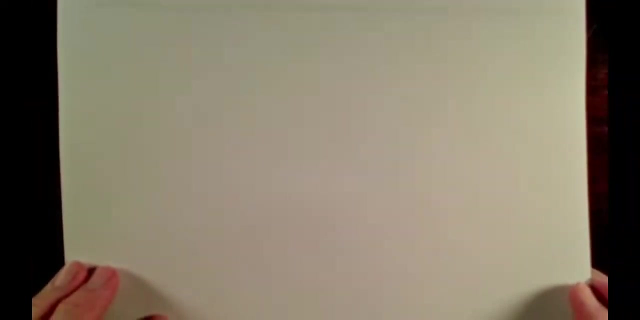 into drawing celestial spheres. let's practice drawing the Earth, with the observer always on top for observers at a number of different latitudes. Okay, so let's go ahead and get started on that, All right. First observer I'm going to draw is: let's draw somebody again at 38. 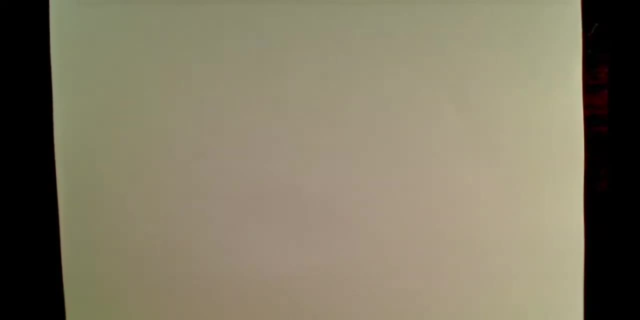 degrees north latitude. So we'll draw somebody at 38 degrees north latitude. So here is. so let me draw here 38 degrees north latitude. So what does it look like for an observer standing on the Earth? We draw in the Earth to begin. 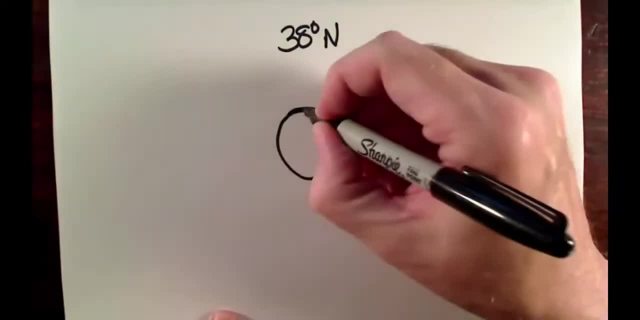 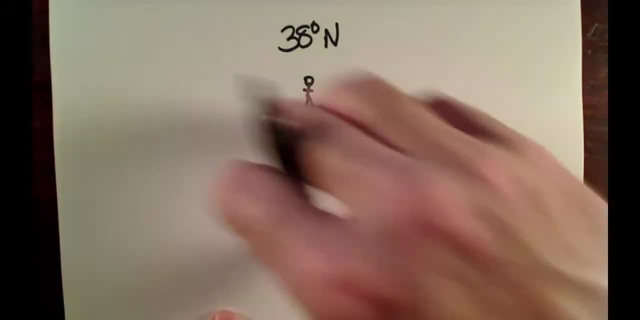 with. and then the second thing we do is we draw our observer standing on top of the Earth, of the Earth right there. And now we have the hard part, the hard decision of deciding how we're going to orient the Earth under it, so that they end up at. 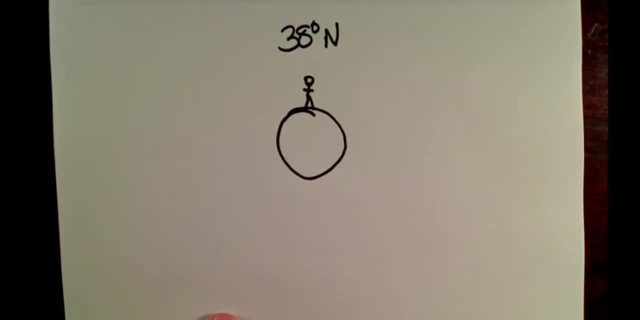 the right latitude. So I need to draw on here the North Pole, the South Pole and the Earth's equator. Well, to draw the North and the South Pole on here, I have to remember that my observer is not standing at the North Pole, so the North 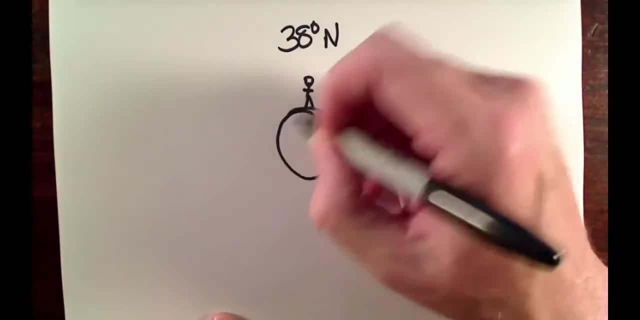 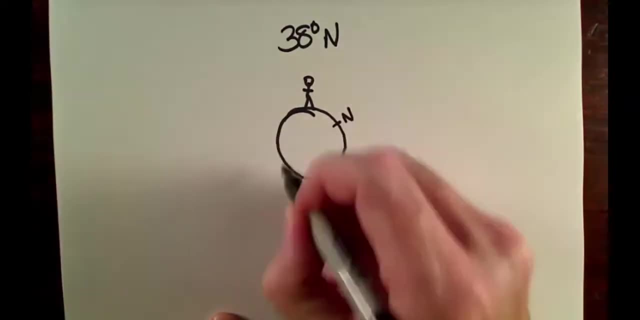 Pole is not below their feet. The equator is not below their feet. In fact, at 38 degrees North, they're about halfway between the equator and the pole. So what I'm going to do is put the North Pole over here, put the South Pole over here. 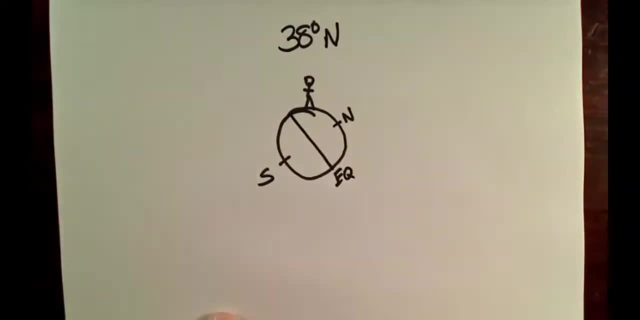 and draw the Earth's equator like that. So now I've got my observer standing straight up and down, You'll see that they are about halfway between the equator and the North Pole, and so this is somebody standing at 38 degrees North. 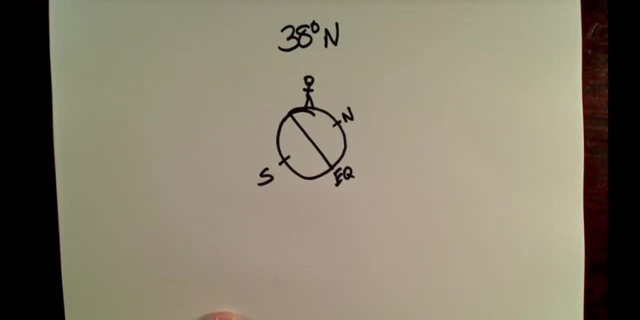 latitude And this is how we will begin our celestial spheres. But before we start drawing the celestial sphere, let's practice orienting the Earth like this for people at a couple different latitudes, Let's move on. Let's try somebody over here at at 90 degrees North latitude, That. 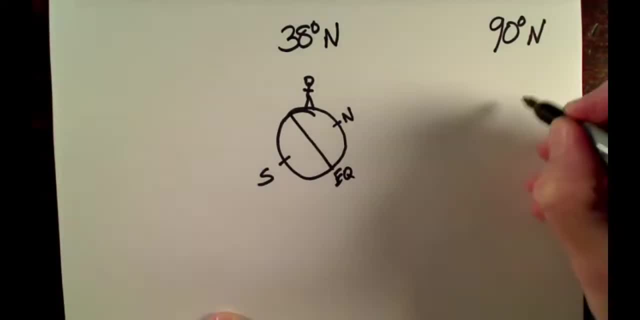 is somebody standing on the North Pole? What would that look like For somebody at 90 degrees North latitude? I draw the Earth, I draw my observer standing straight up and down, and now I need to draw the North Pole of the Earth, the. 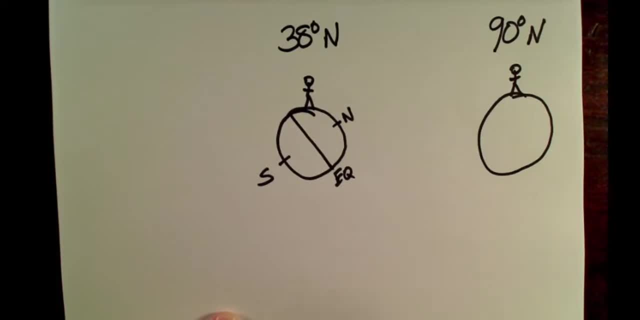 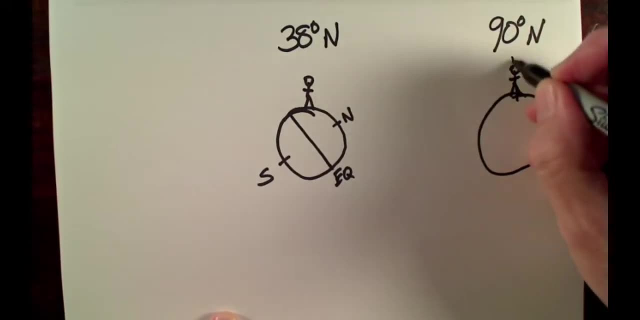 South Pole of the Earth and the Earth's equator. Well, it's fairly easy. now, At 90 degrees North, I know that I'm standing on the North Pole. So right below my feet, right here, I can draw the symbol for the North. 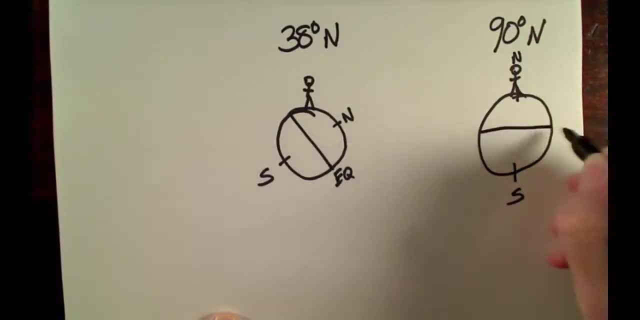 Pole, This is the South Pole and there's the Earth's equator. like that, For someone standing on the North Pole, that is what a celestial sphere looks like. Now let's draw a celestial sphere for someone at, say, the equator at zero. 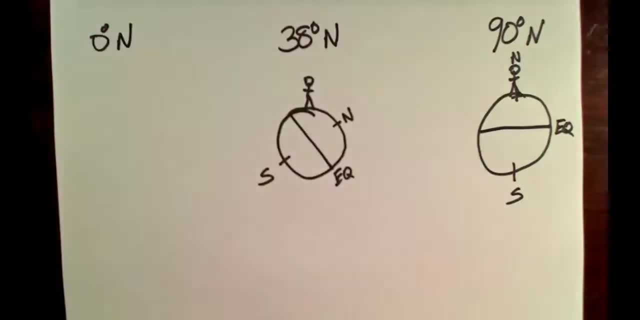 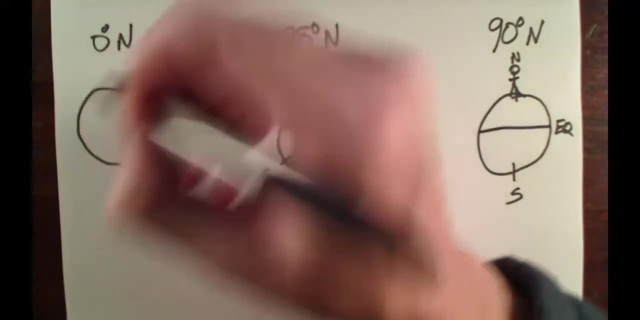 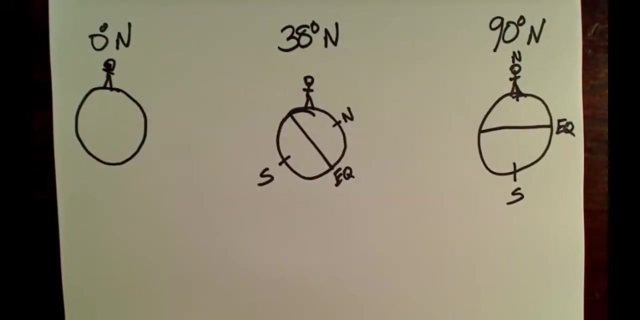 degrees North latitude. So what would that look like? Well, at zero degrees North latitude, let me draw the Earth. I will again draw my observer standing on top of the Earth, because they always picture themselves as standing straight up and down. And now we need to. 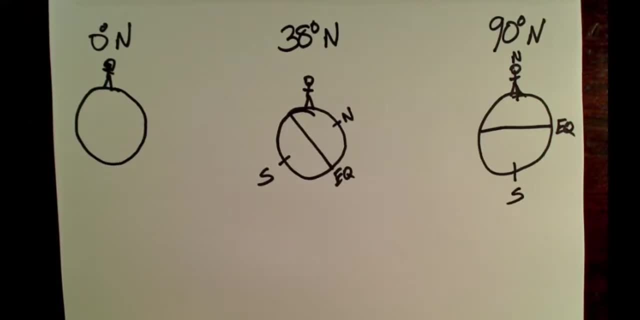 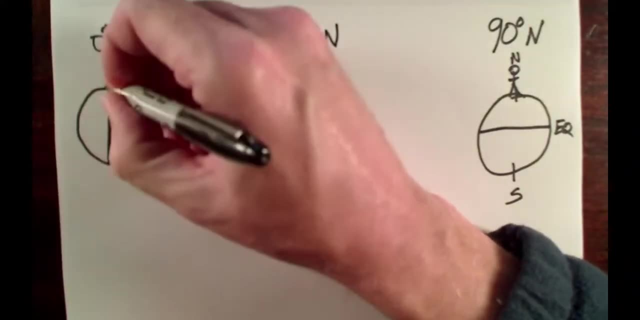 orient the Earth underneath my observer. So how will I go about doing that? Well, at zero degrees North latitude, I'm standing on the equator, which means I draw the equator in like this Right, Because I'm standing on the equator. 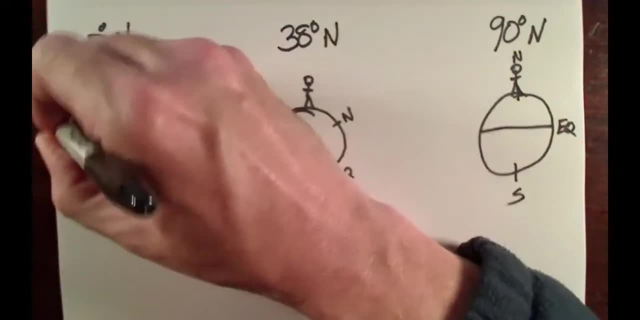 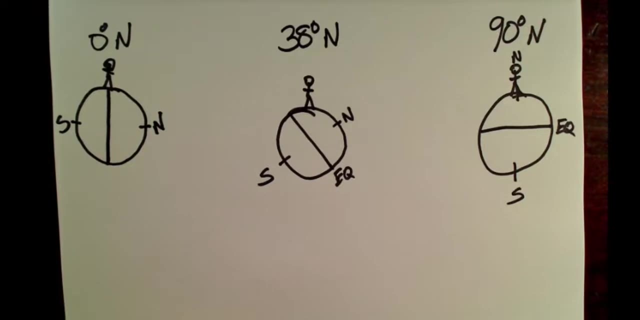 And if that's the equator, that means that this is the North Pole and this is the South Pole over here. Okay, So that's how we would orient the Earth For an, an observer standing on the equator. Now, in all three of these, or at least for these two. 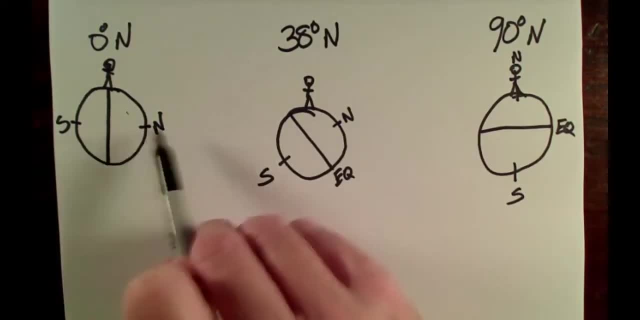 it doesn't matter whether I put, for example, in this case, it doesn't matter whether I put the north pole here or the south pole or the north pole over here. I could switch the two poles when they're standing on the equator. In this case, I could have drawn the equator tilted. 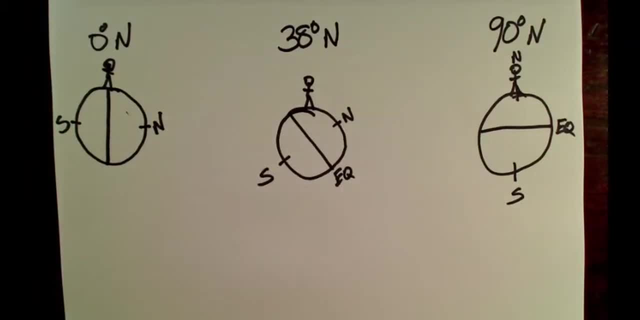 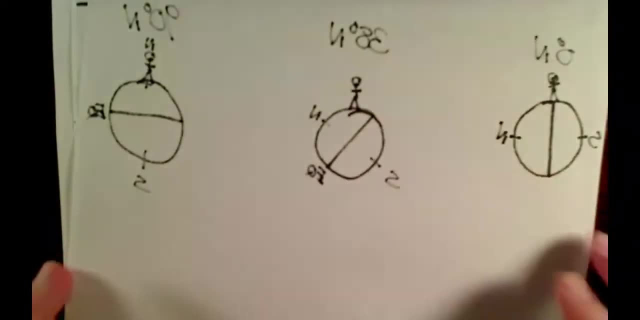 differently, with the north pole over here and the south pole over there. It doesn't matter if you draw it this way or you draw it as viewed from the other side, like this, with this being the north pole over here and the south pole and the equator running like that. Either of those 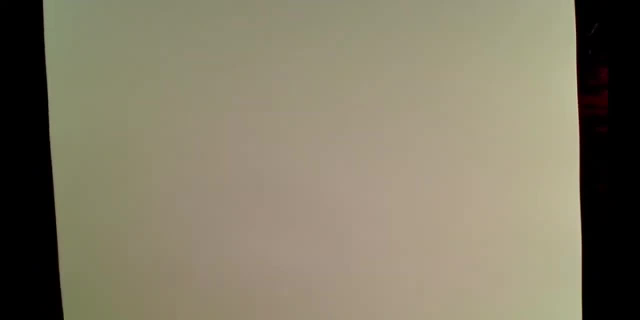 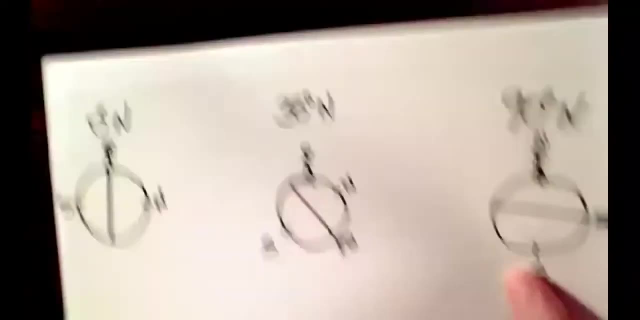 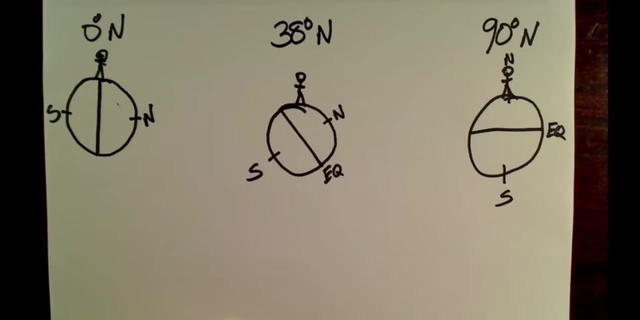 are a perfectly valid way to draw it. I am in the practice of typically drawing these with the north pole on the right-hand side. So typically when I draw my celestial sphere diagrams, I'm going to put the north over there on the right. So those are three different ways to draw the equator. 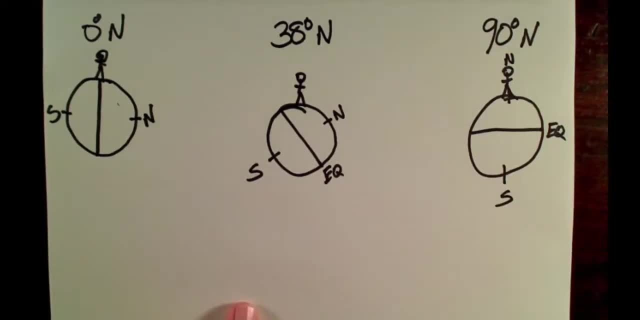 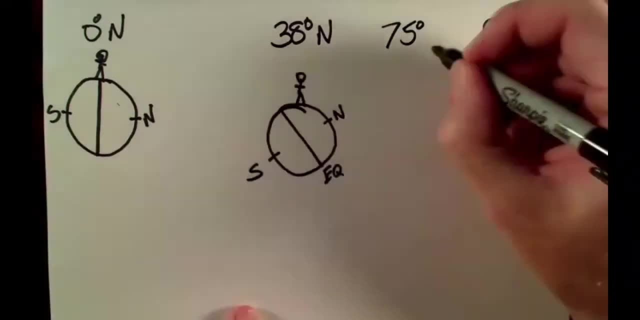 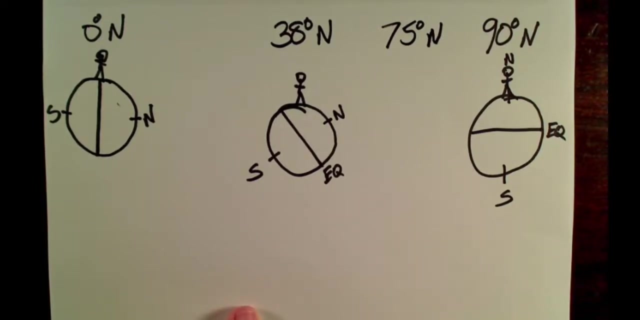 Different latitudes. Why don't we go ahead and practice one for another latitude, Let's do. let's say, 75 degrees north. So what does a celestial sphere look like for somebody at 75 degrees north? You're welcome to pause the lecture at this point. In fact, why don't you do that? 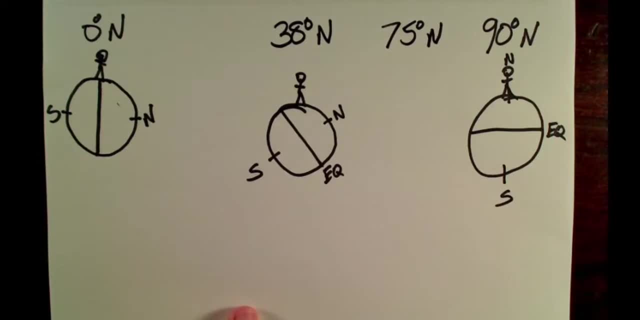 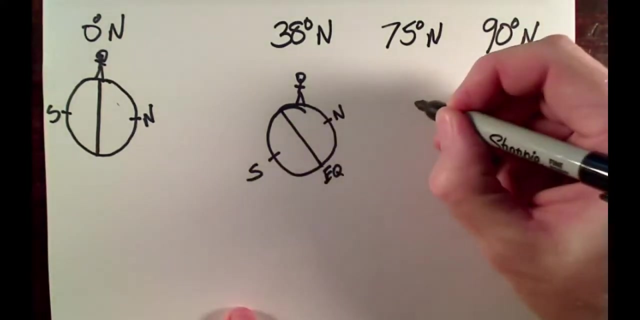 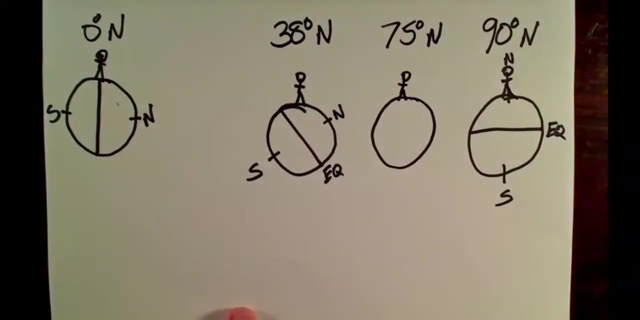 Pause it. And why don't you draw the earth for an observer at 75 degrees north? Okay, Welcome back. Let's see how you did. So first thing I'm going to do is I'm going to draw the earth, Okay, And I'm going to draw my observer standing on top of the earth. Notice that I always 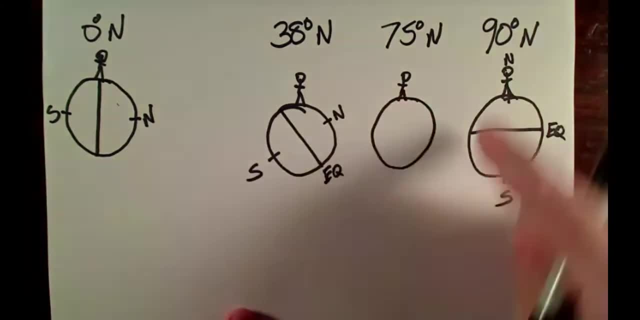 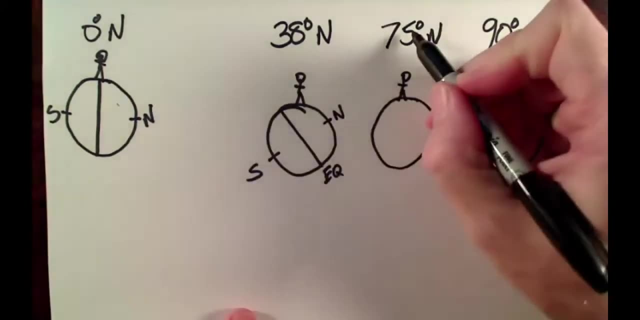 do it exactly the same way. I always draw the earth, Then I draw my observer standing on the earth, And after that I orient the earth underneath my observer For 75 degrees north. I know they're not standing on the north pole, So I'm not going to draw the north pole between their 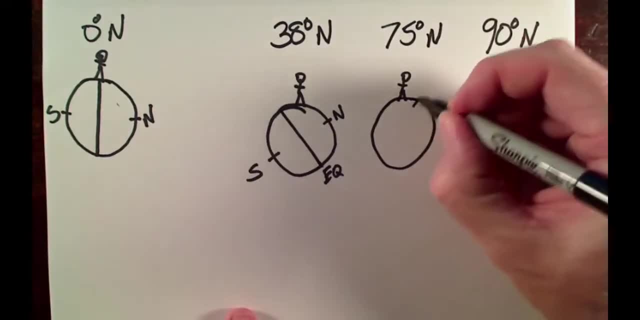 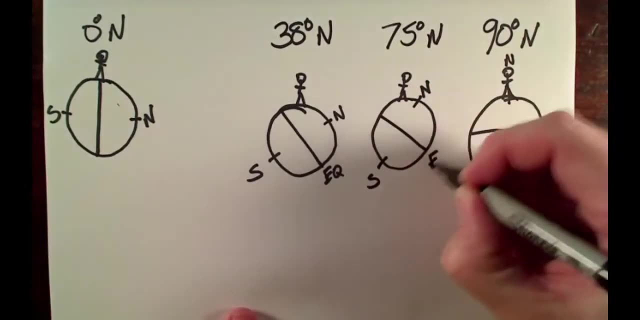 but I also know they're not very far away from the north pole. So I'm going to draw the north pole fairly close to my observer, which means the south pole is here, which means the equator is running like this. Now, when I look at my observer, I see that they are closer to the north pole than 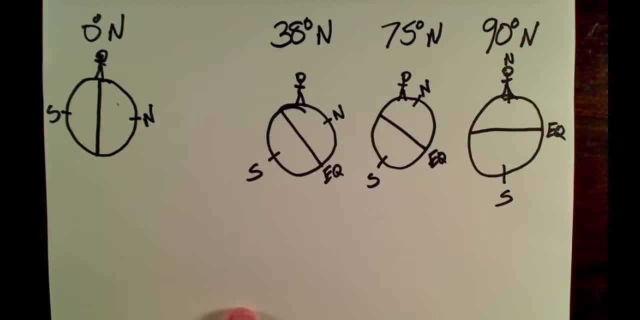 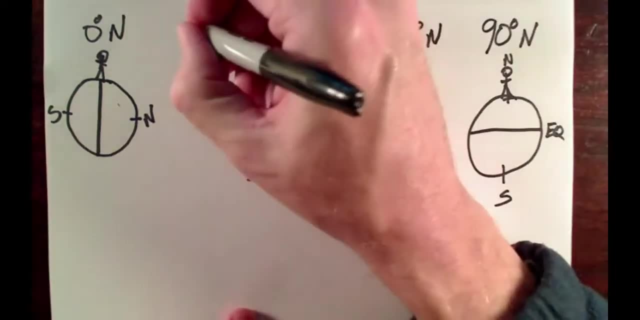 they are to the equator, And so that is what the orientation looks like for someone at 75 degrees north latitude. Finally, let's try one here for, say, somebody at 15 degrees north latitude. What does it look like for someone at 75 degrees north latitude? I'm going to draw the north pole. 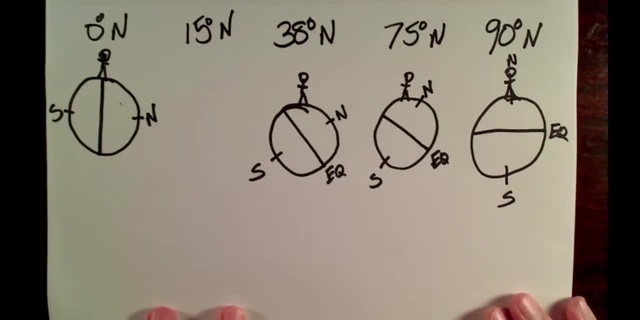 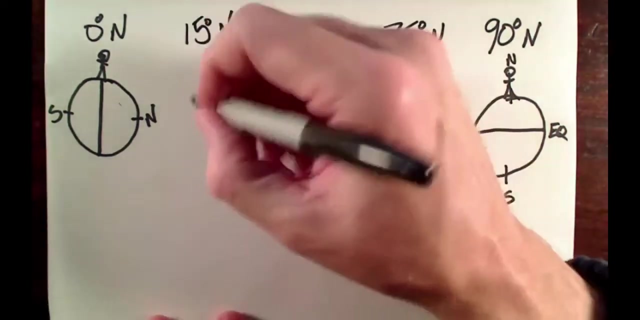 for somebody at 15 degrees north. Go ahead, pause the video. draw your earth for someone at 15 degrees north and I'll be back in a second to show you the answer. All right, so let's take a look at what it is for someone at 15 degrees north. As always, I will draw the earth. I will draw my. 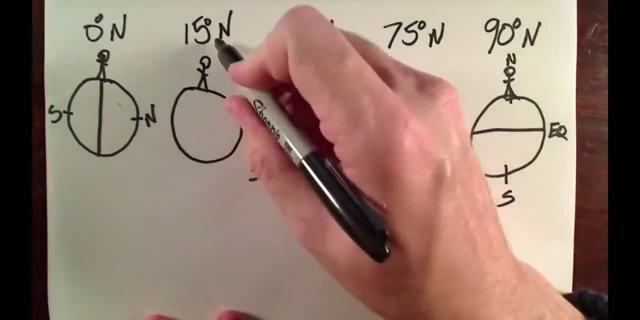 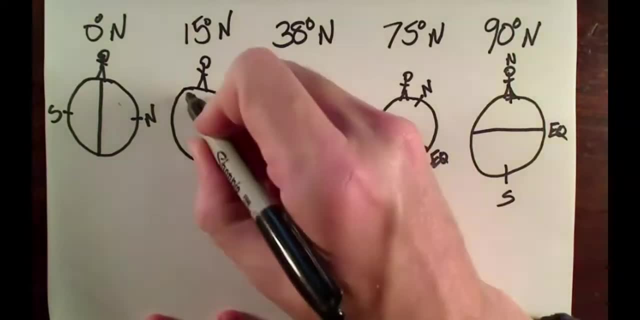 observer standing on top of the earth. Now I know that they are much closer to the equator than the equator is going to be quite far away from them. So let me draw. let's see if I draw the equator like this, so that they are close to the equator but not on the equator, and then I put the north. 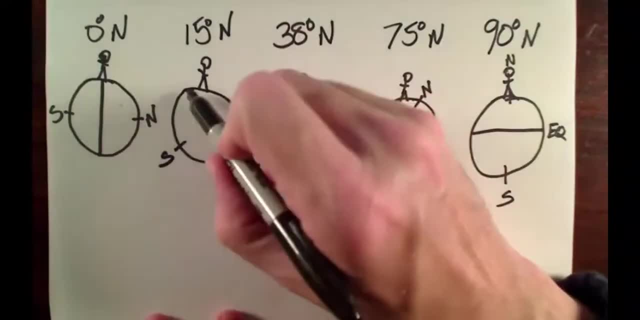 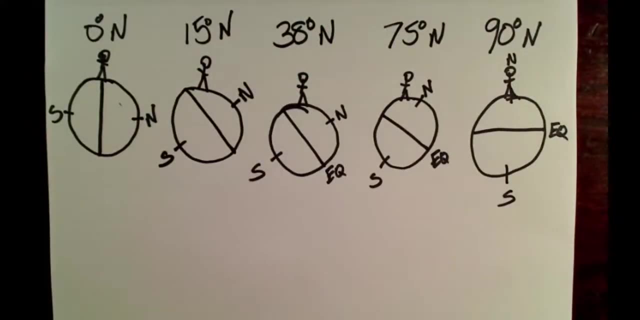 pole over here and the south pole over there. So now when I look at my observer, they're fairly close to the equator. right there They're further away from the north pole and that is what the earth looks like for someone at a latitude of 15 degrees north. So that is celestial sphere. 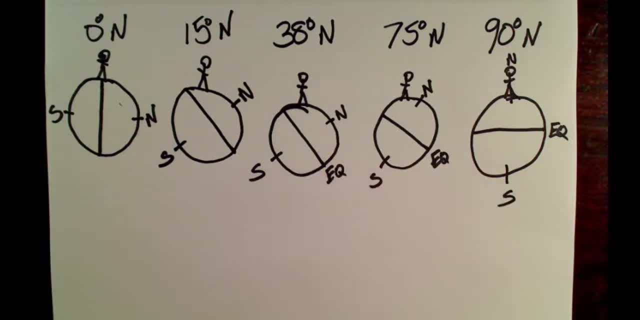 diagrams for different latitudes on the equator. So that's what I'm going to do: I'm going to draw on earth. I didn't do a very good job. between 15 and 38 degrees, They kind of look similar to one. 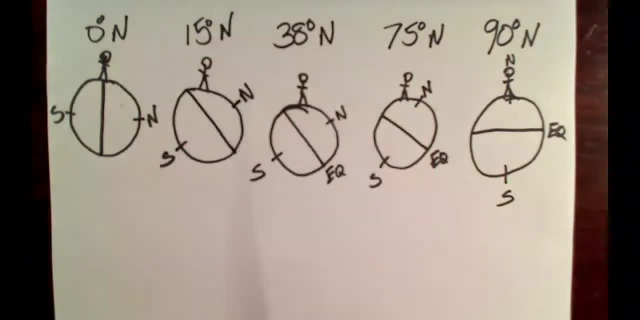 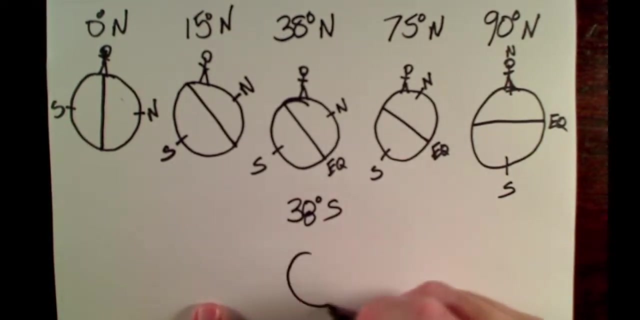 another. This one should have probably been tilted a little bit more over. Let's draw one now for 38 degrees south. What does it look like for someone at 38 degrees south latitude? Well, at 38 degrees south, I will do exactly what I did before. I will draw the earth, I will put my observer standing on. 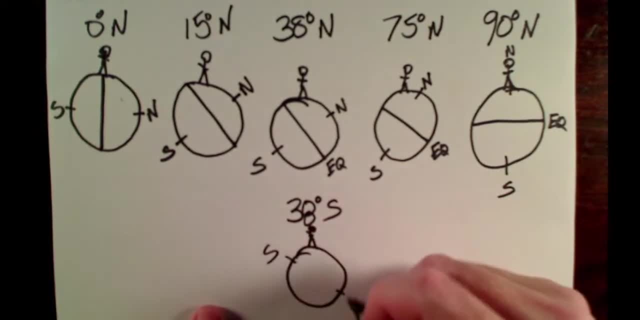 the equator. In this case I'm going to draw the south pole, the north pole and the earth's equator, like that You can tell that they're 38 degrees south, because they are between the equator and the south pole on the earth right. They are south of the equator, so they are at 38 degrees south. 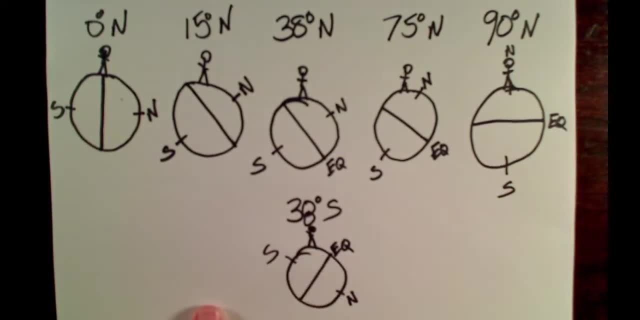 and 38 degrees is about halfway between the south pole and the equator, like that. So that's a pretty good diagram for 38 degrees south. You can imagine what a diagram would look like for somebody at 90 degrees south. Go ahead and pause the video and take a moment to draw that diagram. What would it? 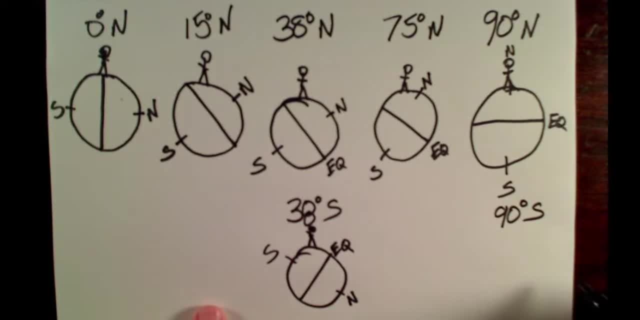 look like for somebody at 90 degrees south. Okay, at 90 degrees south, we're going to draw the earth, We're going to draw the observer standing on top of the earth. Now we need to orient the poles in the equator underneath them. Well, at 90 degrees south, they are standing on the south pole, so that 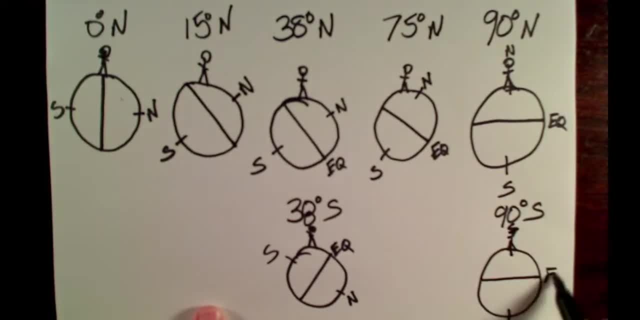 is south. This is the equator. We're going to draw the observer standing on top of the earth. This is the north pole and that is the earth's equator, cutting across like that For somebody at 15 degrees south. so let's do one last one here, at 15 degrees south. 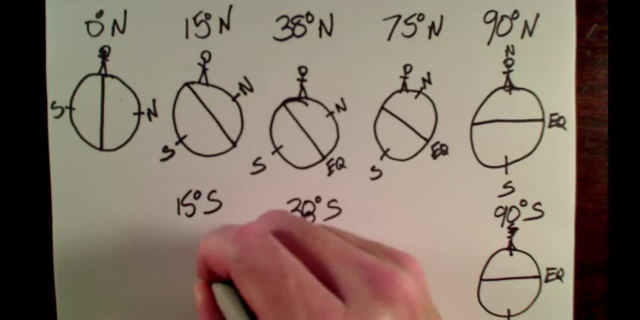 For someone standing at 15 degrees south. I will draw the earth. I will draw my observer standing straight up and down. You will remember that they are closer to the equator than they are to the pole, so I will put the equator fairly close to their feet. 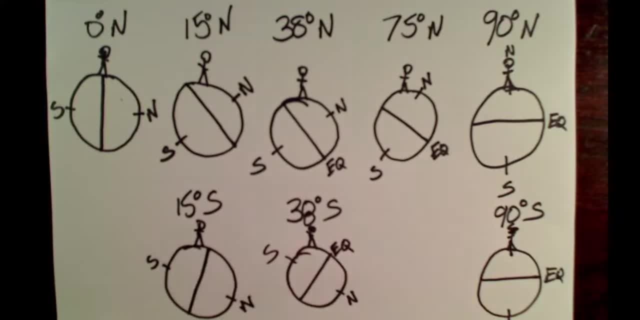 which means that this is the south pole and that is the equator. The equator is the north pole, right there, and you'll see that they're fairly close to the equator, but they are south of the equator, That is, if we start on the equator and head towards the south. 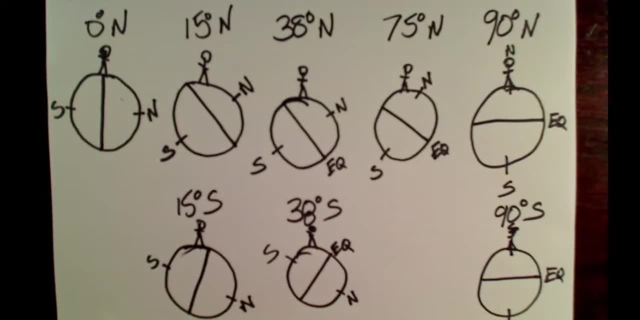 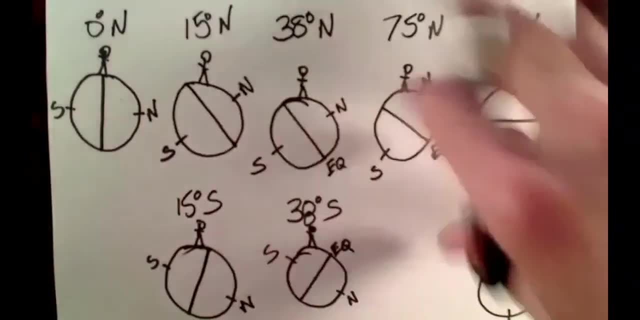 pole. they are south of the equator, so they are at about 15 degrees south latitude. So that's what it looks like for an observer at 15 degrees south. So this has given us some practice orienting the earth underneath our observer for different latitudes on earth. If you need to go back, 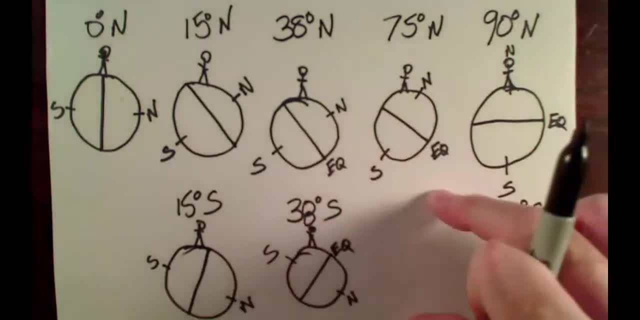 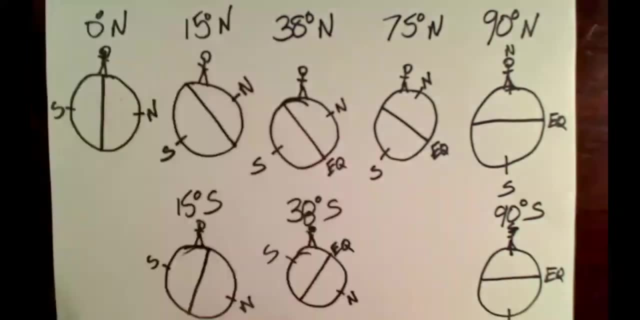 now would be a good time to pause and practice. with these. You could fill in 75 degrees south and imagine what it's also like for somebody on the equator. You can imagine that this one should look exactly like that one. It doesn't matter if you switch the north and the south, because, again, 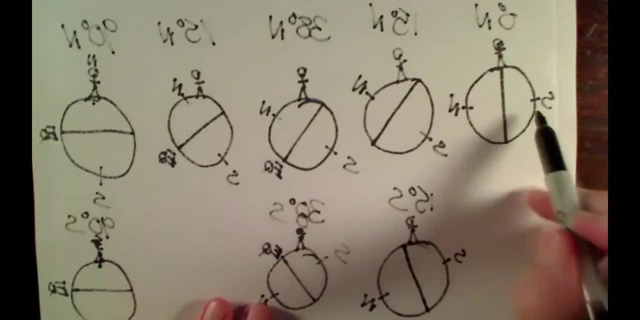 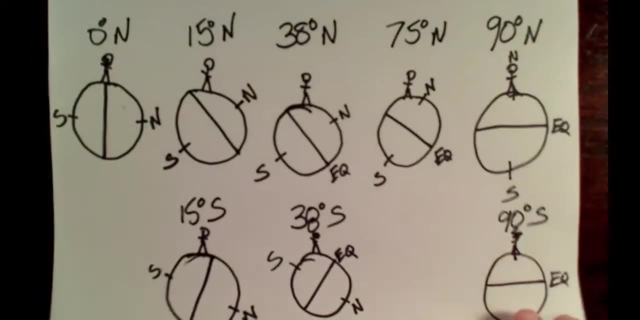 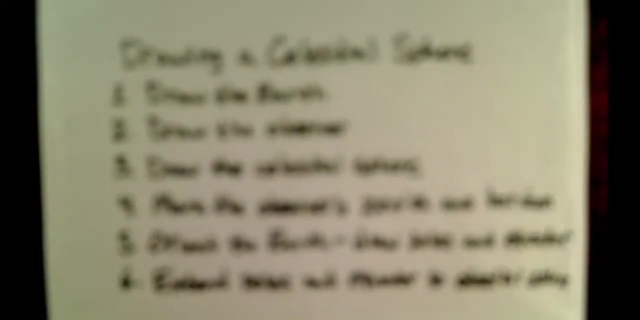 if you switch them like this, it's the same celestial sphere. it's just seen from the other side, and that's a perfectly valid way to draw the celestial sphere. So now let's talk about the steps that it takes to draw a celestial sphere. These are the steps for drawing a celestial sphere. 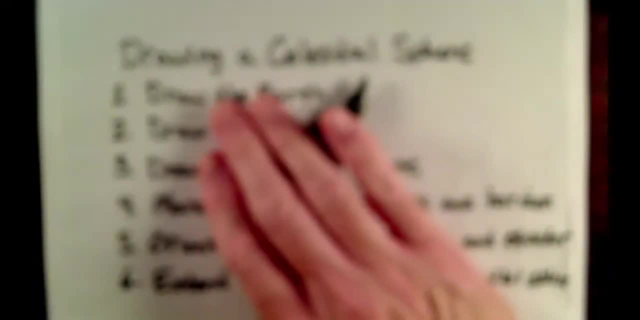 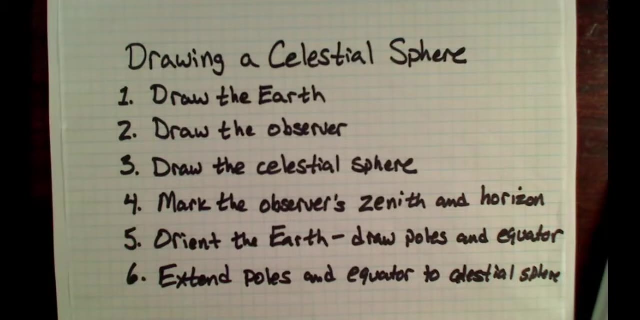 Get the camera to focus here. There we go. So for drawing a celestial sphere, the first thing you need to do is draw the earth. The second thing you need to do is draw the observer standing straight up and down. Then we're going to draw the celestial sphere around the earth and the 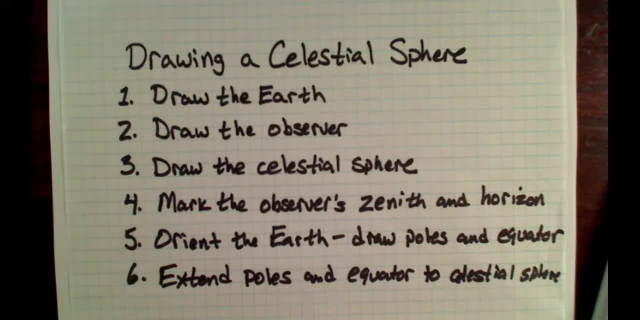 observer. We're going to mark the observer's zenith and their horizon and then we will orient the earth underneath the observer. We'll draw the north pole, the south pole and the south pole And the equator, And then we will extend those poles and the equator out onto the celestial. 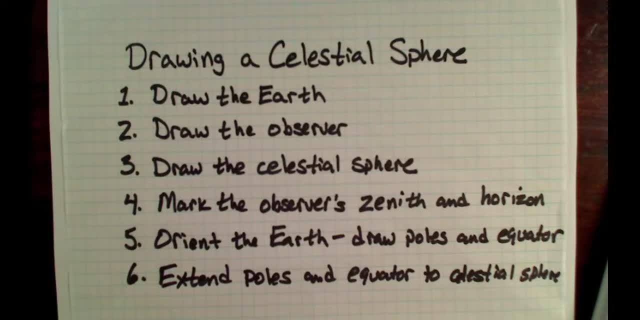 sphere. Basically, we're going to do exactly what we did in those diagrams a second ago. Every time I draw a celestial sphere, I will always follow these six steps in exactly this order. So I will always draw the earth and then the observer and the celestial sphere. I will mark 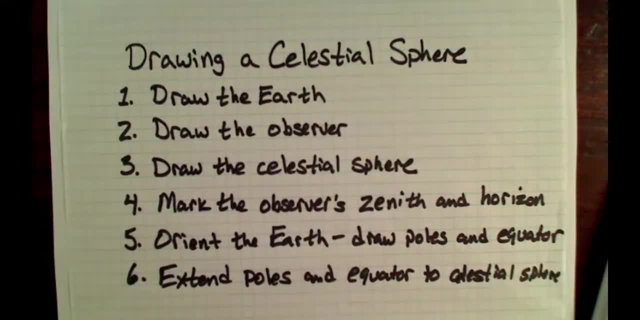 their zenith and horizon. I will draw the poles in the equator and then I will extend the poles in the equator, And then I will draw the poles in the equator, And then I will extend the poles in the equator, And then I will extend the poles in the equator, And then I will extend the poles in the. 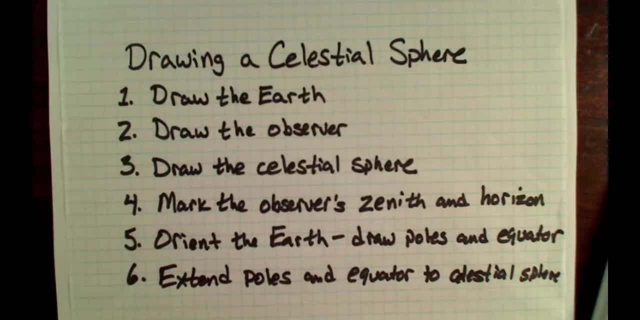 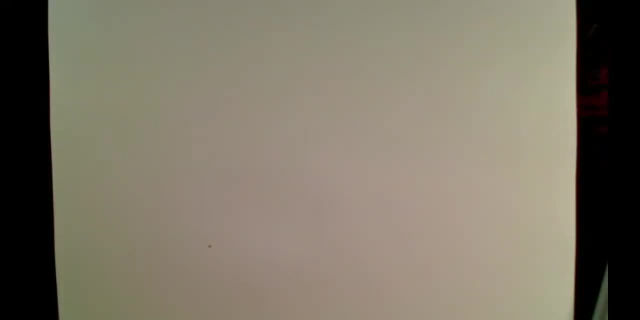 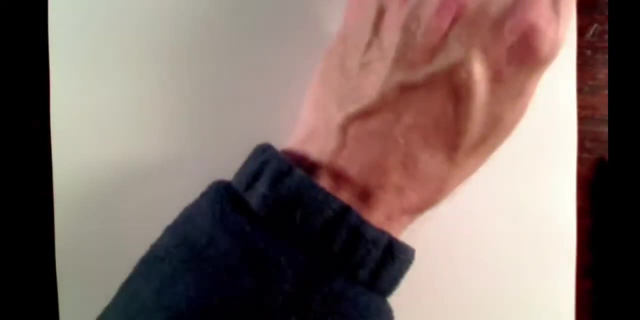 equator to the celestial sphere. I think you should get in the habit of always drawing your celestial spheres in the same way. So let's practice a celestial sphere here, And let's practice a celestial sphere for an observer at 38 degrees north latitude. So let me slip that in. 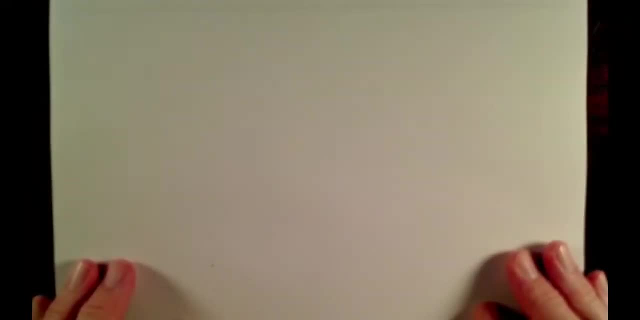 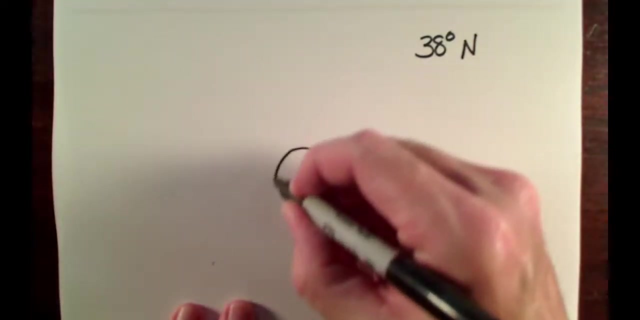 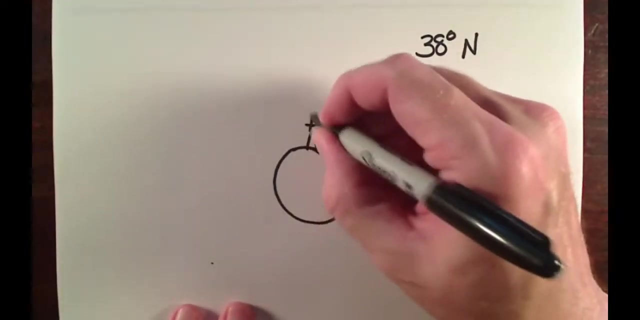 there, All right. So let's draw a celestial sphere for an observer at 38 degrees north latitude. So this is the latitude that we have right here in Charlottesville, Virginia. So first step, draw the earth. Second step: draw my observer standing straight up and down on top of the earth. So there's my 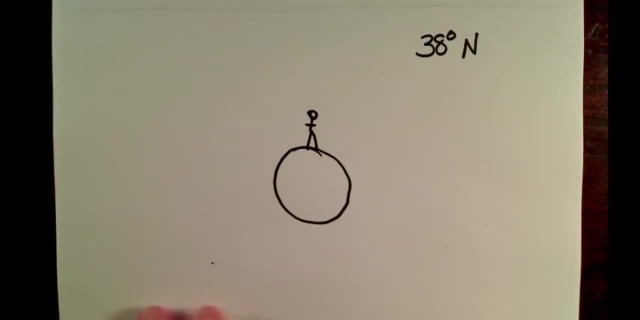 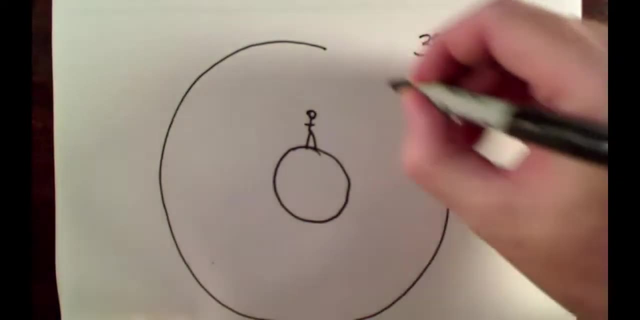 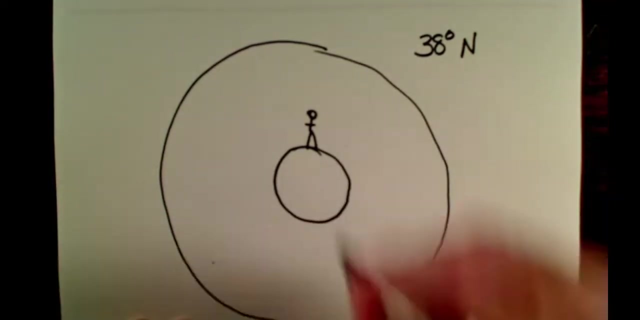 observer straight up and down on top of the earth. The next thing is draw the celestial sphere. So I'm just going to draw this big circle around the earth. that is the celestial sphere. Okay, so there's the celestial sphere. The next thing I need to do is mark the observer's zenith and horizon. The zenith is the point. 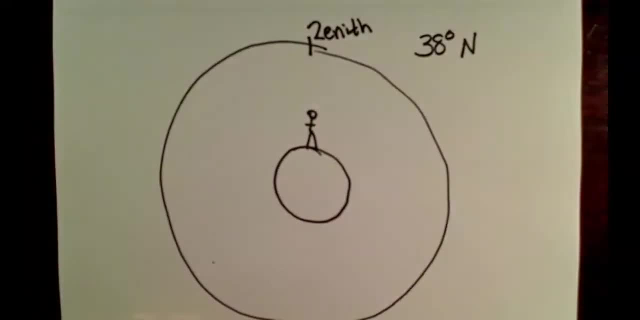 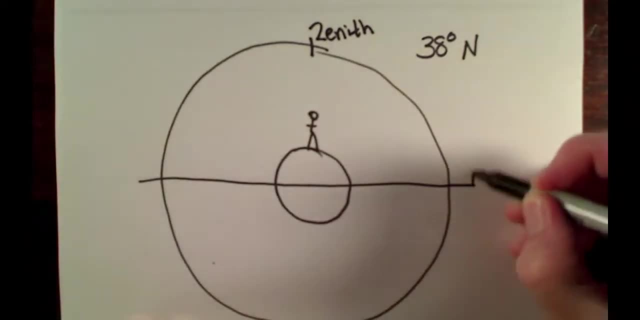 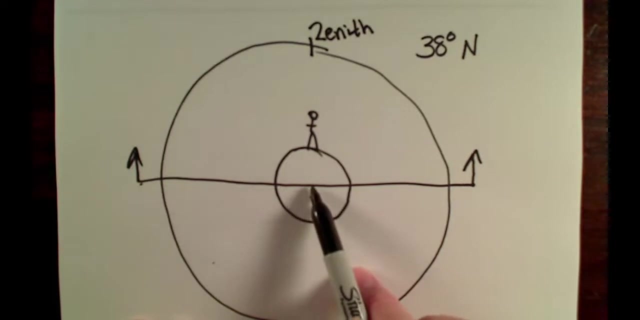 straight over their head. So there is the zenith up there And their horizon. I'm going to draw like this And they can see everything above the horizon and they can see nothing below the horizon. And this time I drew the horizon going through the center of the earth, And I will talk in a 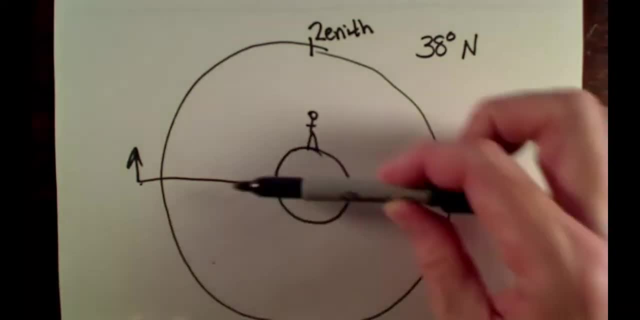 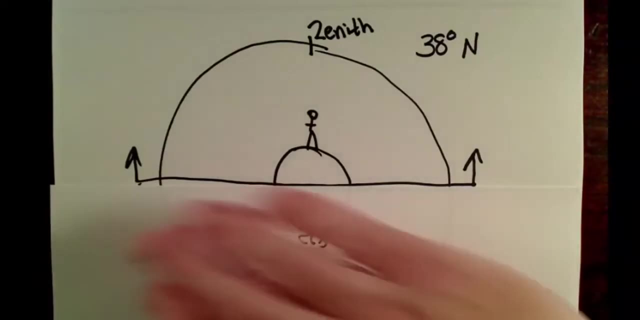 I've drawn the horizon through the center of the earth. They can see everything above the horizon. They can see nothing below the horizon. That is, everything down here is hidden from view. So that is how we view the sky. We can't see anything below the horizon. Now we're going to 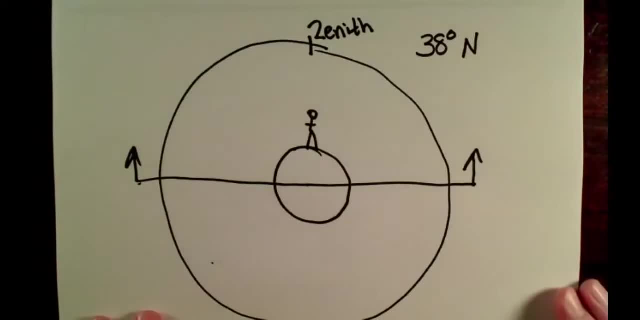 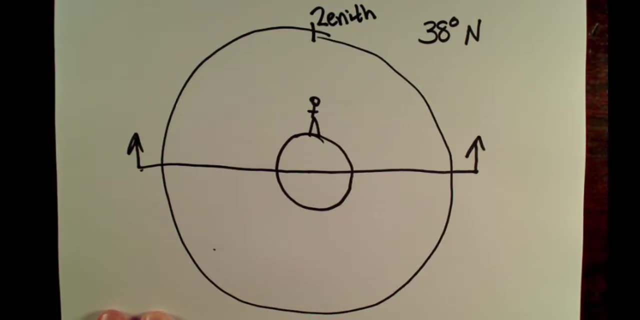 continue the diagram and show the whole celestial sphere here, but just know that you can't see anything below the horizon. All right, step number five: orient the earth underneath the observer. Draw the poles in the equator- This is for someone at 38 degrees north. At 38 degrees north, they're. 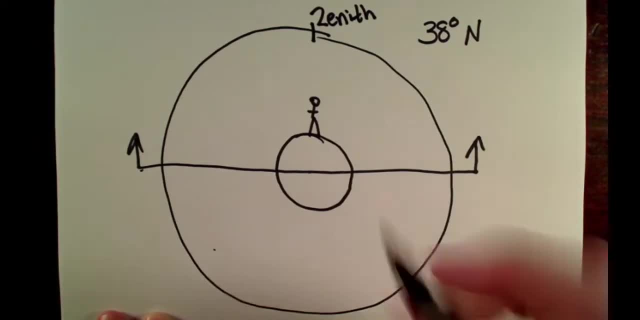 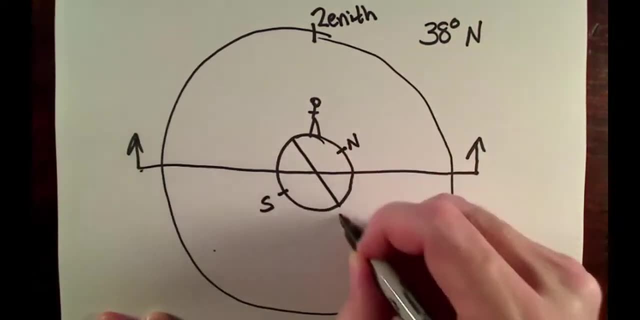 about halfway between the pole and the equator, a little bit closer to the equator. So I'm going to head and draw the north pole here, the south pole here, and draw the equator at a right angle to those and there is the earth's equator. So here's the equator, I head north from the equator. 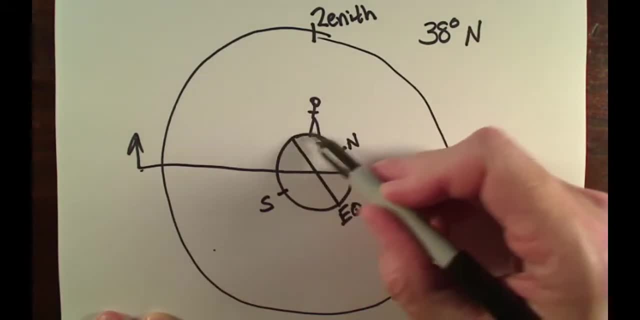 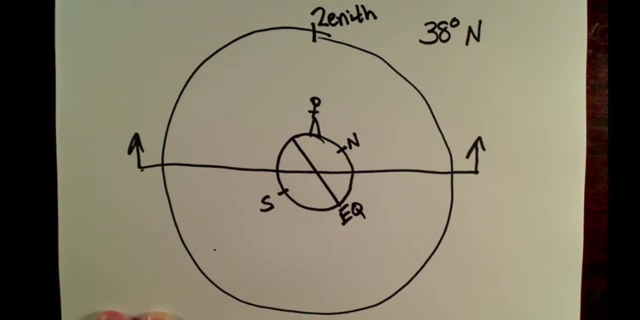 I get to my observer. They're a little bit less than halfway between the equator and the north pole, so that's pretty good there for 38 degrees North latitude. So that's the earth oriented underneath. Now I need to extend the north pole. 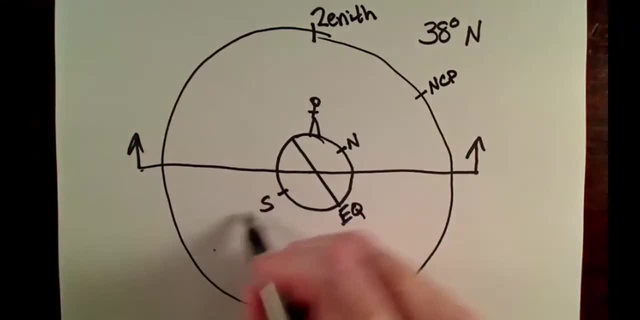 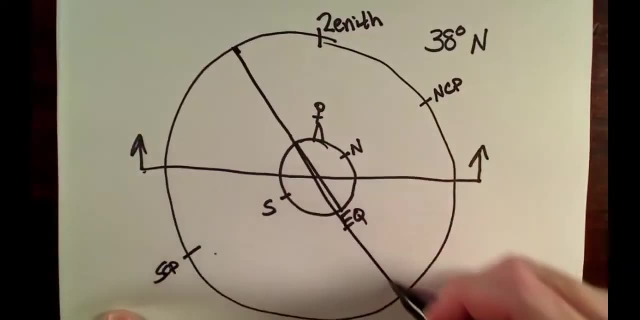 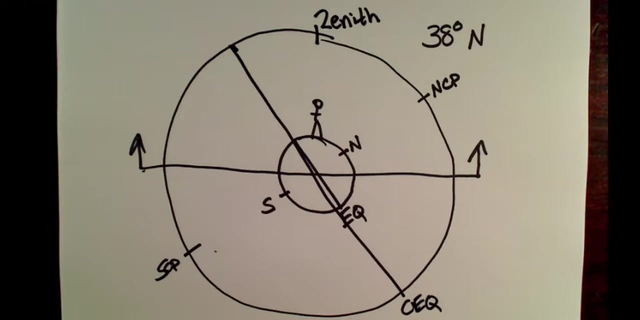 out into space to get the north celestial pole, extend the south pole into space to get the south celestial pole and extend the earth's equator into space to get the celestial equator. And this is how the sky appears to an observer at 38 degrees north latitude. You'll notice that the 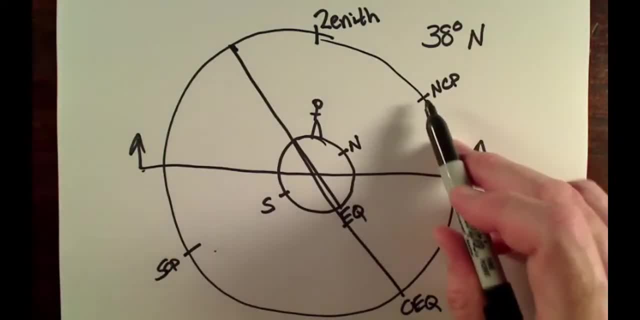 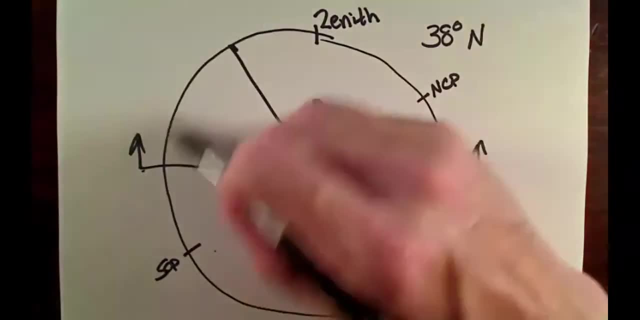 north celestial pole is about halfway between the equator and the north celestial pole. In fact, as we'll see, it's a little bit less than halfway up in the sky. The zenith is straight over their head. The earth's equator gets quite high in the sky, but the earth's equator doesn't. 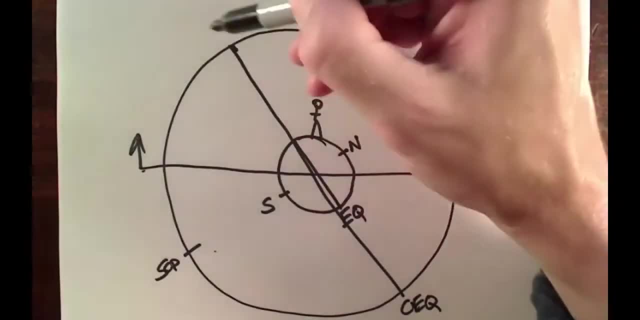 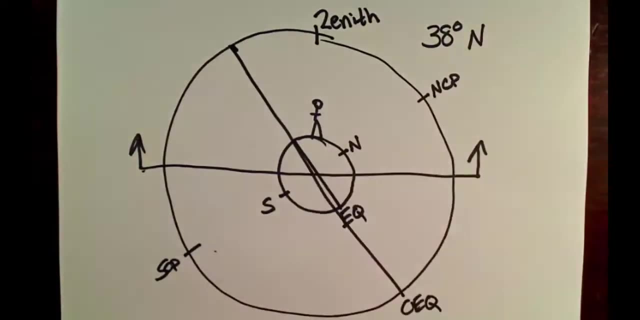 get straight overhead: It rises over here in the east, moves across the sky and sets over there in the west. So that is the two-dimensional celestial sphere for an observer at 38 degrees north. That's how you draw your celestial sphere. 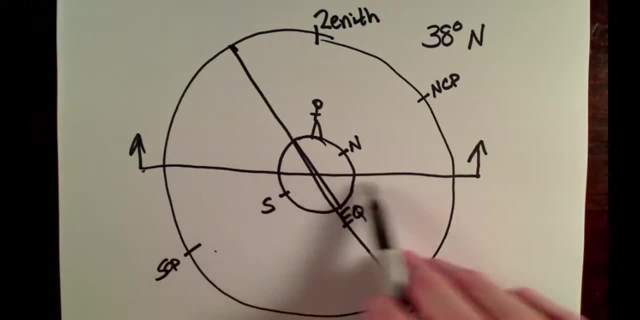 Now I want to spend a moment here to talk about the celestial sphere. I want to talk about the celestial sphere. I'm talking about why it was that I drew the horizon through the center of my celestial sphere and I didn't draw it through the feet of my observer, like I did earlier in the very 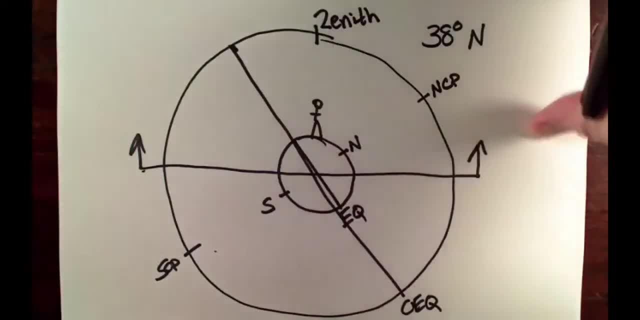 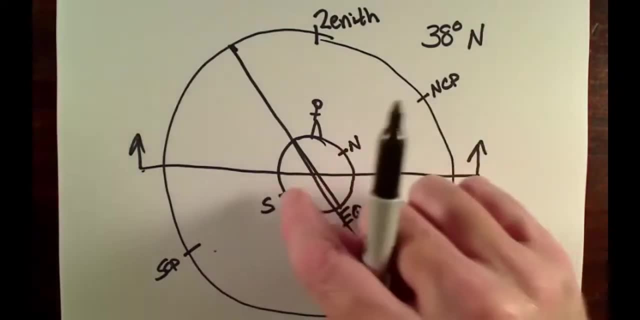 first diagram that we drew. Why did I draw it this way? The answer has to do with the fact that I drew the earth too big here Now. I drew the earth too big for a reason: I wanted you to see the north and the south pole, and I wanted you to see the equator. In truth, the earth is an infinitesimally. 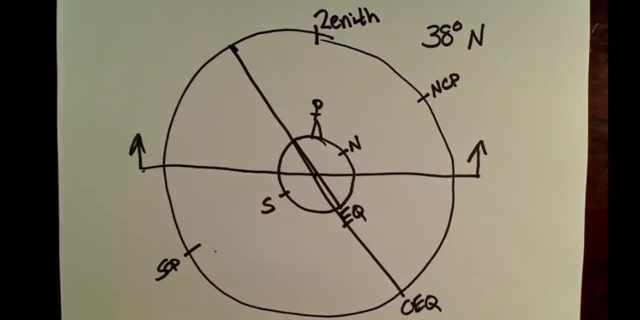 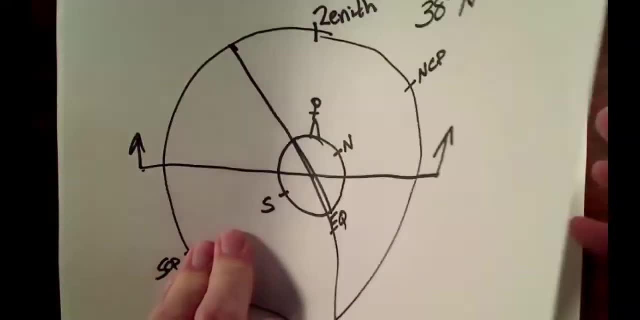 small point right there, And because the earth is an infinitesimally small point, we couldn't see the north and the south poles and the equators. Let me draw a proper celestial sphere with the earth to its proper size and you'll understand why I draw the horizon. 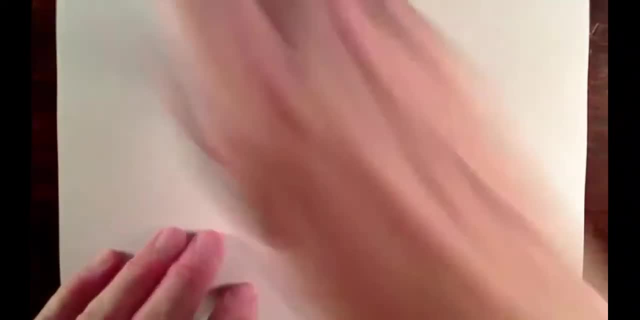 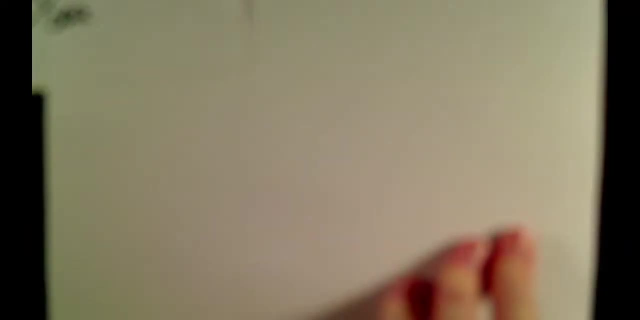 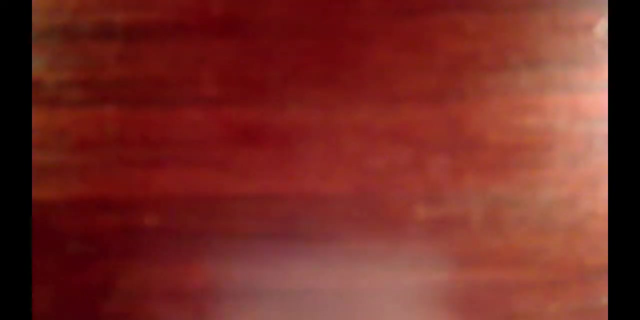 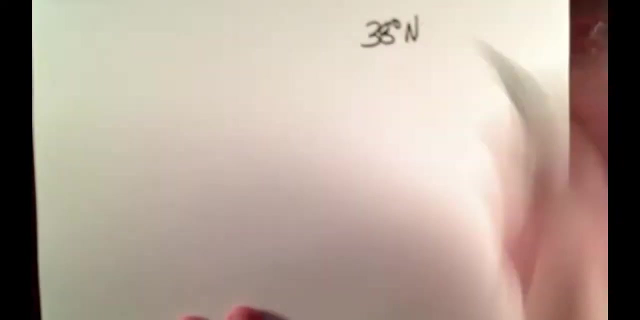 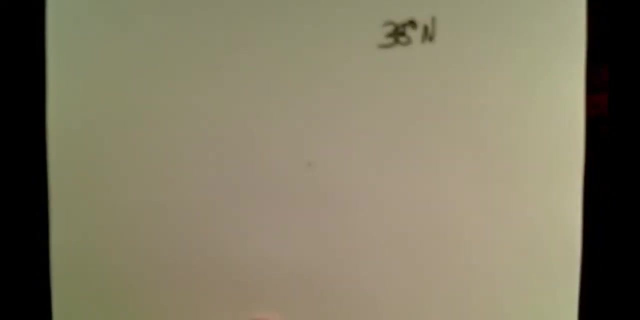 through the center of the celestial sphere. Okay, so let's imagine that I'm going to draw my celestial sphere for someone at 38 degrees north latitude, But now I want to draw it to a more proper scale. So here's the issue. That's the earth, right? So the first thing I do is I draw the earth. 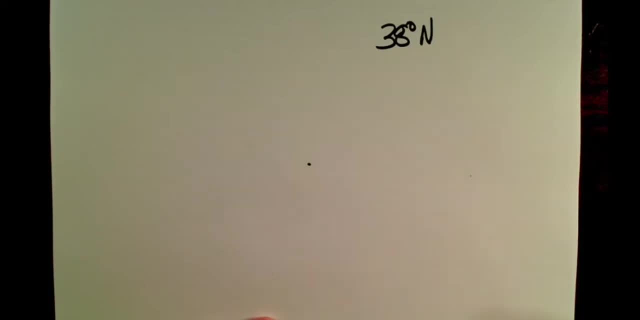 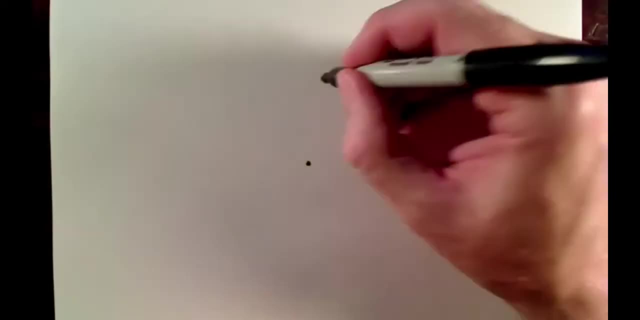 The earth is infinitesimally small compared to the celestial sphere. Now I draw my observer standing on top of the earth. So there's the observer standing on top of the earth. Okay, now I draw the celestial sphere around it. So there's the celestial sphere. 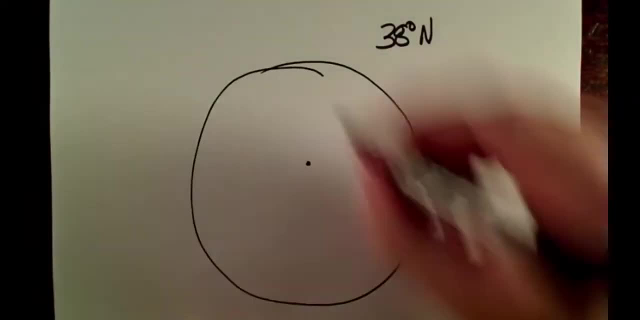 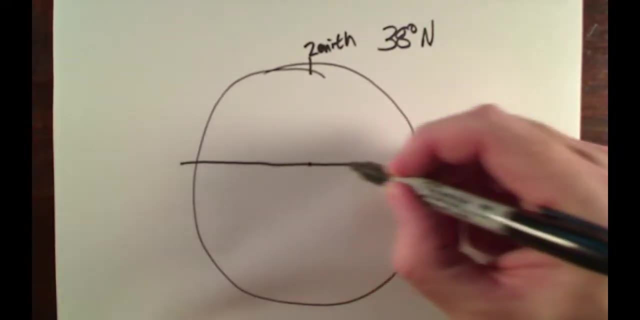 surrounding the earth. And now I need to mark the observer's zenith. So there's their zenith Going through their feet. I have the horizon right here that runs through their feet, so they can see everything above the horizon. That's what those two arrows represent. They can see. 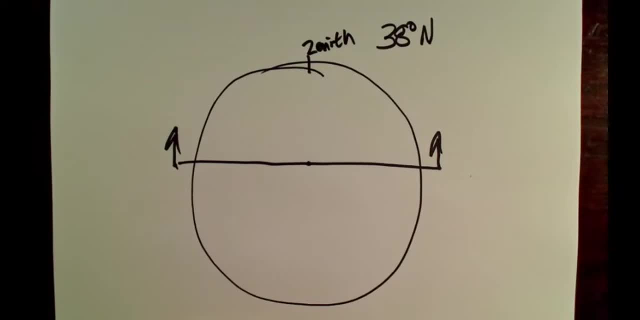 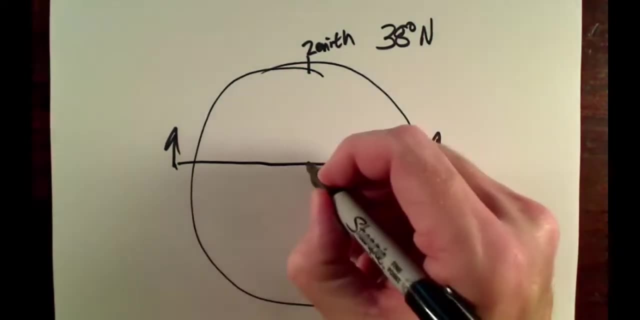 everything above the horizon, but they can't see anything below the horizon. Okay, so I've marked their zenith and horizon. Now I need to orient the earth underneath the observer. So I draw in the north pole, I draw in the south pole, the equator right there, And then I extend the 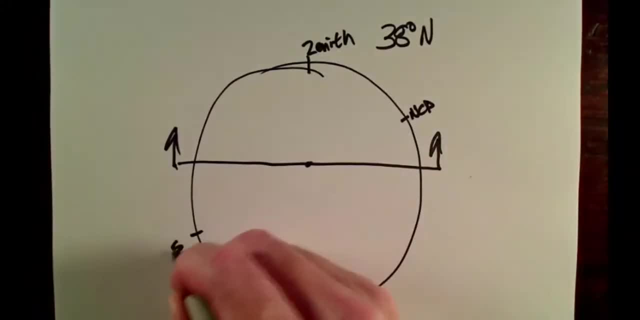 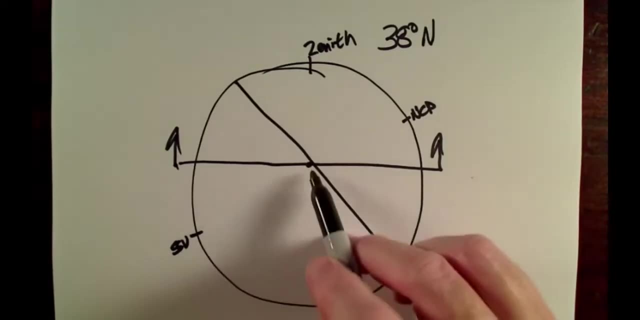 north pole out to get the north celestial pole, the south celestial pole and the celestial equator. So you'll notice in this diagram here that because the earth is infinitesimally small at the center, you couldn't make out any of the essential details such as the north pole. 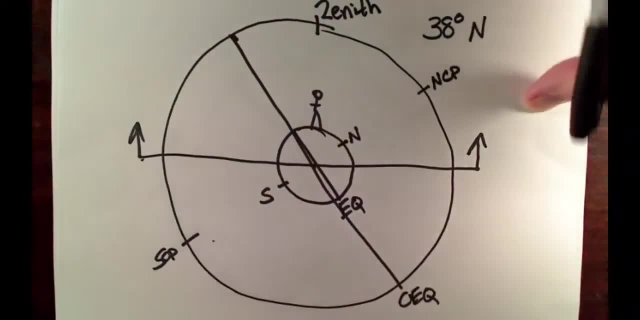 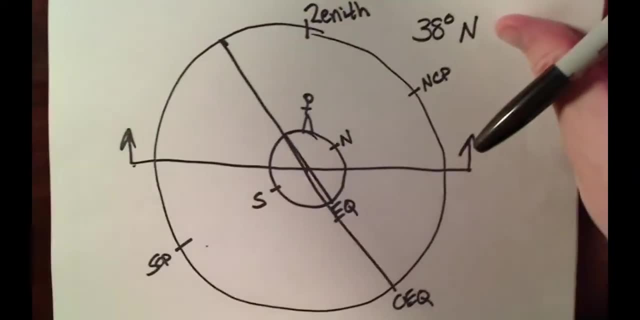 the south pole and the earth's equator, because it's just too small. So, rather than so, the solution to that is to make out the north pole, the south pole and the equator. So I'm going to draw the earth a little bit too big, And when we draw the earth too big now, we can see the north. 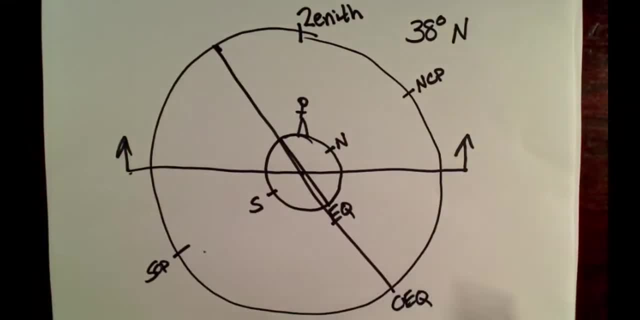 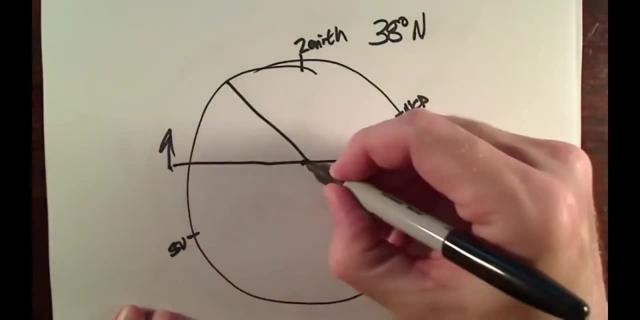 pole and the south pole and the equator. But when we draw the observer's horizon, we want to be careful to draw it through the center of the earth, because in truth, like this diagram, the earth is an infinitesimally small point down there at the center, And so the horizon really does cut the 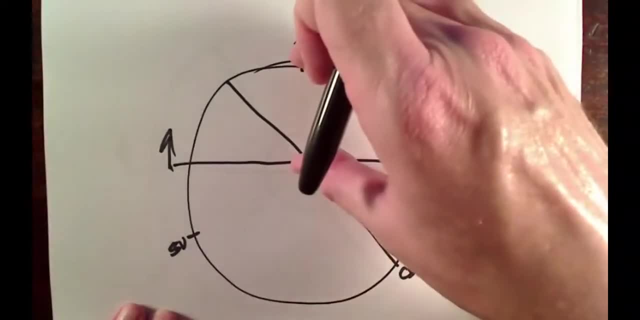 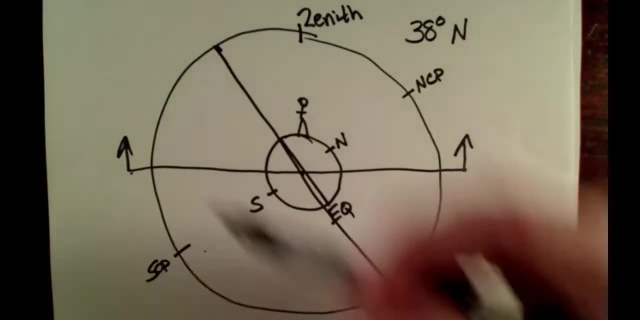 celestial sphere into two equal halves. When you're standing on the earth, you can see exactly half the sky above you, and exactly half the sky is hidden below you In this diagram, though if I were to draw my horizon up here through the feet of the observer, 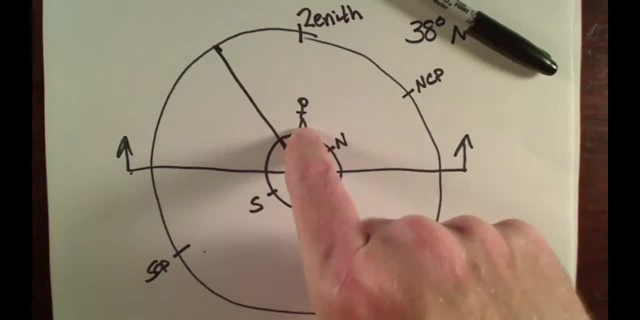 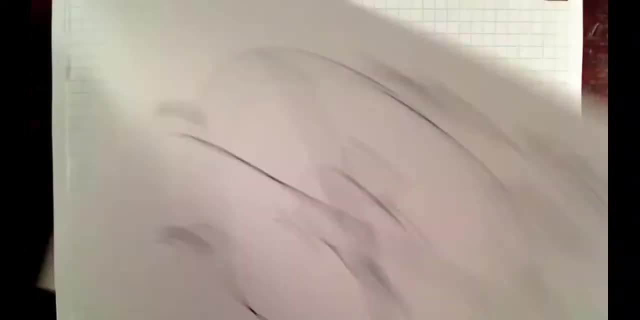 it looks like they can see less than half of the sky, and more than half of the sky is below their horizon, And that's not the way it works. So that's simply why I drew the horizon through the center of the earth, right there. So let's draw a couple more celestial spheres to get some. 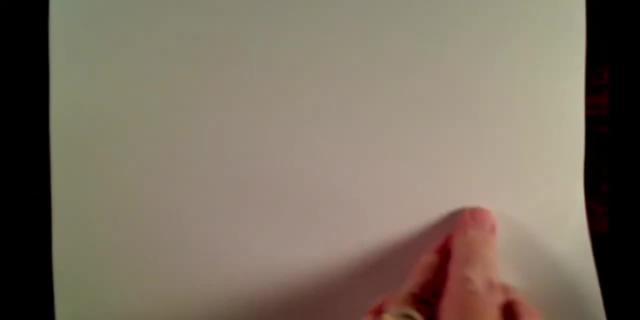 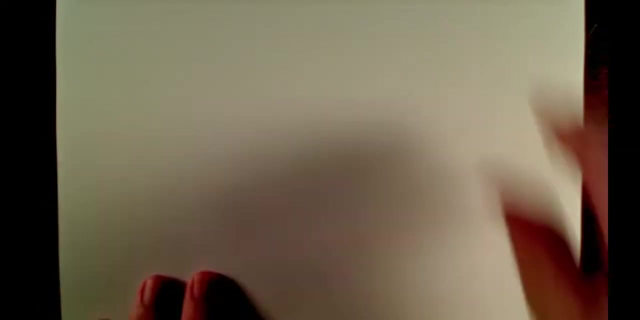 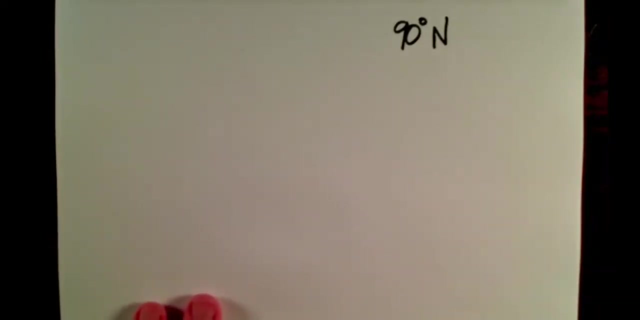 practice here. So let's draw a celestial sphere for Santa Claus living up there on the north pole. So Santa Claus lives at 90 degrees north latitude. So let's draw a celestial sphere for Santa Claus at 90 degrees north latitude. So 90 degrees north. We begin by drawing the earth. 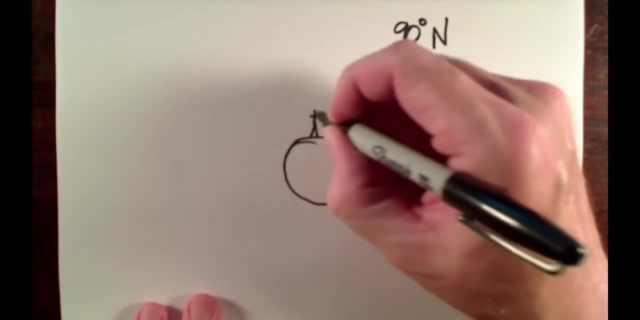 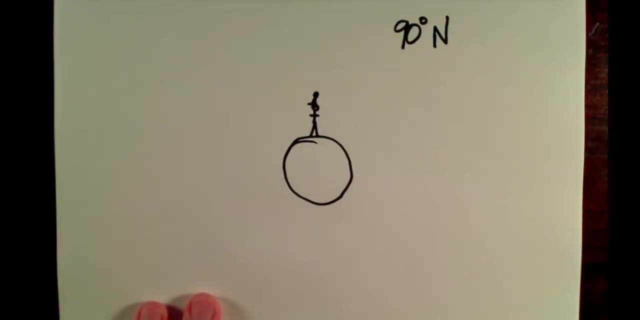 Then we draw our observer standing straight up and down on the earth. So there's Santa Claus. I'll give Santa a Santa hat, because that's Santa Claus. So there's our observer standing straight up and down on top of the earth. Next step: draw the celestial sphere. 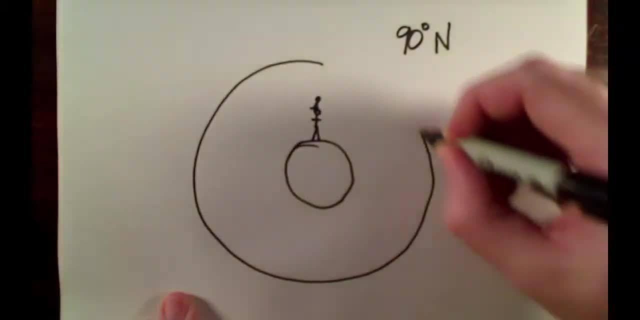 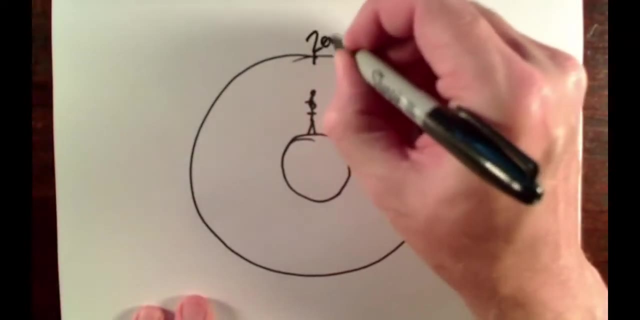 So Santa's standingylong over the earth. but when we draw the earth we can draw our observer standing. So there's the celestial sphere surrounding the earth. Next I need to mark the observer's Zenith. So that is their Zenith And I need to draw in their horizon. 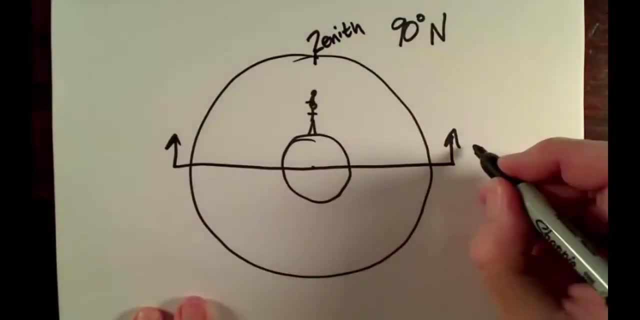 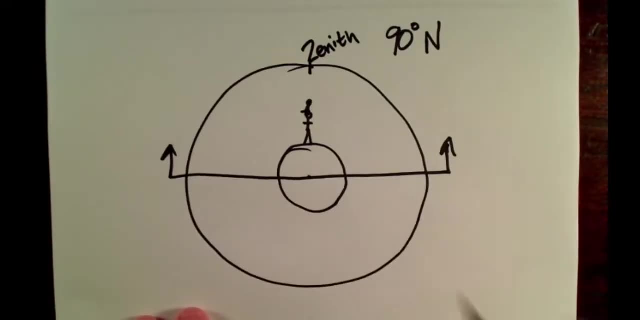 So there is their horizon. They can see everything above the line, but they can't see anything below the line. Next, I need to orient the earth underneath the observer, and this one's fairly easy, because we're standing at 90 degrees north. We're standing at 90 degrees west. 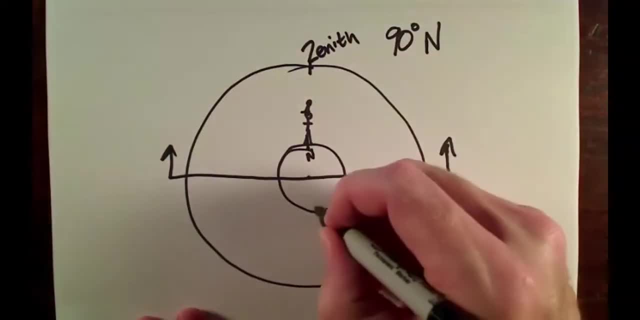 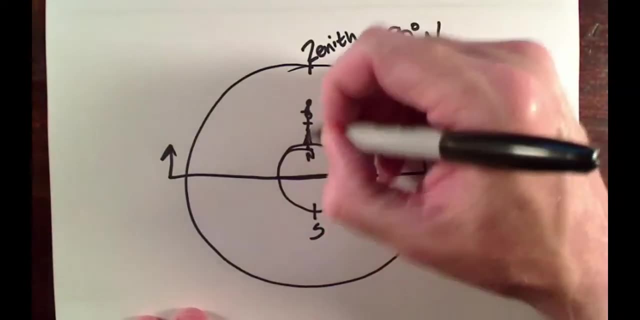 north. we're standing on the north pole. so this is the north pole of the earth, that is the south pole of the earth. this is the earth's equator, right there and now. if i extend the pole out, i get the north celestial pole up here, i get the south celestial pole down here, and then this: 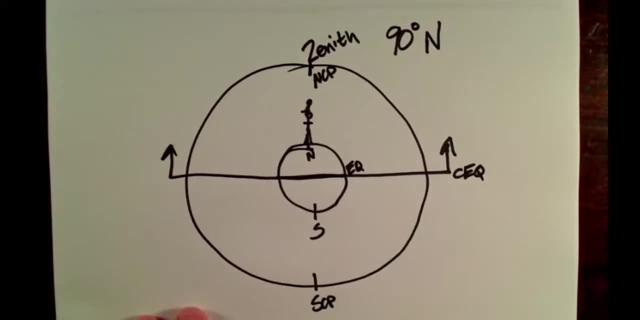 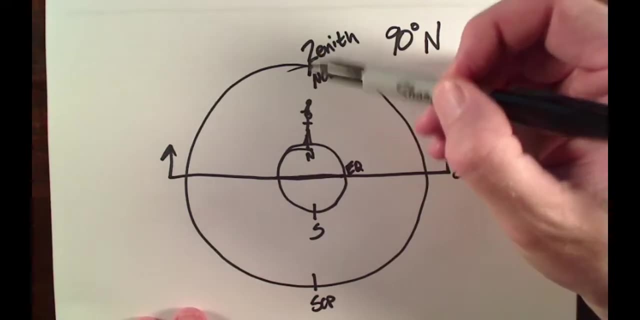 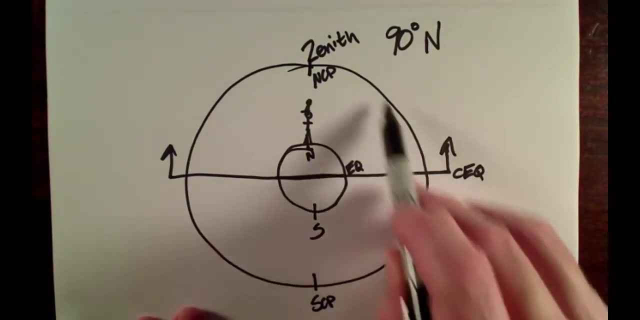 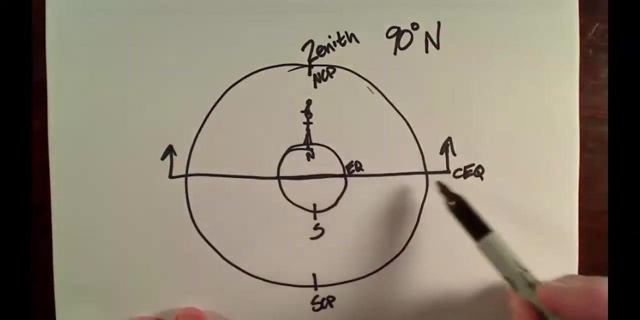 becomes the celestial equator. a couple really interesting things about this diagram. you'll notice that because i'm standing on the north pole, the north celestial pole is straight overhead, it's at my zenith, and you might remember that the altitude: it measures how high something is, starting from the horizon and measuring up. so in this case, the north celestial pole, the north pole. 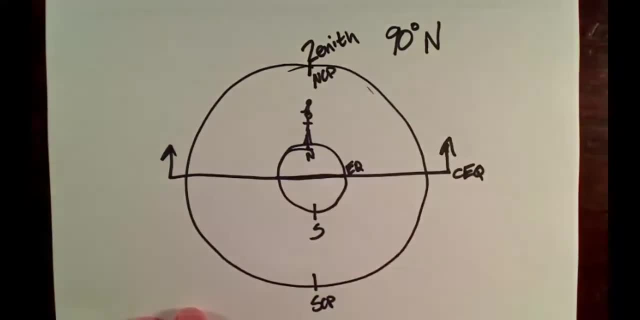 in the sky, because it's at my zenith- is 90 degrees up. the altitude of the north celestial pole is 90 degrees and that's an important thing to remember. i'm going to start a table right here for some of our results and, in this table, what we're going to do. 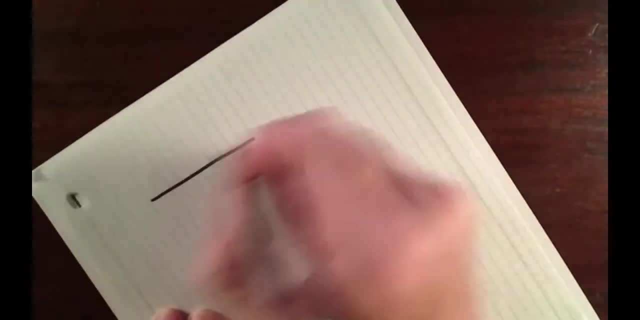 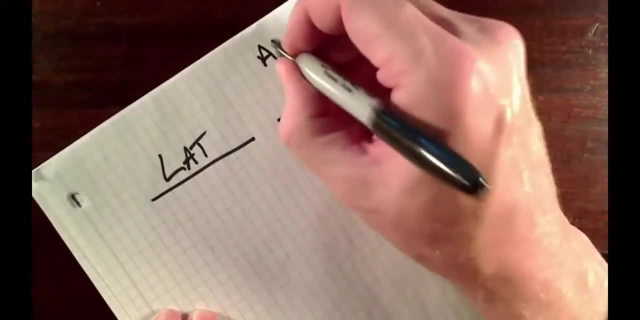 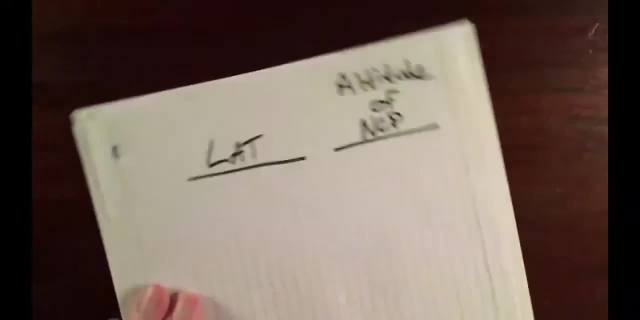 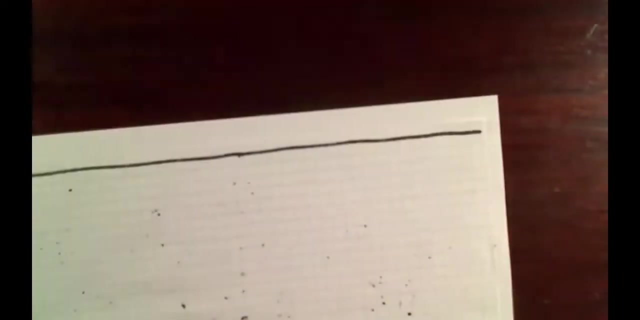 and we're going to record the altitude of the north celestial pole, that is how high up it is in the sky. so our latitude and the altitude of the north celestial pole. so what is it in this case? well, let's go back for santa claus standing at the north pole. our latitude is 90 degrees. 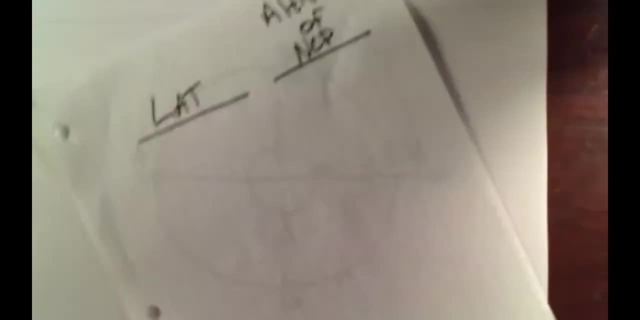 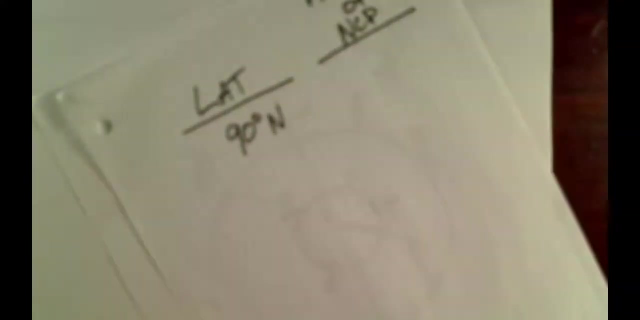 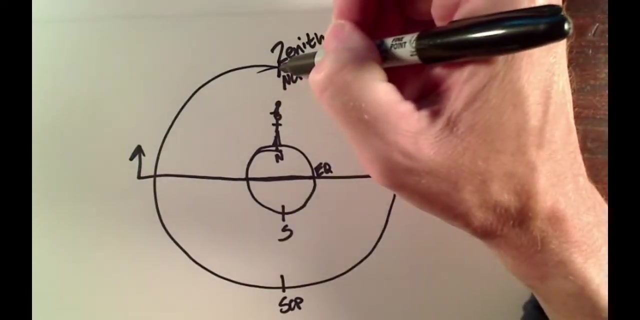 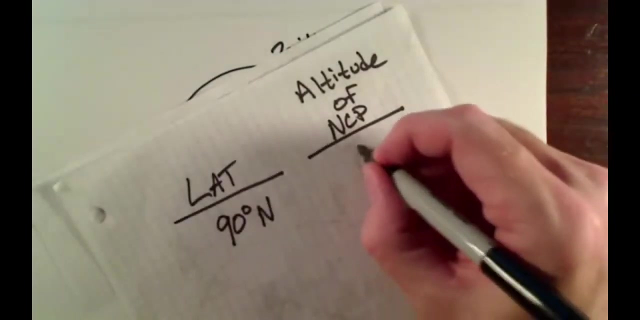 north, so our latitude is 90 degrees north. the altitude of the north celestial pole: if i start on the equator and measure up to the north pole, i get all the way up to the zenith up there. that is a right angle, a 90 degree angle, and so the altitude of the north celestial pole happens to be 90. 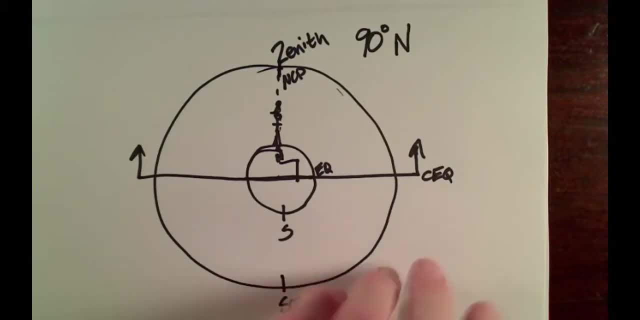 degrees. let's draw another celestial circle and we're going to start a table and we're going to, and this time let's draw it for someone standing on the equator of the earth and see. oh, one more thing i wanted to mention before we do that. one sorry mention about this one is not only is the 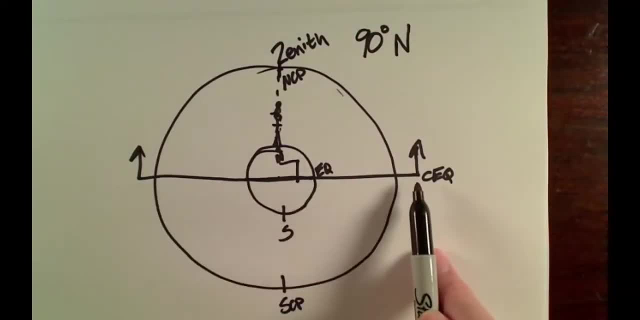 north pole at your zenith, but you will notice that the earth's equator corresponds to your horizon, that is, if you're standing on the north pole. the north celestial pole is straight over your head and the celestial horizon, the celestial equator, matches your horizon. it lies all the way on the 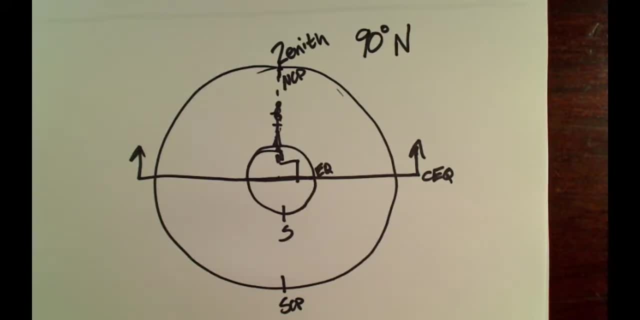 horizon around you. later on we're going to see something really cool that, if you think about what happens as the earth turns, remember the stars are going to move on the celestial sphere as the earth turns and they're going to move round and round like this. so the 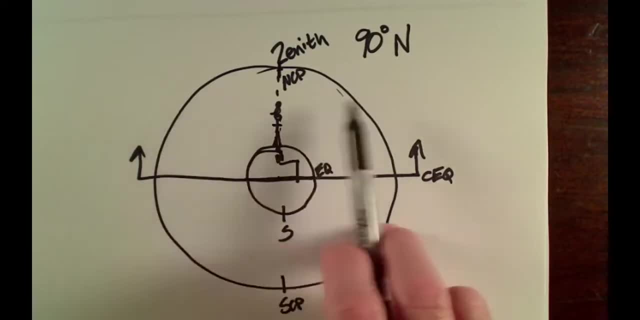 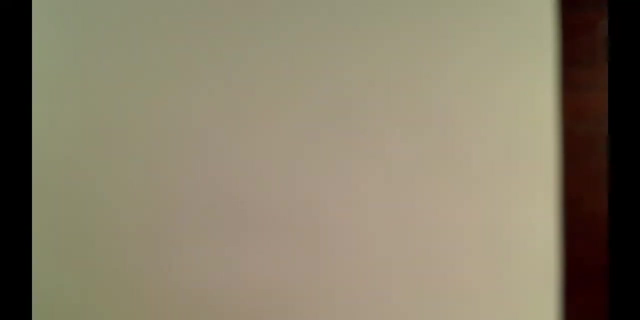 stars up there at the north pole are moving round and round like this. they never rise or set, they just go round and round and round the sky up there. but we'll talk more about that later, in a future lecture, when we talk about as the world turns. for right now i want to draw another celestial. 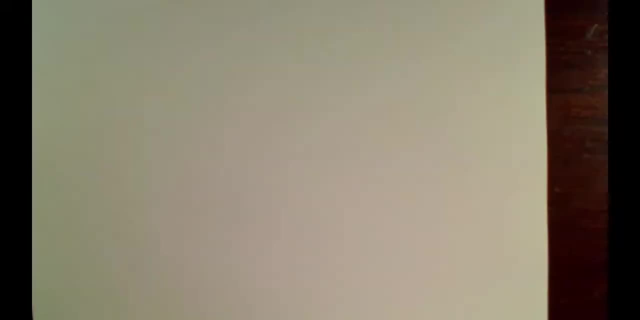 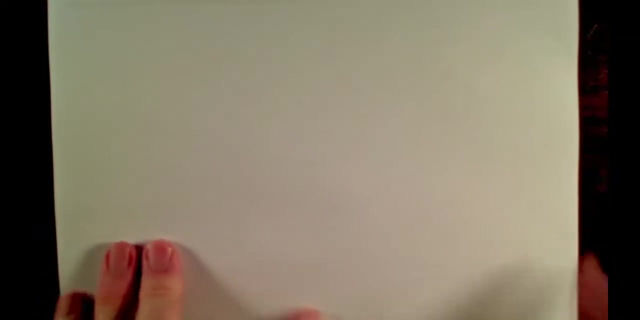 sphere, and this one for itself. you can just move in 18 degrees b, it's down to about 18 degrees. there are times when you 있지 the celestial at zero degrees north, somebody on the equator. So let's draw our celestial sphere for somebody at zero degrees north latitude. I don't really have to. 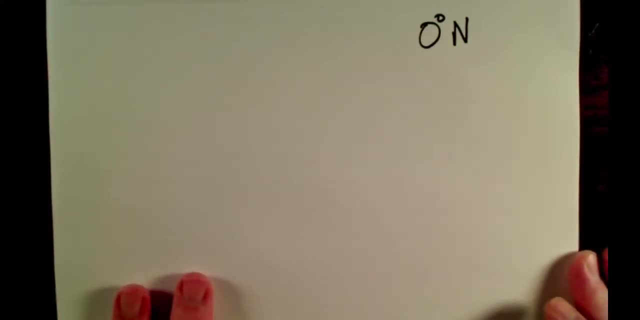 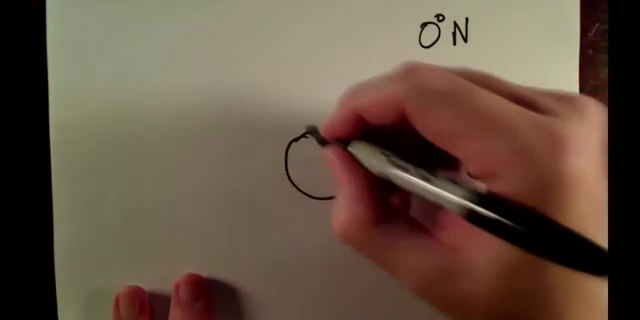 say north, they're on the equator, so zero north is the same as zero south, But let's go ahead and draw it anyhow. Step number one: draw the earth. Step number two: draw my observer standing straight up and down. Step number three: draw the. 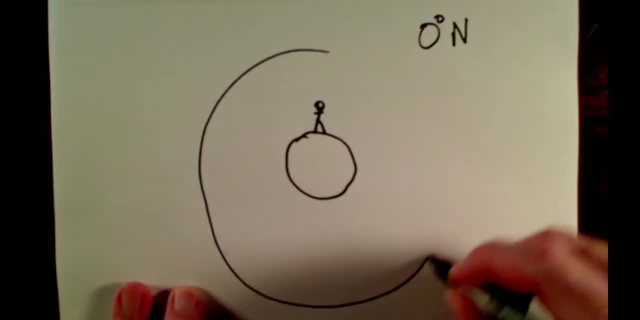 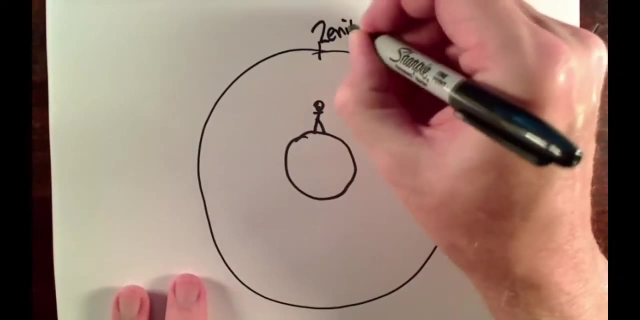 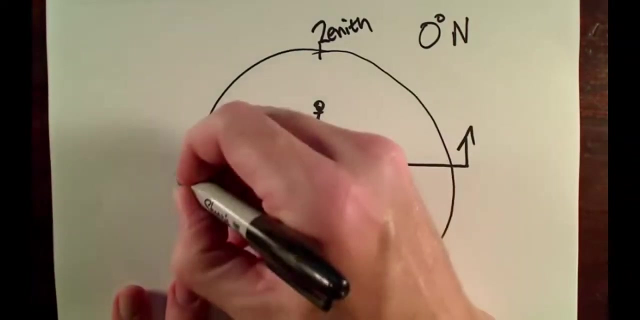 celestial sphere. So I'm just gonna put a big circle around them that represents the celestial sphere. Step number four mark the observer's zenith, the point straight overhead, and their horizon. They can see everything above the horizon and they can't see anything below the horizon. Everything below the horizon. 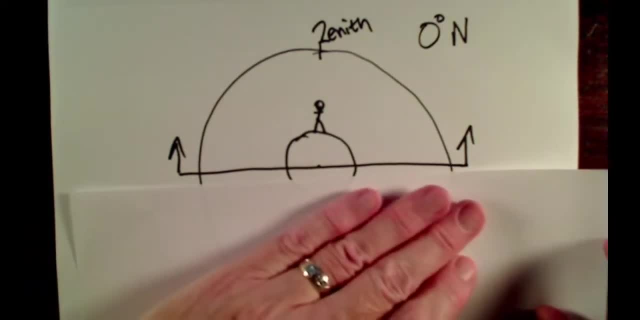 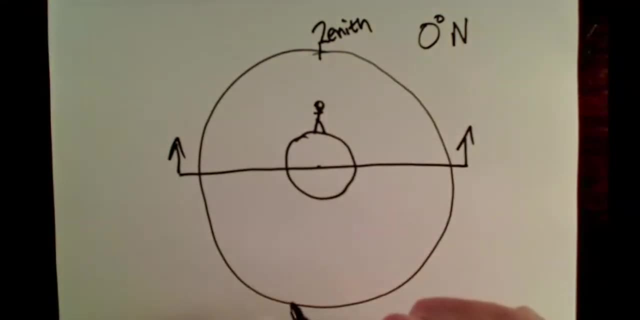 down here. everything down here is hidden from view. So that's their view of the sky. Let's mark the earth underneath the observer. Step five: well, I know that they're standing on the equator, so the Earth's equator must be running like this, because 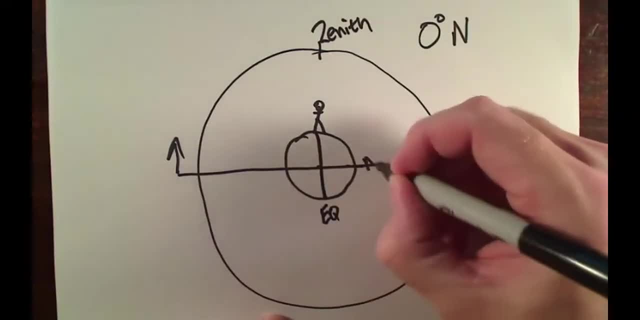 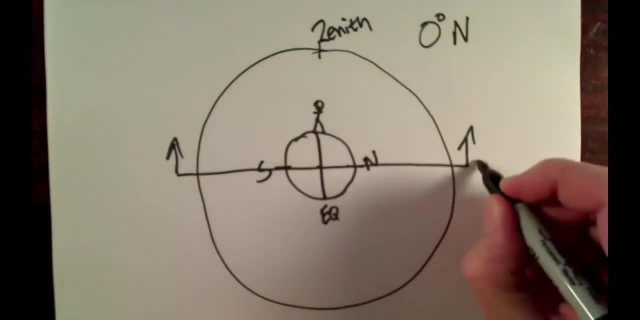 they are standing on the equator, And that means that this is the North Pole and this is the South Pole. Again, you could switch north and south doesn't really matter there. but once I've put the north over here, then this becomes the North Celestial Pole, that becomes the South Celestial Pole, and this 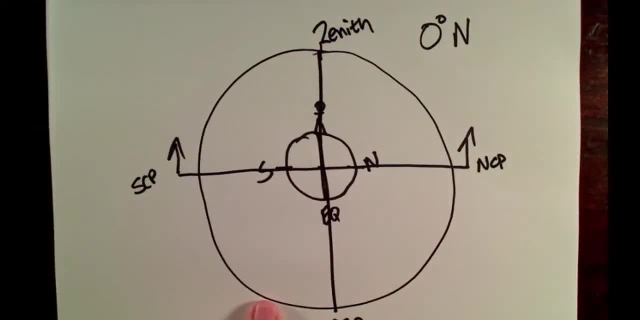 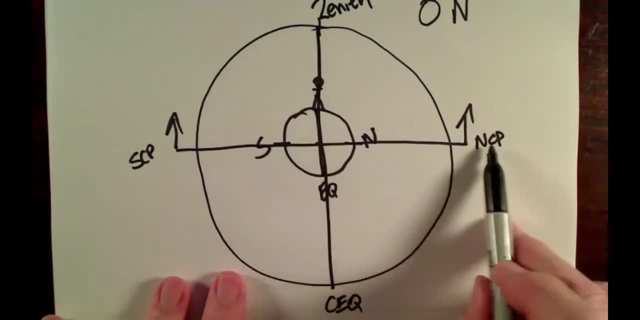 becomes the Celestial Equator. So for an observer standing on the Earth's equator, two things. the first thing is you'll notice that the North Pole, the North Celestial Pole, is right on your horizon, right there. The question is, what is the altitude of the North Celestial Pole? 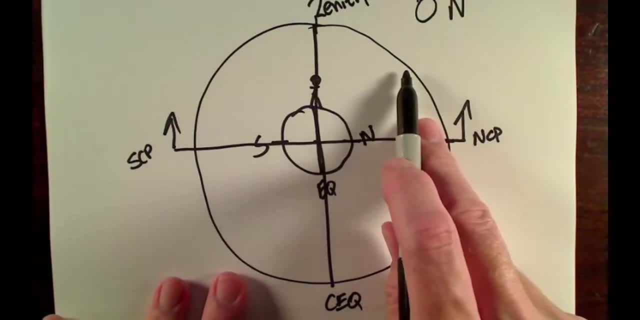 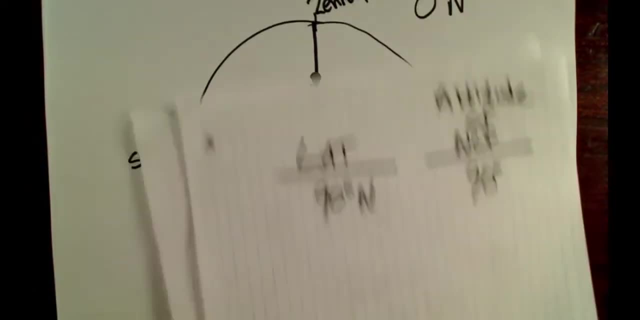 Well, altitude is how high something is above the horizon. Since it's sitting on the horizon here, the altitude is zero degrees. So, going back to my little chart that we had started a minute ago, the altitude when you're on the equator, the. 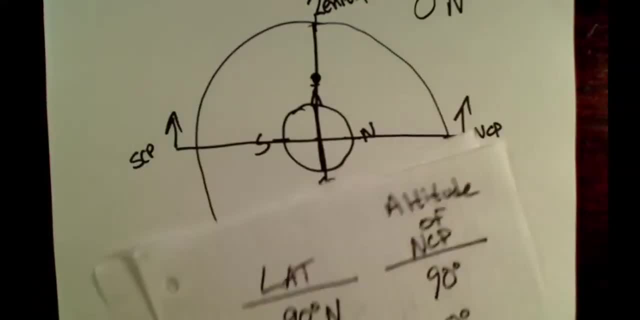 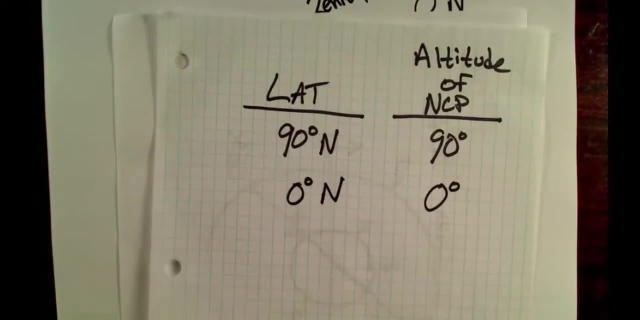 altitude of the Celestial Pol is zero degrees when you're on the equator. and well, what's your latitude? Well, your latitude is zero degrees. And now you will notice an interesting pattern starting to develop, That is, the altitude of the north celestial pole in your 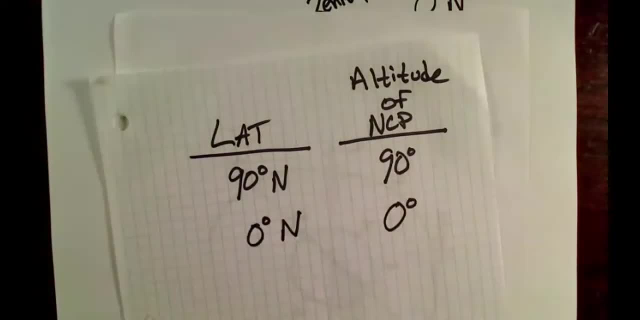 sky appears to be equal to your latitude on the surface of the earth. That is to determine what latitude you are at all. you have to do is measure how high up the pole is in the sky. When you are on the equator, the north celestial pole has an altitude of zero degrees. It's right on your 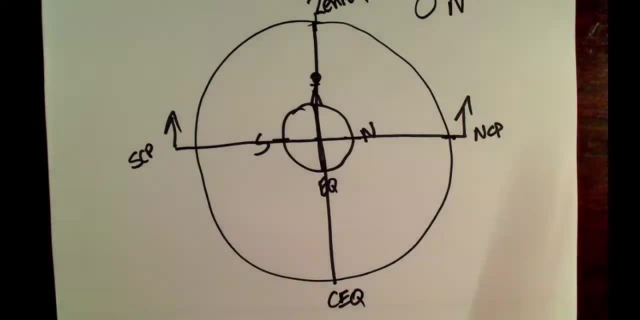 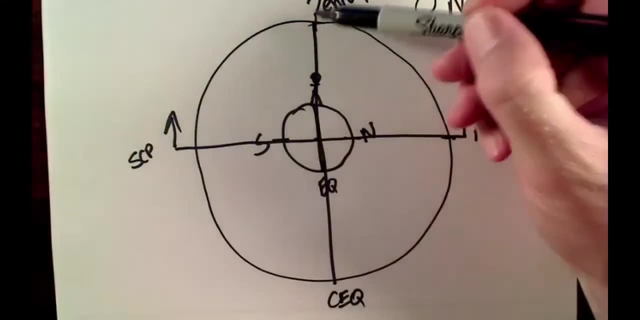 horizon. That is, if you were looking at the north celestial pole and you looked out there, you would see it right on your horizon. It has an altitude of zero degrees. when you are at zero degrees north, Cutting through your zenith, straight overhead is the celestial equator. So because you are standing, 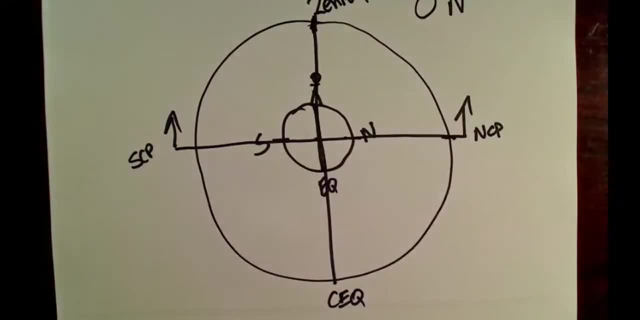 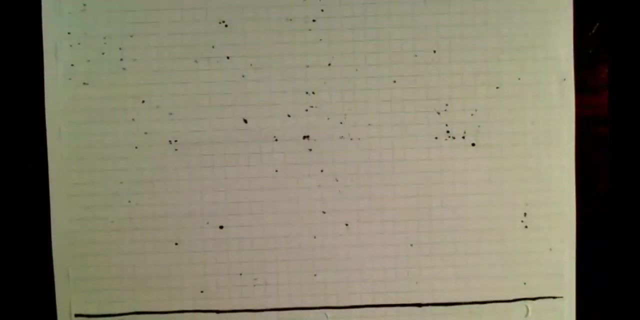 on the earth's equator. the celestial equator goes straight overhead, right through your zenith right there. So that is a celestial sphere for someone at zero degrees north. I'm zero degrees north on the equator, So let's go back for a second and let's draw our celestial. 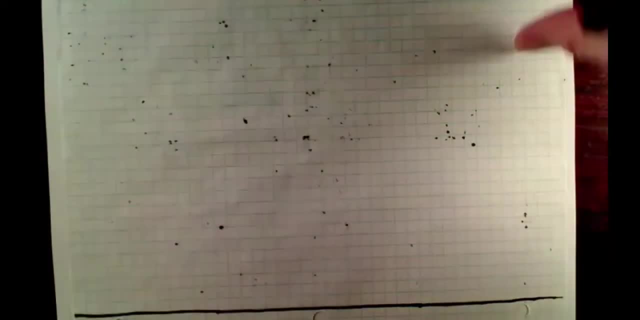 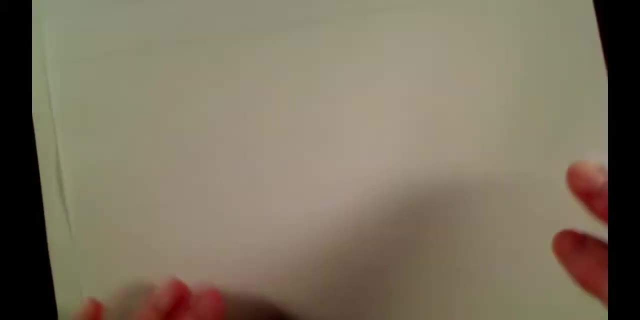 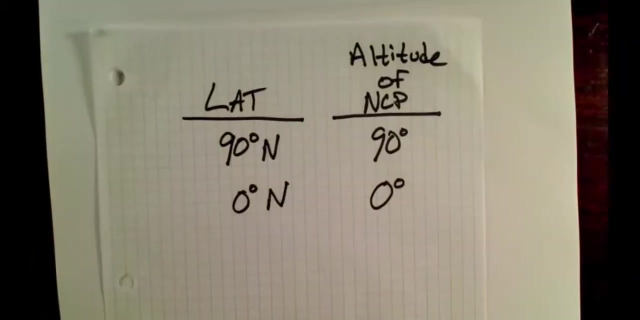 sphere for 38 degrees north latitude again for here in Charlottesville, And let's see what that celestial sphere would look like this time, taking into account this interesting piece of information that the altitude of the north celestial pole is equivalent to our latitude on earth. So let's draw. 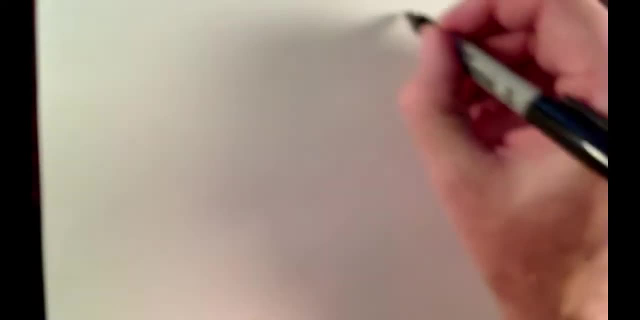 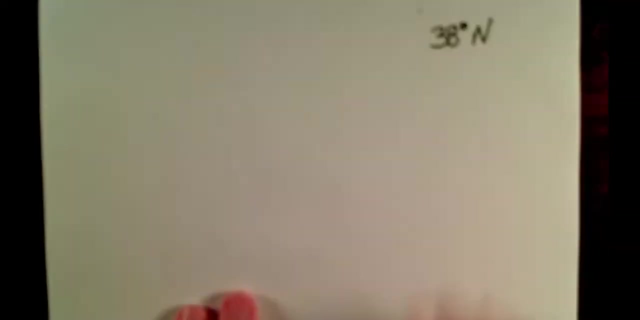 that celestial sphere again. So let's go back. Always good practice to do one for 38 degrees north, because that's where we live here in Charlottesville, So this is one that we should be really familiar with. So, step number one: draw the earth. 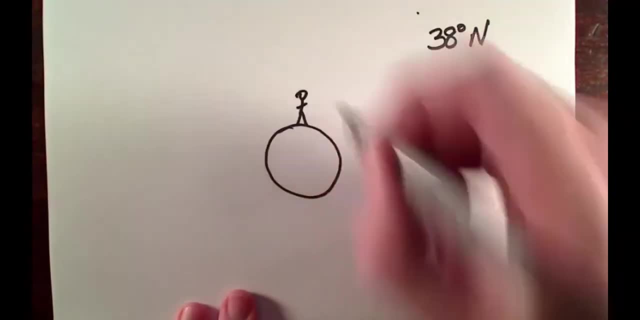 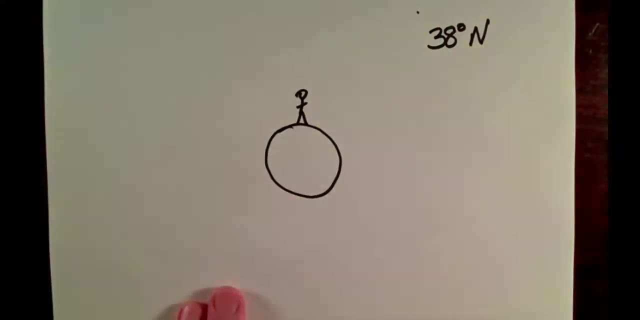 Step number two: draw our observer standing on top of the earth. In fact, now would be a good time to pause this video and finish your 38 degree north celestial sphere and then see if it matches mine. I'm going to go ahead and push ahead here, but 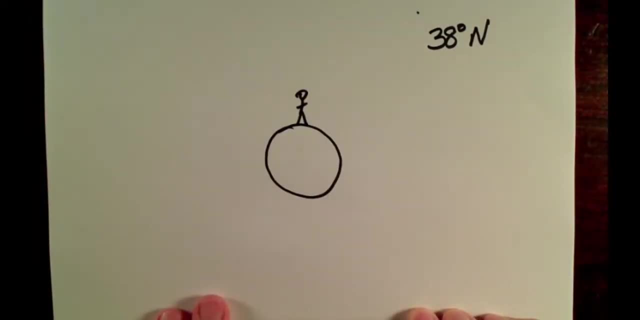 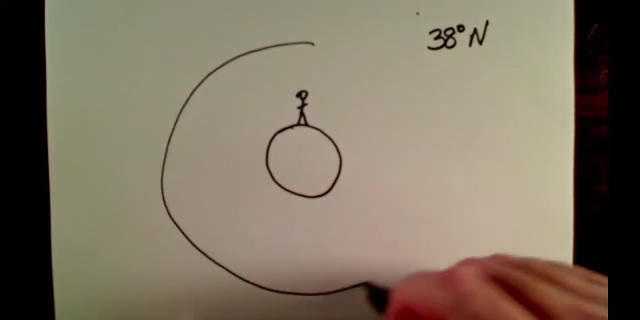 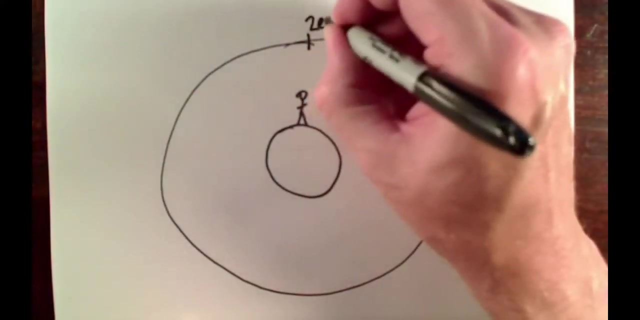 But if you'd like, now would be a good time to pause and do that, All right. Next step, number three: draw the celestial sphere around it. There's our celestial sphere. Number four: mark the observer's zenith and draw in their horizon. 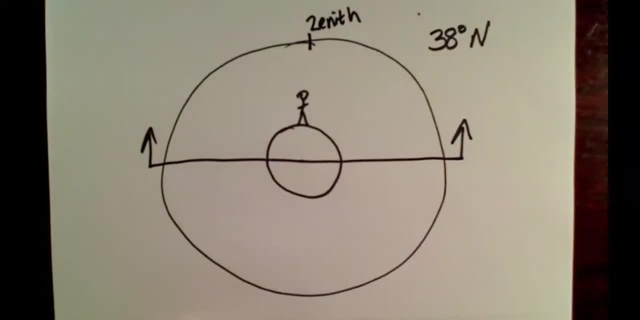 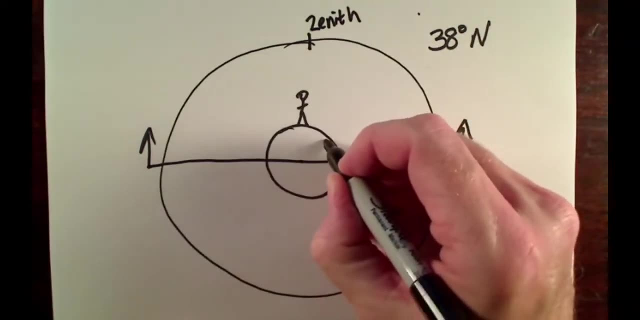 They can see everything above the line. They can't see anything down here. Now orient the Earth underneath the observer. Well, 38 degrees north. We've done this a couple times, so now I'm pretty familiar with it. So the north pole goes over here. 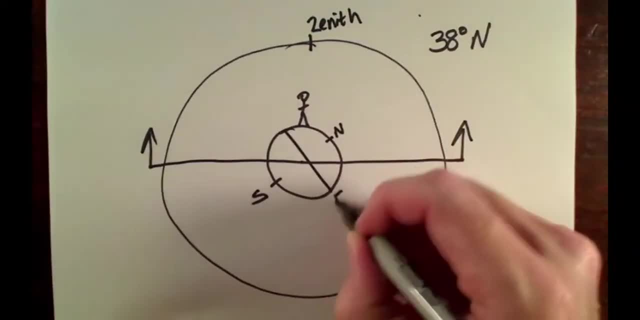 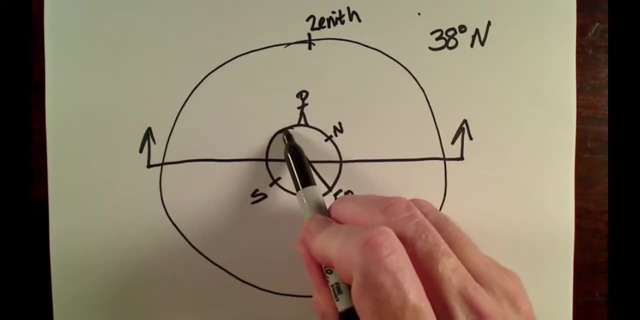 The south pole goes over there. That is the Earth's equator right there. So I have oriented myself. So my observer here they're closer to the equator than they are to the pole. If I start on the equator and head to the north, I get to my observer. 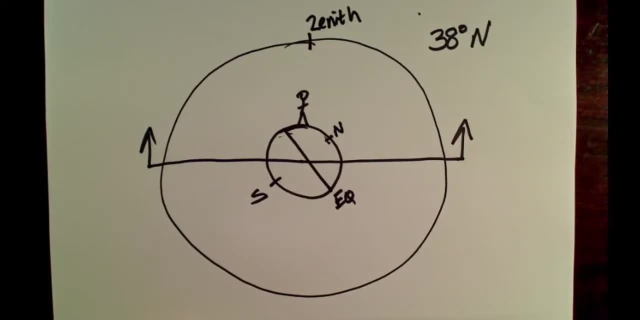 So they are north of the equator. So my observer there is at 38 degrees north latitude. So I've oriented the Earth And now I can do things like draw in the north celestial the pole, the south celestial pole, and I can draw in the celestial equator. 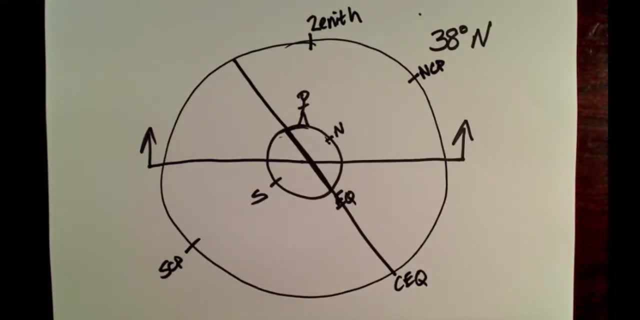 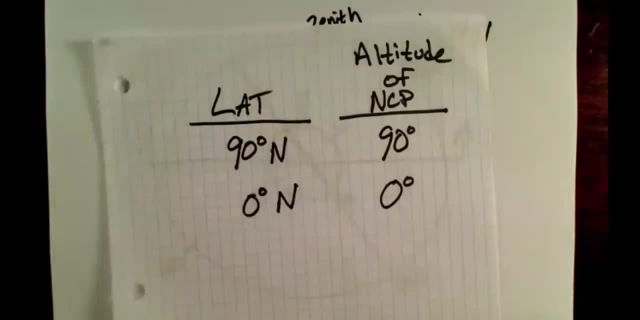 So that is the celestial sphere that we drew for an observer at 38 degrees north a little while ago. but here's the key Now. let's take into account this new piece of information here: that the latitude, that the altitude of the pole in your sky is equivalent to your. 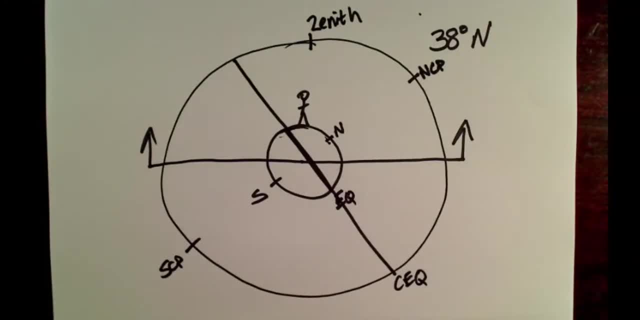 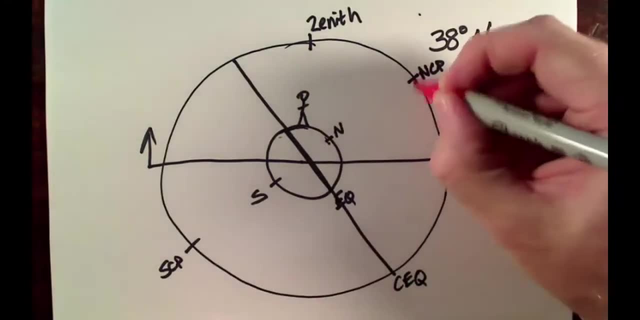 latitude on the surface of the Earth. What does that mean? What that means Is the altitude of the north celestial pole. Let me use a different color right here. This angle: the altitude of the north celestial pole, how high it is in the sky. 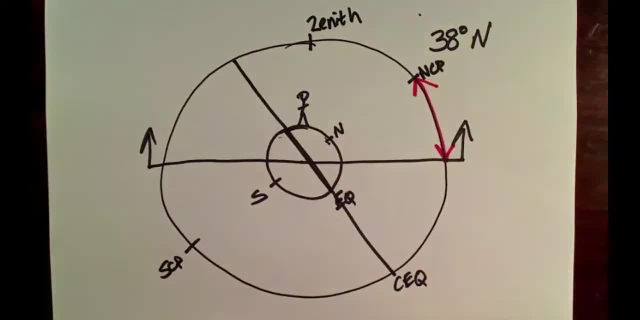 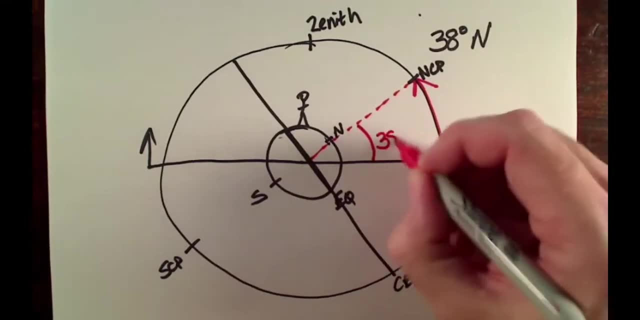 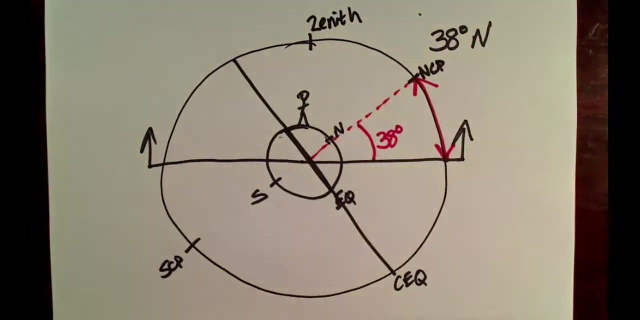 that is starting on your horizon, measuring up to the north celestial pole. right there, that angle, this angle right here, is 38 degrees. The north celestial pole, when you are at a latitude of 38 degrees north, appears 38 degrees up in the sky. 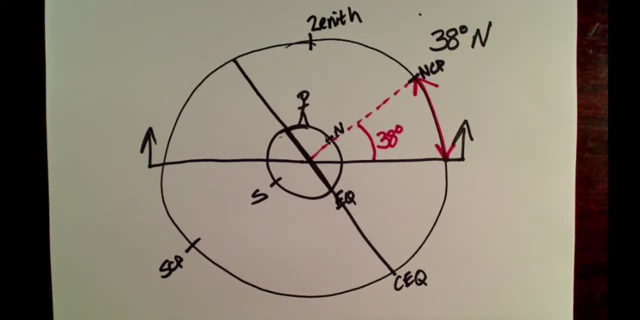 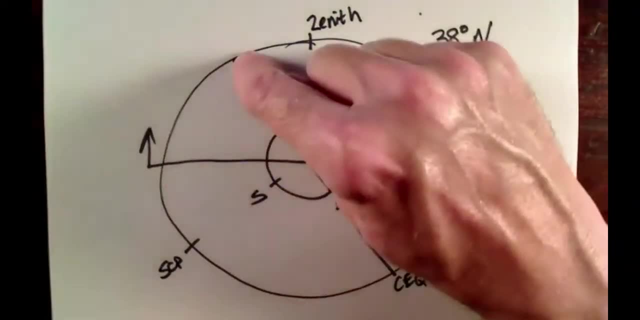 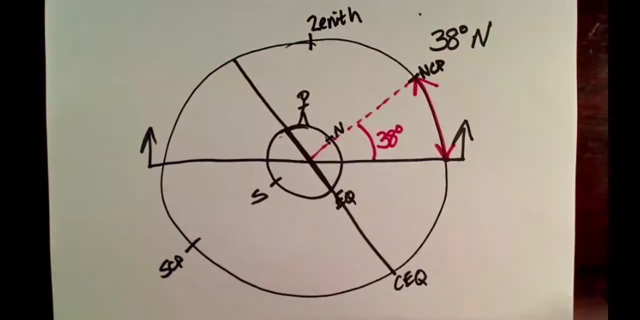 So that is how high the pole is in the sky Now. we can also figure out from that how high the equator is. right here Now. the equator is important because we are going to find later on that when it comes to our seasons, the Sun wanders north and south of the equator. 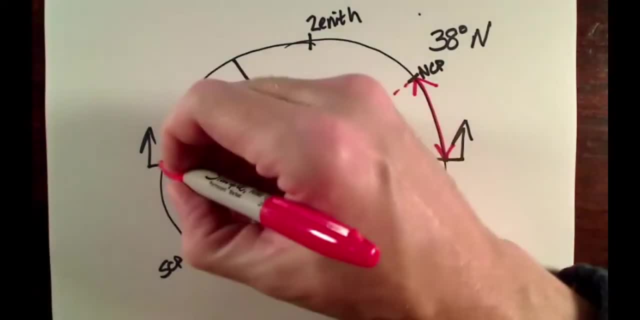 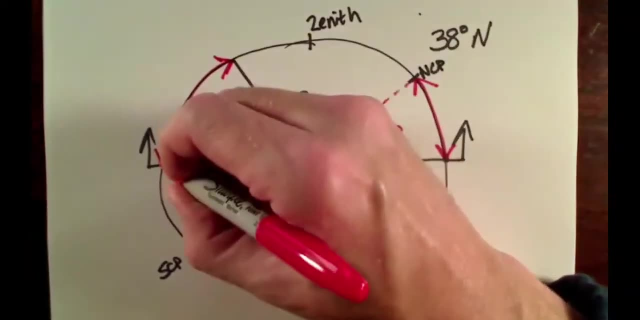 And we will always be indexing the Sun with respect to the equator. So we need to know this angle right here. How high up is the Equator in the sky at it's maximum altitude? Passing the Sun out of the equator altitude? right So the equator starts in the east, goes across the sky, sets in the 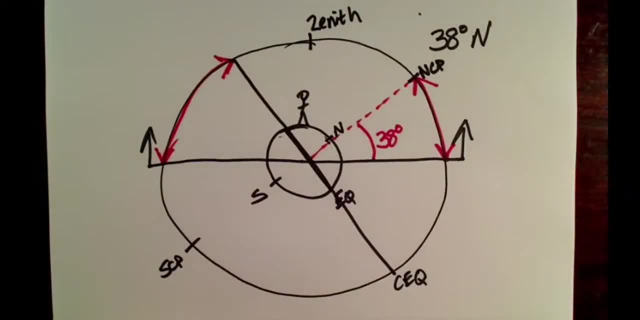 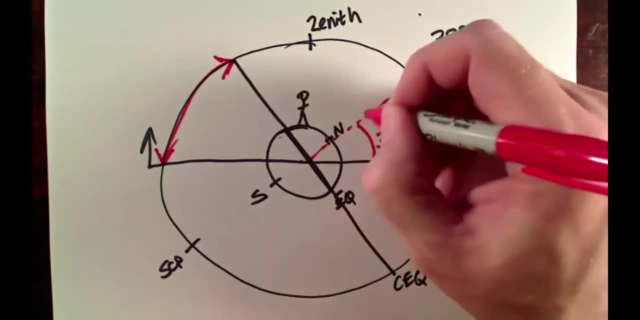 west. But the question is, how high up does the equator get right there? What is that angle? The question is, how am I going to figure out what that angle is? I know this one's 38. What is this angle right here, This angle from the north celestial pole to the? 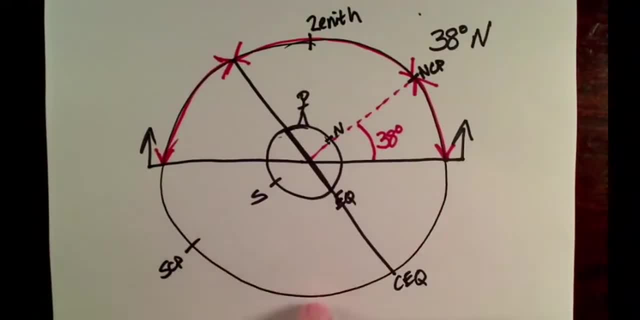 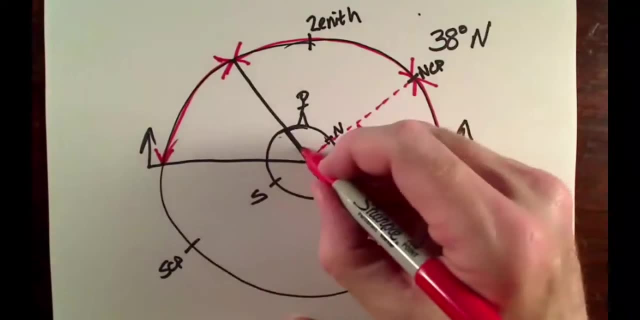 equator. Well, now think about that one for a second. So first of all, just look at it. Equator north pole, Equator north pole. You probably noticed right away that that's a right angle. Now it makes sense right, Because the angle from the equator to the 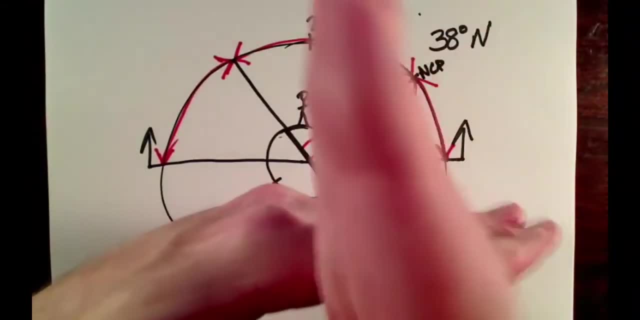 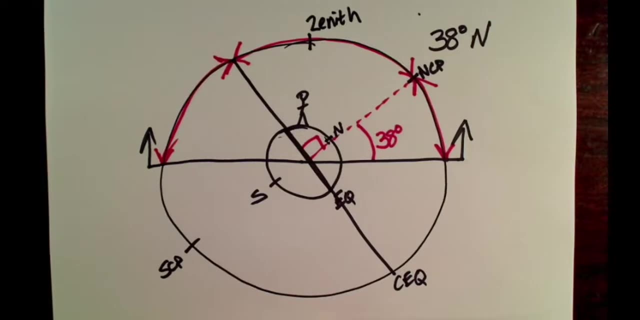 north pole. if I think about the equator and the north pole, they're at right angles to one another. They're always at right angles to one another. No matter where you are on Earth. the angle from the north pole to the equator is always 90 degrees. If this, 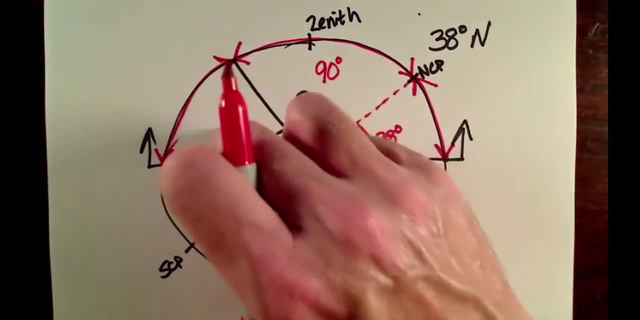 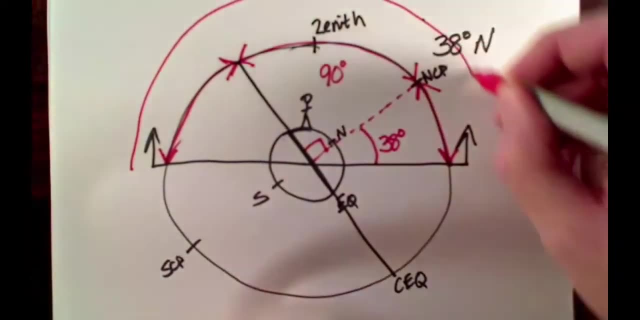 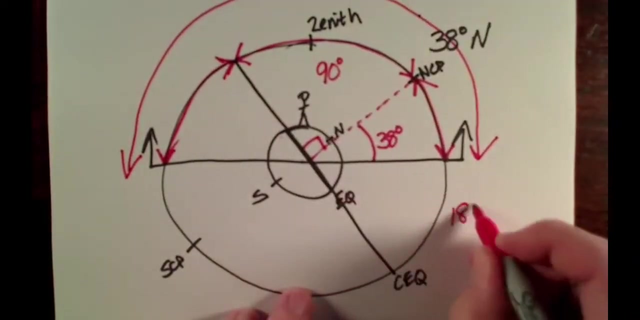 angle is 38 and that angle is 90, that allows us to figure out what this angle is, And the reason is that from here, all the way across to here, is half a circle. That angle, that total, is 180 degrees: Half a circle And 180 degrees. it's made up of three angles. 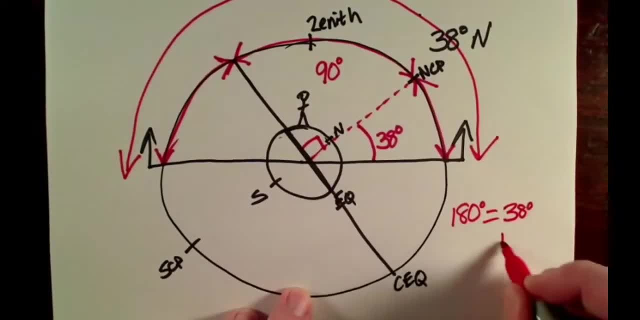 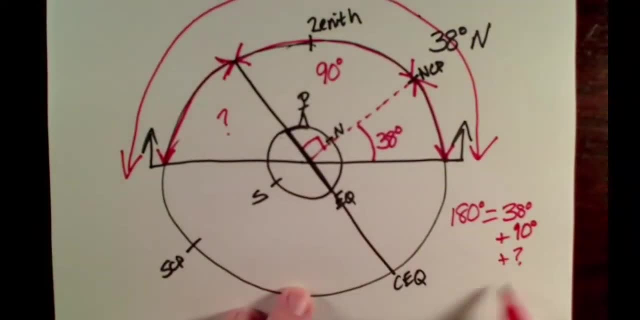 It's made up of this one which is 38,, plus this one which is 90,, plus this one that I want to know. Okay, So what is this angle that I want to know? Well, it's whatever will make these all add up to 180 degrees, Or, another way to put it, 180 degrees minus. 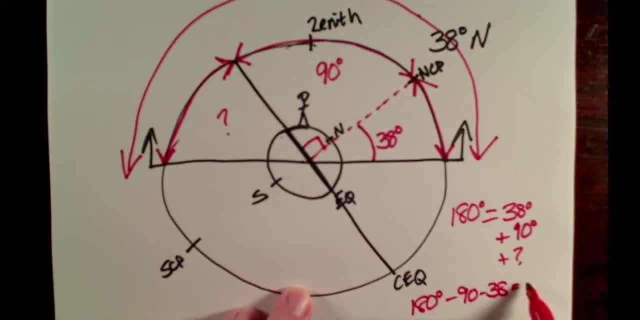 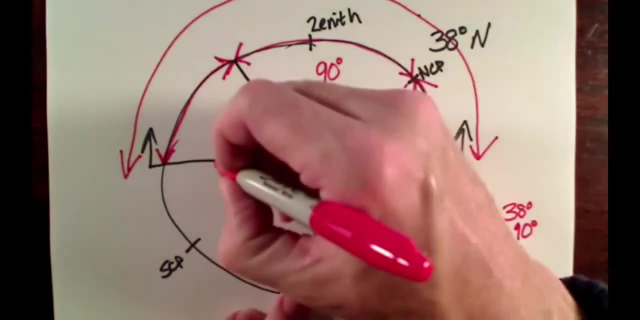 90, and minus 38, is what that angle that I want to know is. And so 180 minus 90 is 90.. 90 minus 38 is 52 degrees. So this angle right here is 52 degrees, The celestial equator. 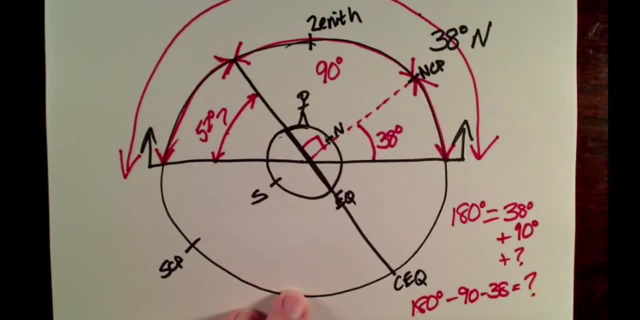 is 52 degrees up in the sky as seen from Charlottesville. So now we've been able to use our simple celestial sphere diagram to make all kinds of really cool measurements. We've determined that the north pole is 38 degrees up. The angle from the pole to the 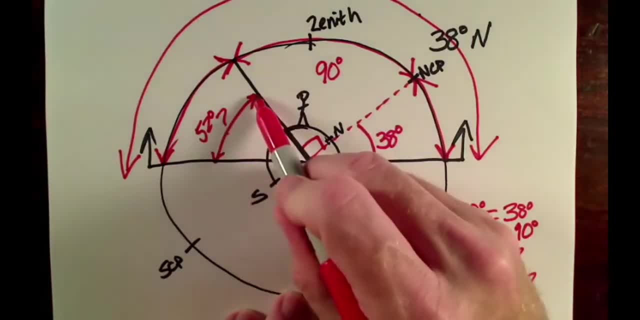 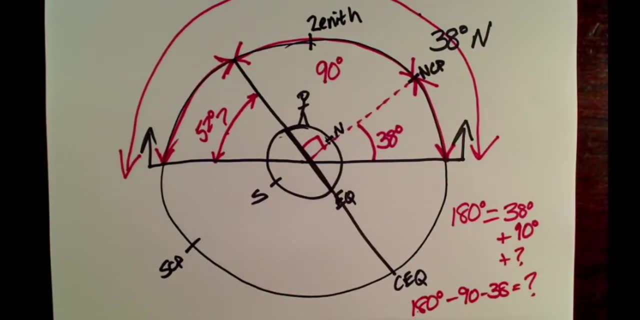 equator is always going to be 90, and we've determined that the equator is 52 degrees up in our sky. So that is the full celestial sphere diagram for Charlottesville. Later on, when we study the sun, we'll learn that the north pole is always going to be 90 degrees. 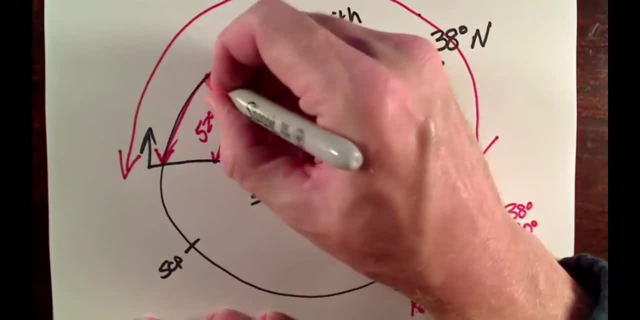 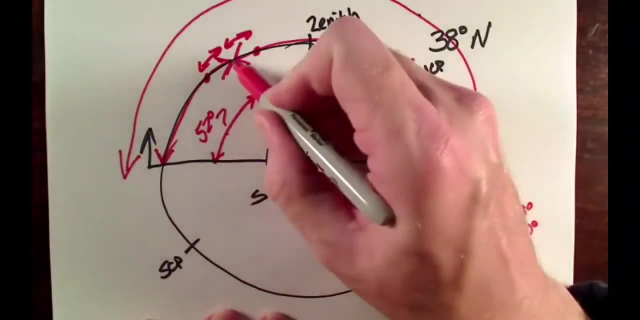 we will find that the Sun can be north of the equator or it can be south of the equator, If we know how far north of the equator it is or how far south of the equator it is, and we know that the equator 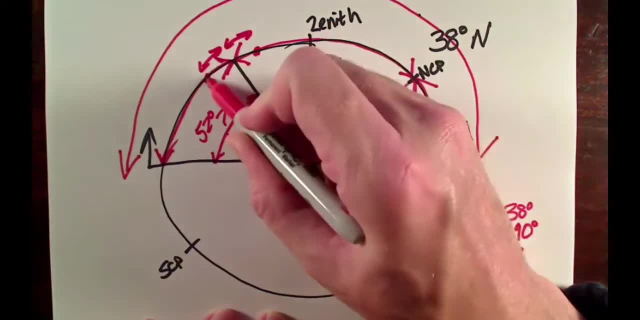 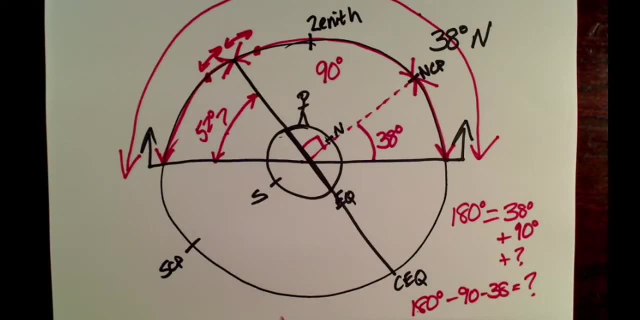 is 52 degrees up. we can either add to that or subtract from it to find out how high the Sun is in our sky at the different seasons. But we're gonna save that for a future lecture. We'll come back to these kinds of diagrams later on. 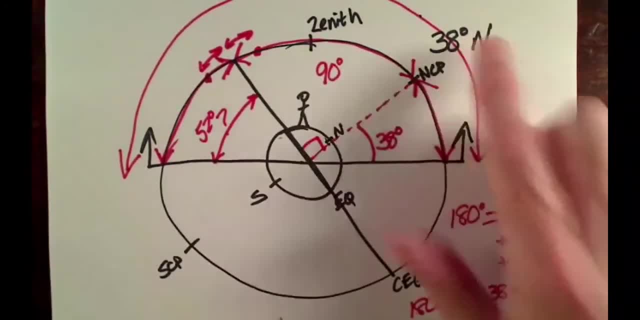 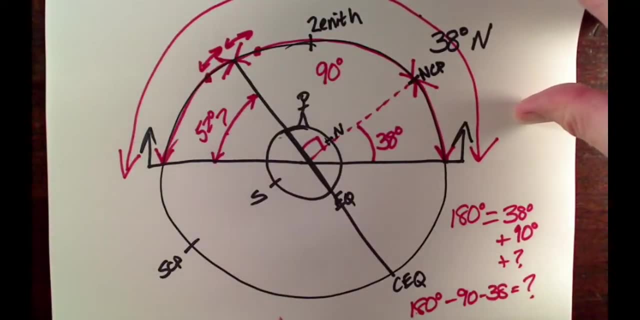 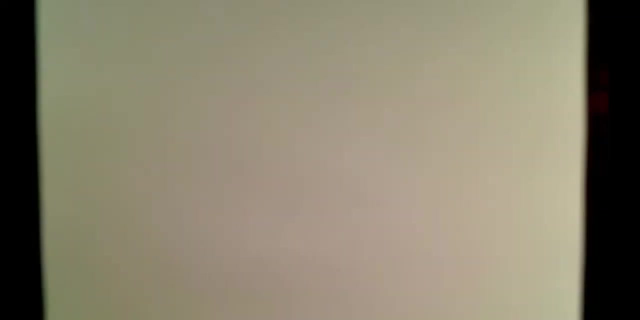 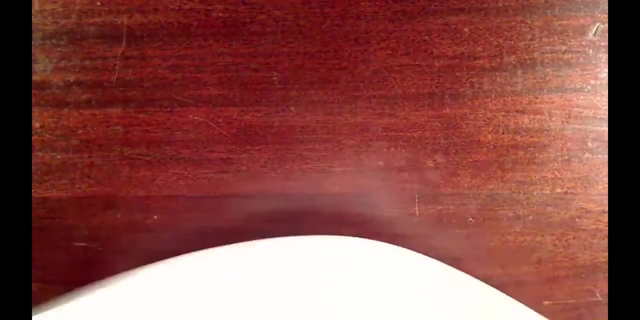 So that is our celestial sphere for 38 degrees north, adding in this new information about some of these angles. So let's do a couple more celestial spheres for practice, just to see what they look like. Let's do a celestial sphere for somebody at. let's go back to our celestial sphere for somebody at the equator. 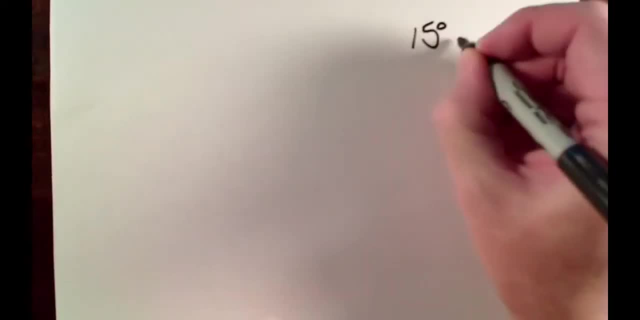 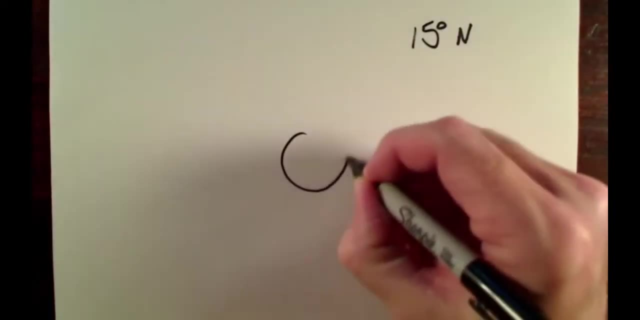 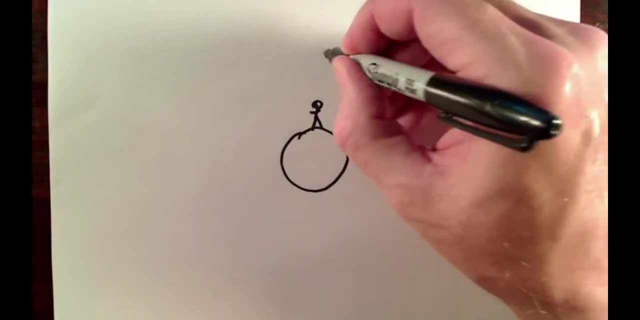 Somebody at 15 degrees north. So let's do 15 degrees north latitude and see what the celestial sphere looks like. So step one, draw the Earth. Step two: draw my observer standing straight up and down on the Earth. Step three: draw the celestial sphere around my observer. 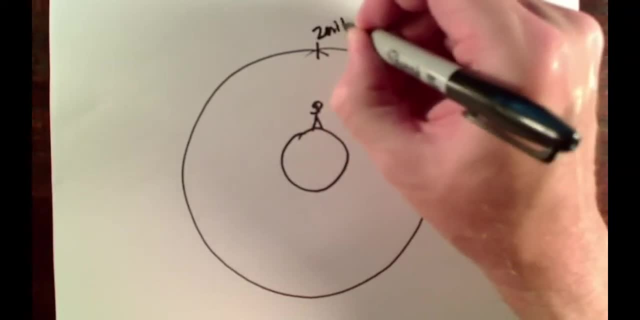 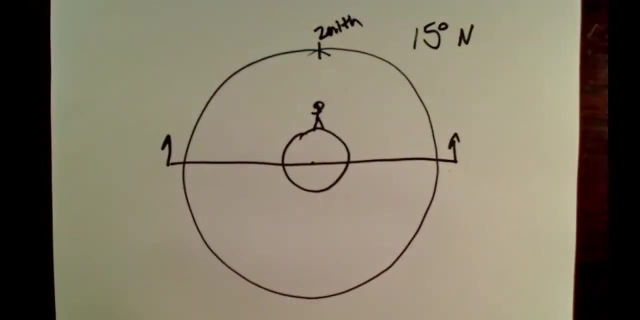 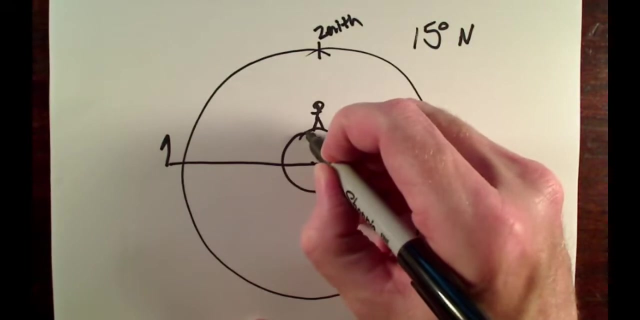 Step four: mark the observer's zenith and mark their horizon. Step five: orient the Earth underneath the observer At 15 degrees north. I'm a lot closer to the equator than I am into the pole, So I'm going to draw the equator like that, and that means that the north pole is over here and the south pole is right there. 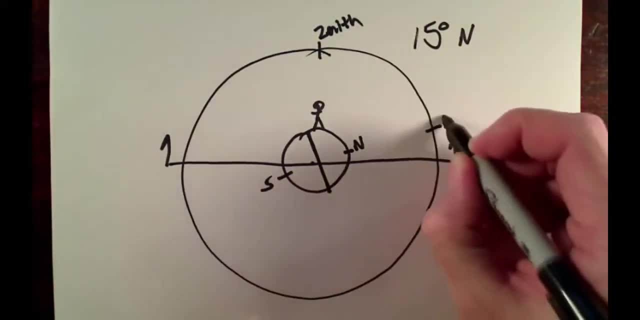 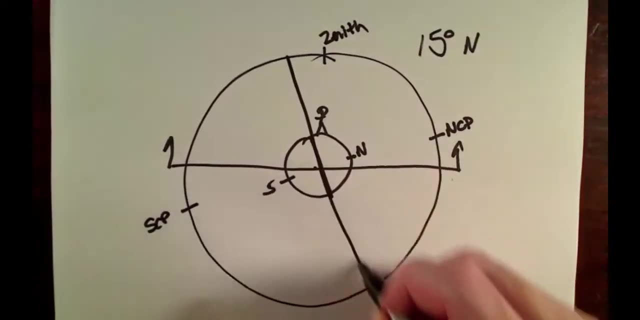 And now I'm going to extend the north pole out to get the north celestial pole, Extend the south pole out to get the south celestial pole right there And extend the equator out to get the celestial equator And then go ahead and draw the equator. 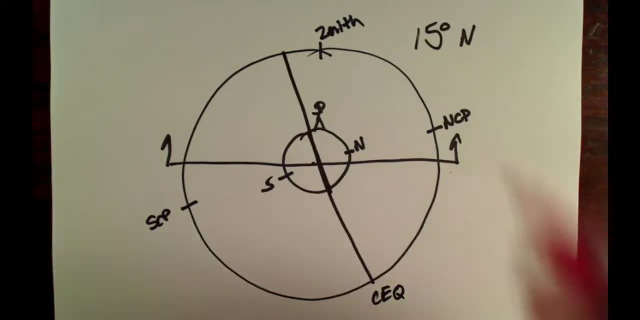 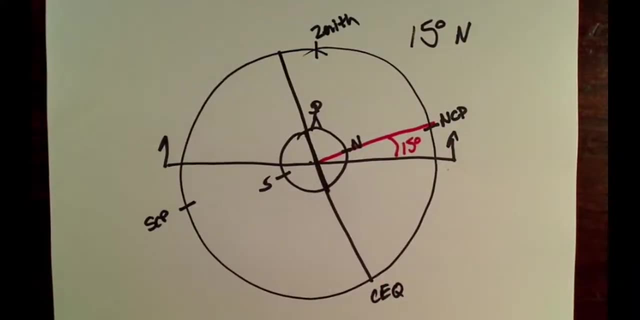 Going back to the things that I learned a second ago, the north pole in the sky, because I'm at 15 degrees north. the north pole in the sky is only 15 degrees above the horizon, Not very far. Remember your outstretched hand. 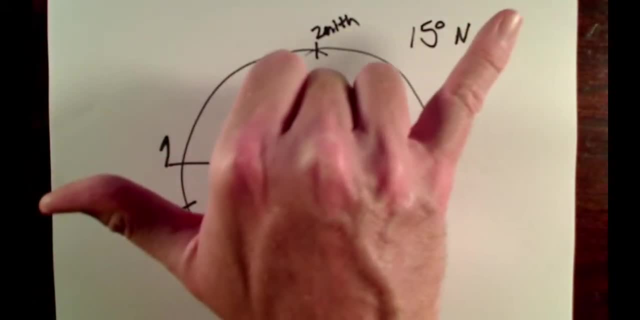 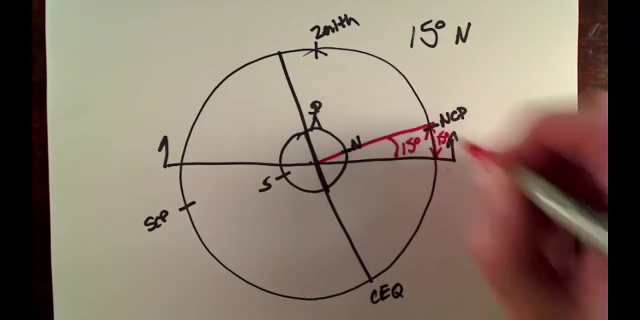 If you stretch your hand out like this, it's 20 degrees from side to side. So the pole is less than that above the horizon, So it's only 15 degrees. This angle right here is 15 degrees up. What is the angle from the pole to the equator? 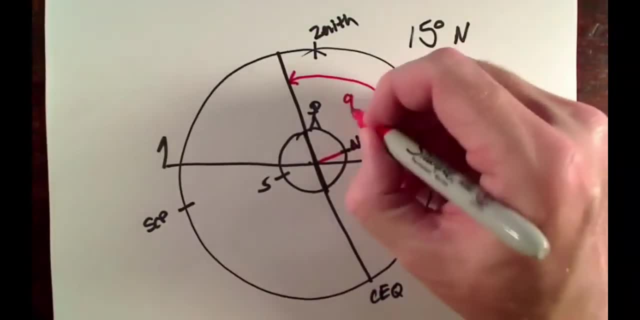 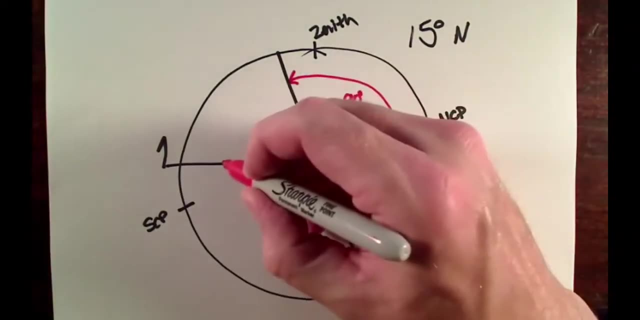 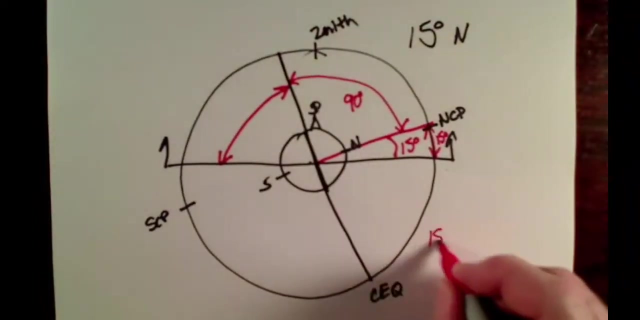 What is it? It's 90 degrees. It's always 90 degrees, no matter where you are on Earth. And if this is 90 degrees and that is 15 degrees, that means that the equator here must be this angle plus that one. plus that one have to equal 180 degrees. 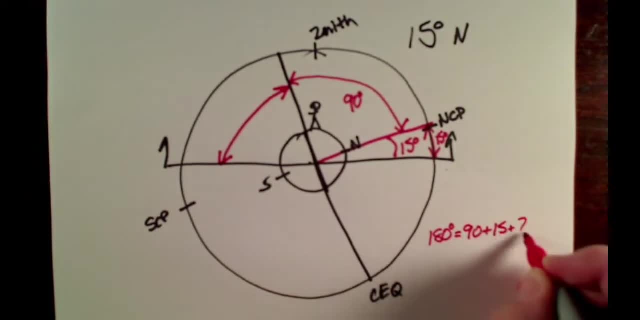 Has to be equal to 90 plus 15 plus the angle that I want to know. So the angle that I want to know is 180 minus 90 minus 15, which is 180 minus 90 is 90.. 90 minus minus 15 is 75 degrees. 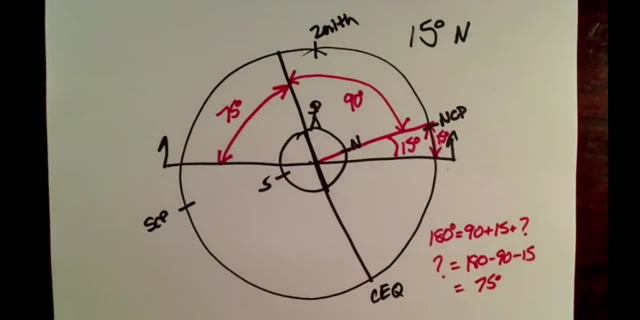 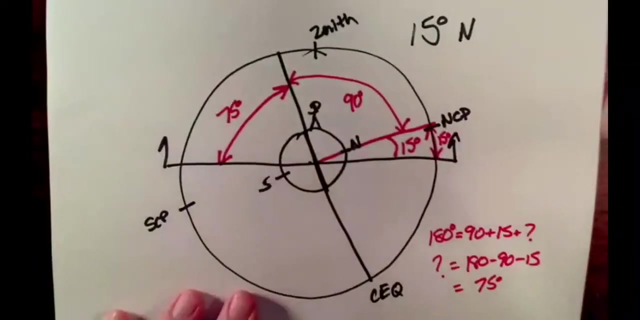 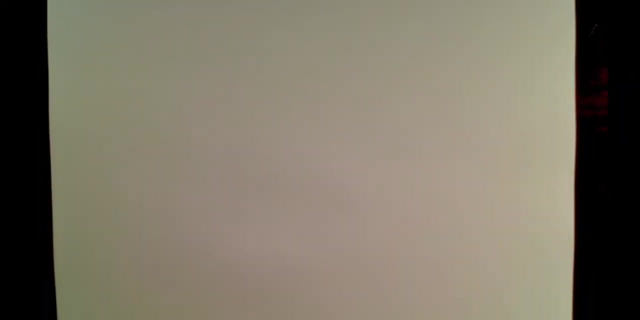 So this is 75 degrees up in the sky. So that is a celestial sphere for somebody at 15 degrees north latitude. Let me finish by drawing a celestial sphere for someone in Australia, particularly someone at, let's say, 38 degrees south latitude. 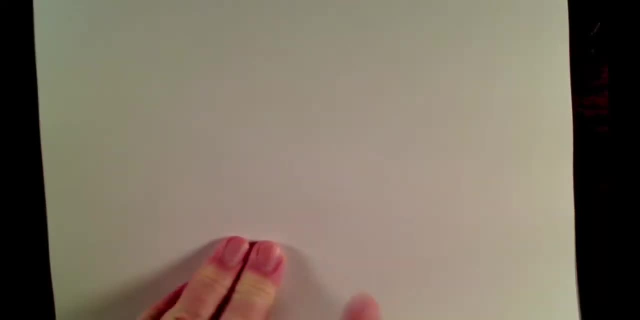 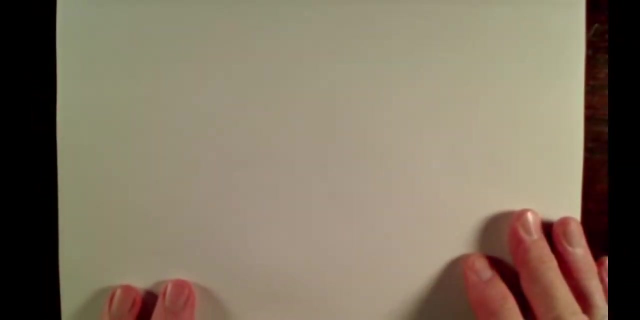 They're the same latitude in the southern hemisphere that we are here in the northern hemisphere. So here in the northern hemisphere we're at 38 degrees north, And in the southern hemisphere they are, of course, at 38 degrees south. 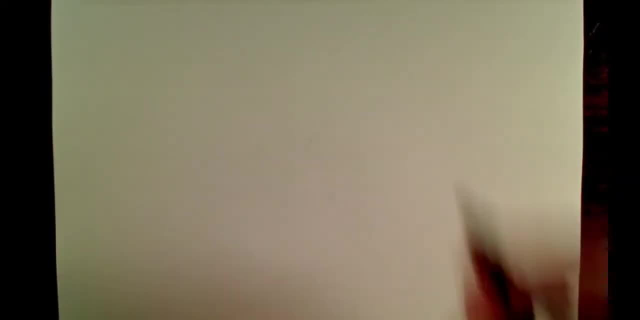 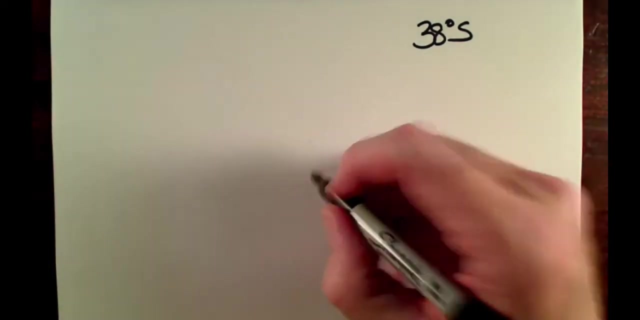 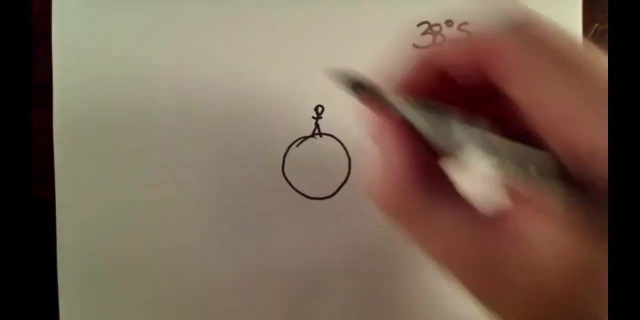 So let's draw that celestial sphere for them. So this is a celestial sphere for someone at 38 degrees south latitude. What does that look like? All right, Step one: draw the Earth. Step two: draw my observer standing straight up and down. 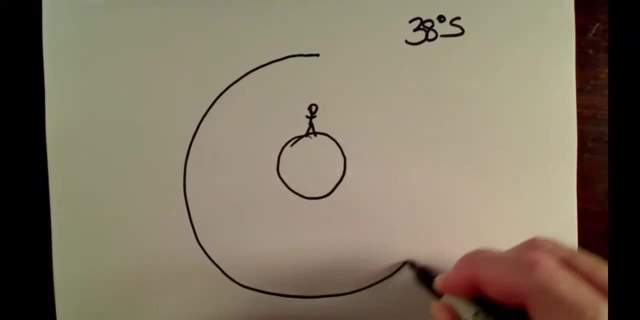 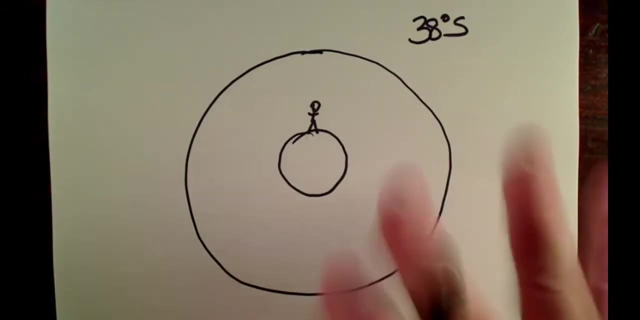 Step three: draw the celestial sphere Again. notice that I always do this in exactly the same order every time, so I don't forget anything, And by doing it the same every time, I make sure that I don't miss out on anything important. 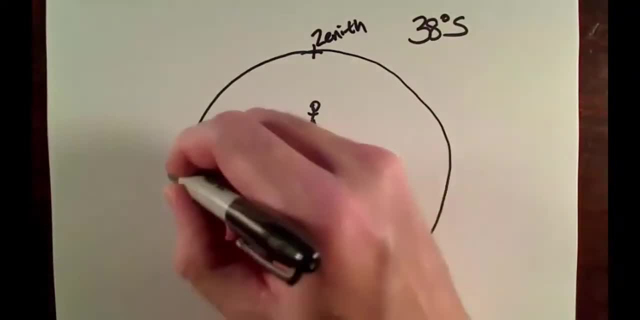 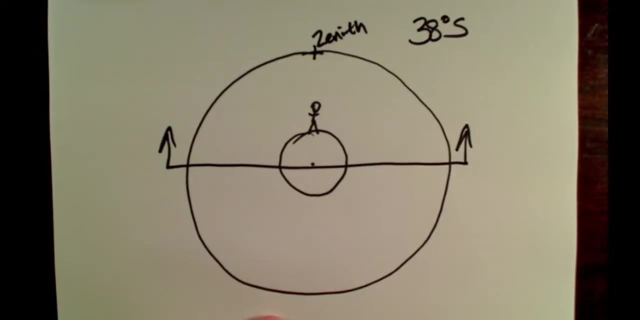 Zenith. Step four: mark the zenith and their horizon. They can see everything above the horizon. They can't see anything below the horizon. Now it gets tricky. Number five: orient the Earth underneath the observer. Okay, They're at 38 degrees south. 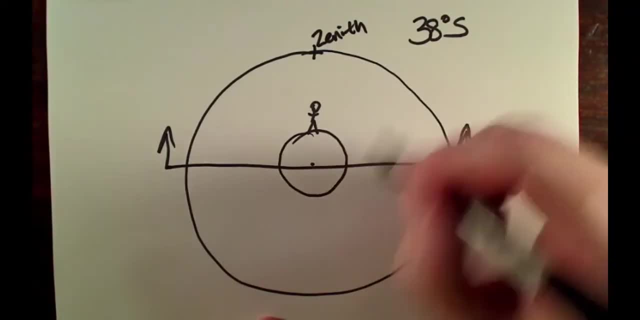 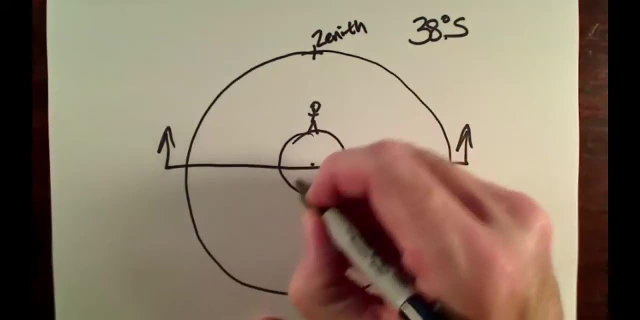 So this time I'm going to reverse things a little bit and I'm going to say: okay, 38 degrees south, They are halfway between the equator and the south pole. So if I orient the Earth like this, if I draw the equator like this, 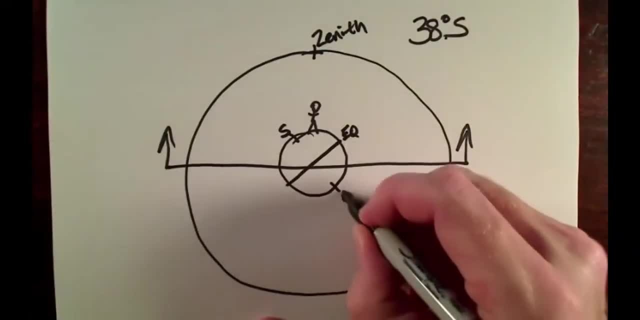 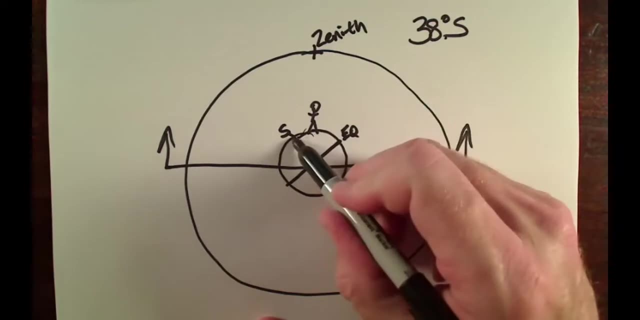 that would be the south pole right there, and that would be the north pole right there. Now that makes sense, right? I go from the equator to the south pole. They're about halfway in between the equator and the south pole. 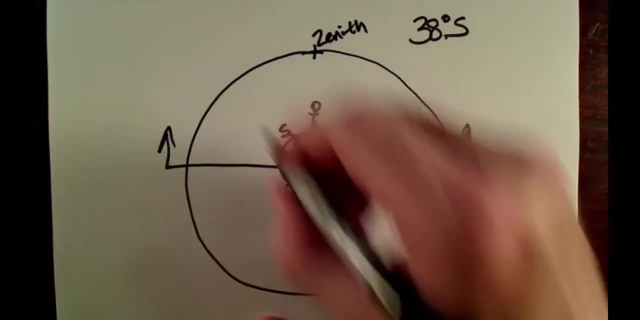 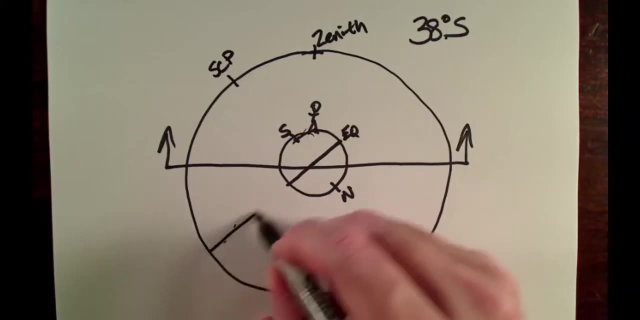 So that looks pretty good for somebody at 38 degrees south, Which means that this is the south celestial pole, this is the north celestial pole down here, and then this is the celestial equator. The last thing we need to figure out is how high the south pole is in the sky. 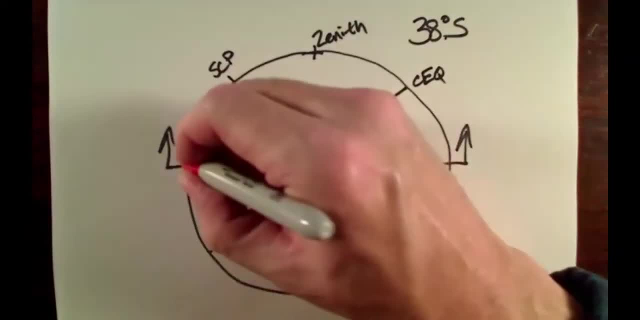 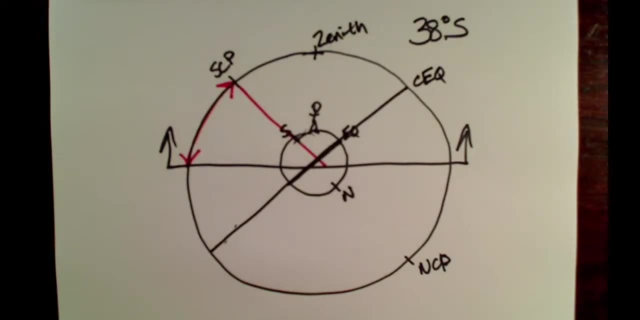 What is this angle right here? That is, how high up is the south pole? Well, you can do the same exercise we did before. You could draw a celestial sphere for someone standing on the south pole and you would see that the altitude of the south celestial pole. 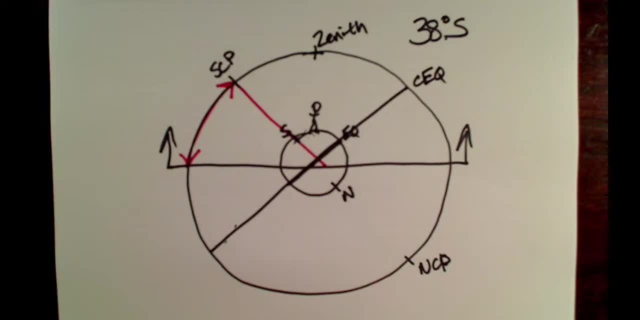 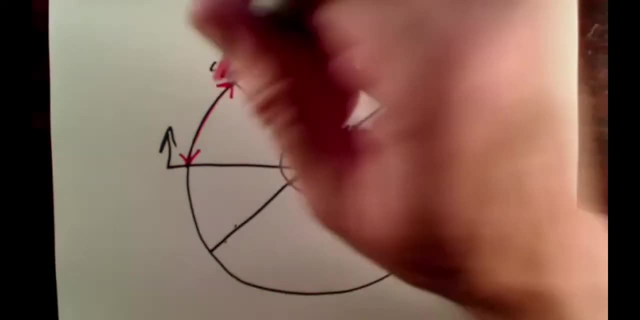 when you are at a latitude of 90 degrees south. the altitude of the south pole is 90 degrees, And what that means is in the southern hemisphere the same rule holds. If you can find the south celestial pole in the sky, its altitude, how high it is above the horizon. 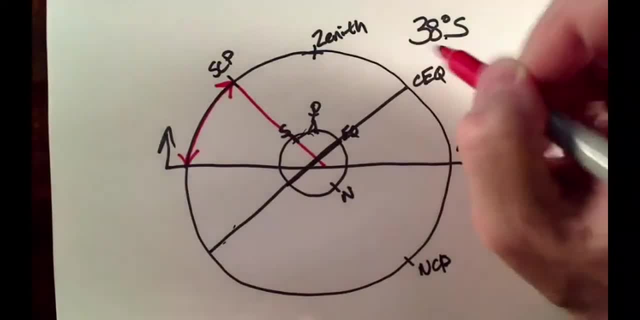 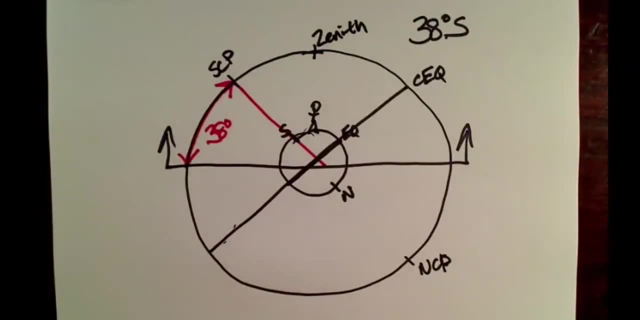 is the same as your latitude. So if they are 38 degrees south, that means that this angle is 38 degrees. That is, the south pole is 38 degrees up in their sky, The angle from the south celestial pole all the way around to the equator, right here. 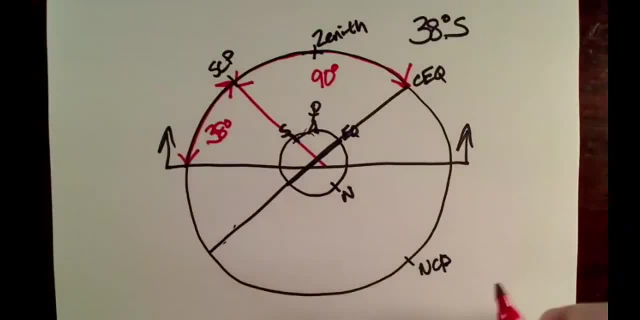 well, that's going to be 90 degrees. It's always 90 degrees And that means the celestial equator. right here, that celestial equator must be 52 degrees up in the sky, So they see the sky just like we do in Charlottesville. 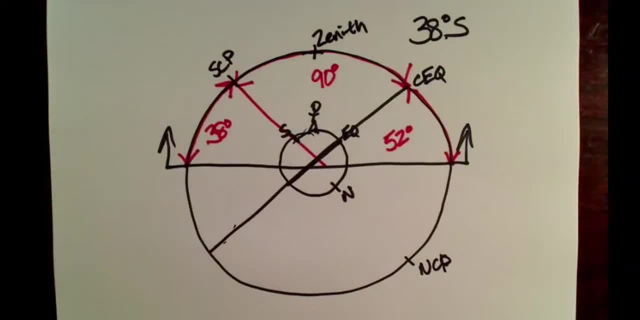 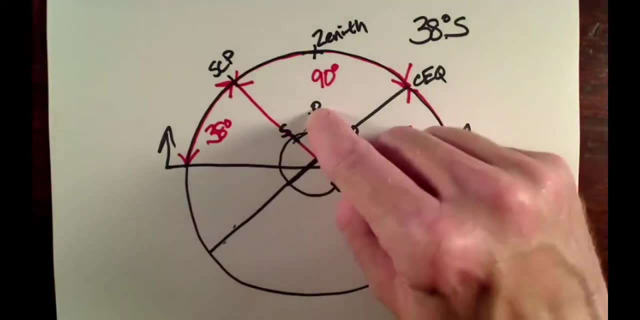 Our pole is 38 degrees up and their pole is 38 degrees up. Our equator is 52 degrees up. their equator is 52 degrees up. The difference is is, when they look in their sky, they see the pole in the southern sky, whereas we see the pole in the northern sky. 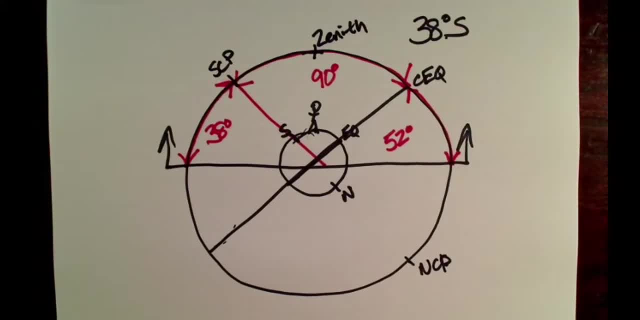 The north celestial pole for them is down here, below their horizon. And remember, the Earth is turning around this axis right. So the Earth is turning round and round this axis right here. That means the north celestial pole never rises above their horizon. 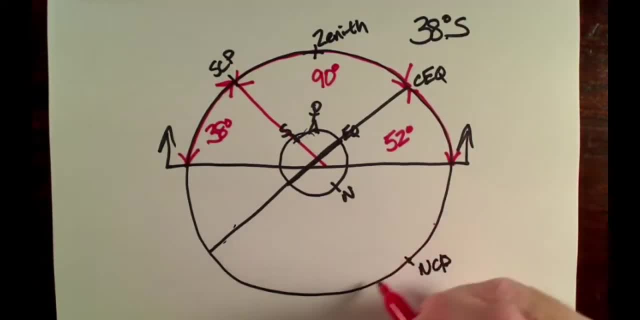 The Big Dipper, which is located close to the pole. here, as the day goes on, the Big Dipper goes round and round the pole, like this down here. the Big Dipper never rises above their horizon. Some of the stars in the northern sky here go round and round and never rise up. 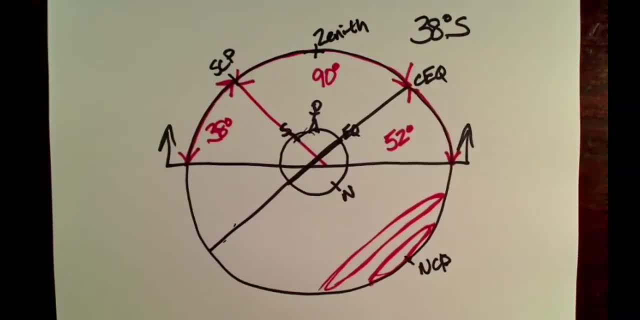 So in the southern hemisphere they don't see some of the northern constellations that we can see In particular. in fact, exactly the constellations that we see here in Charlottesville that are circumpolar are invisible to people that are at the same latitude in the southern hemisphere. 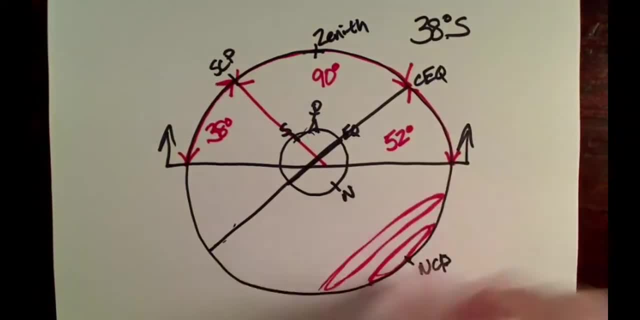 So our circumpolar constellations that never set, never rise for someone at 38 degrees south latitude. The same is true, of course, when we do the celestial sphere in the opposite direction, When we take that celestial sphere for someone at 38 degrees north latitude. 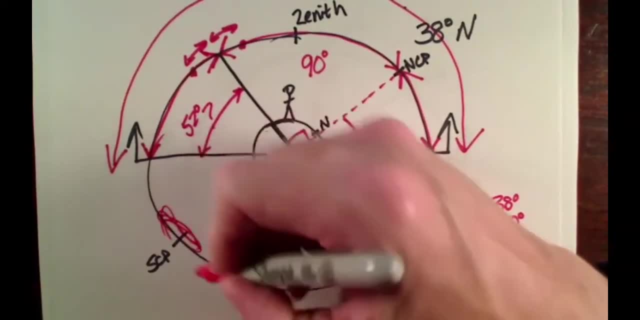 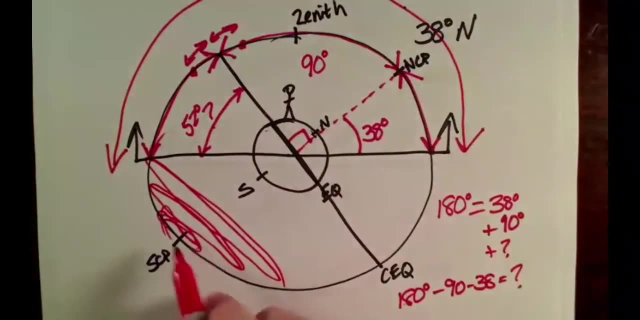 all these constellations around the south celestial pole are going round and round down here and they never rise up and we never get to see them. So one of those, for example, is the beautiful Southern Cross that's down here in the southern sky. 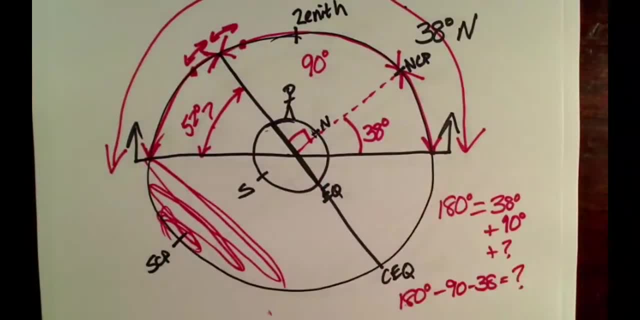 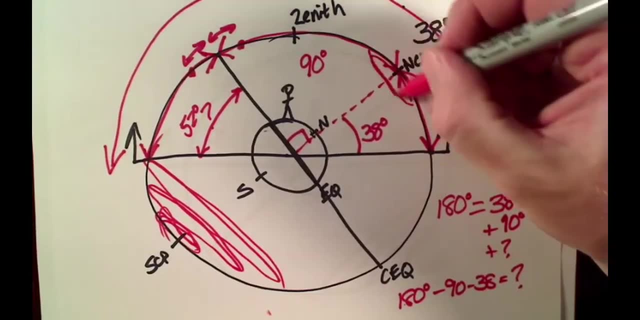 It goes round and round and round and it never rises above our horizon. It's eternally invisible to us. On the other hand, there are all these stars up here that, as they go round and round the sky, as the Earth turns. 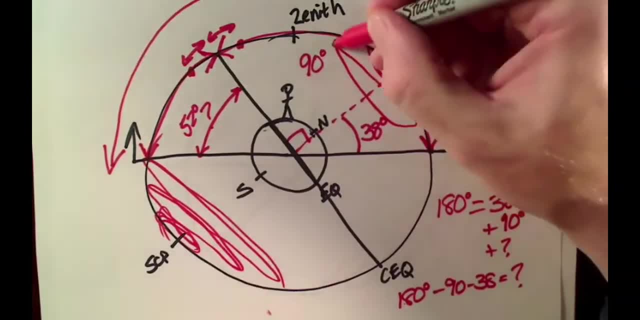 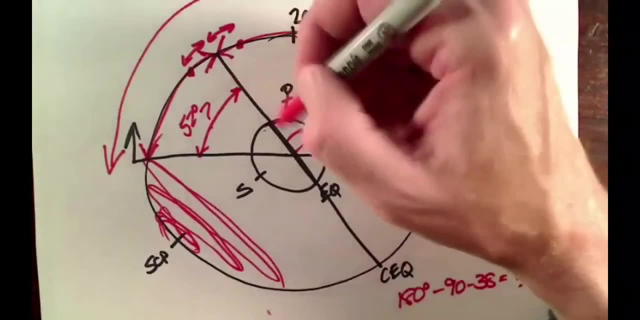 they are eternally visible to us. They're always visible. These are the circumpolar constellations as they go round and round the sky up here, And then most of the stars, especially those around the equator right here. they do set below the horizon. 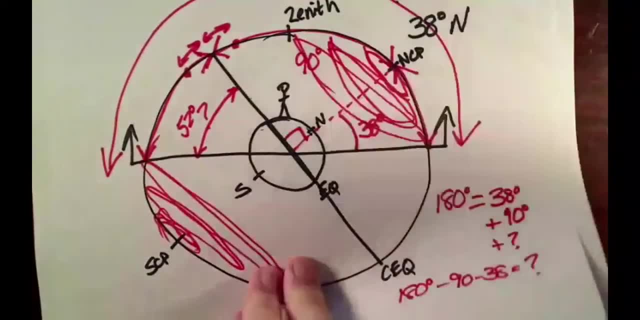 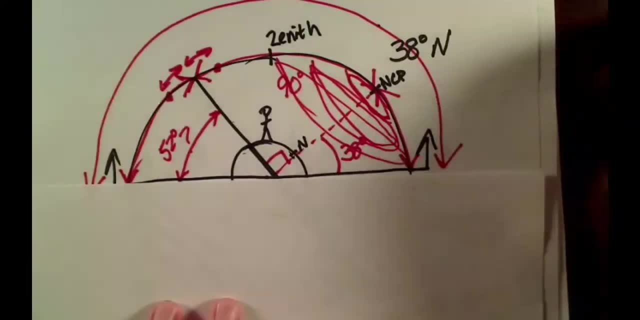 So we've got the horizon right here. Let me grab a clean piece of paper Right. We can see everything above the horizon. We can't see anything below the horizon. So what happens for most stars is they rise, they move across the sky. 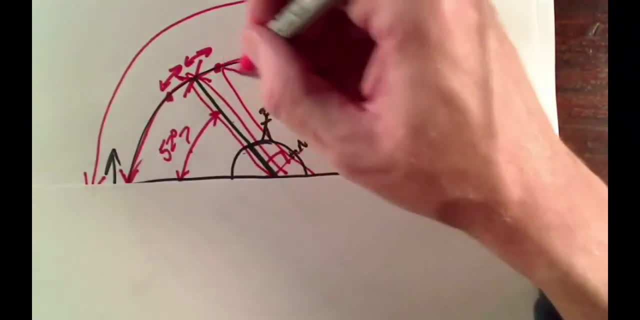 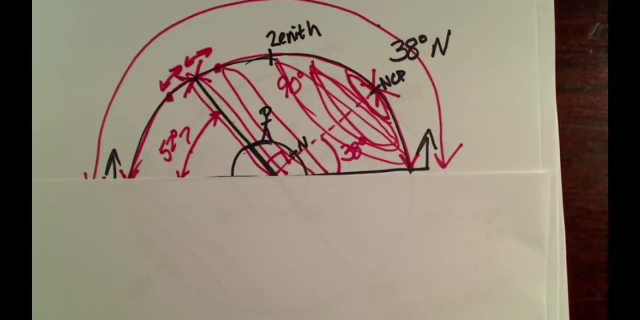 and then they set on the other side of the sky, Or they rise, move across the sky and set on the other side of the sky. So those are celestial spheres And a hint about how we will be using celestial spheres when we talk about the seasons later on. 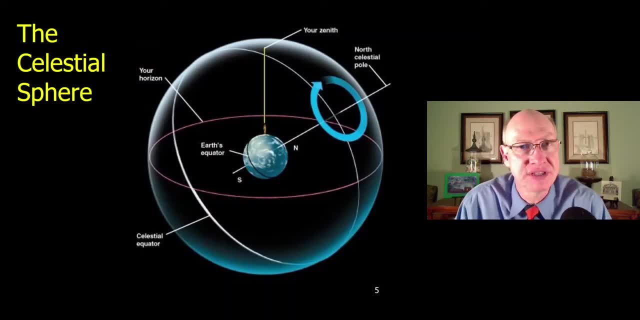 I hope that you've learned from that now how to draw a two-dimensional celestial sphere, and you've also learned some of the basic angles that are needed for orienting our celestial sphere and using it for measurements in the sky. I just want to remind you of a couple key points about the celestial sphere. 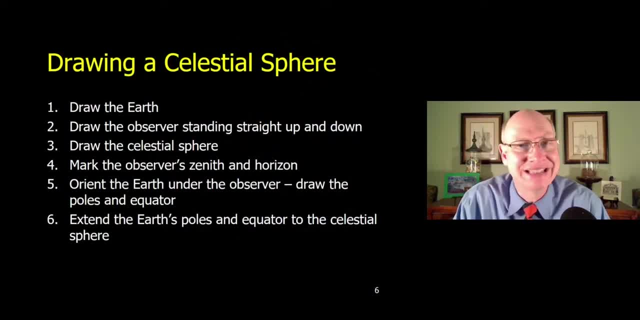 The first one is that I always drew it in exactly the same way. When I was drawing my celestial sphere, I always followed these six steps in this order: Draw the Earth. Draw the observer standing straight up and down. Draw the celestial sphere. 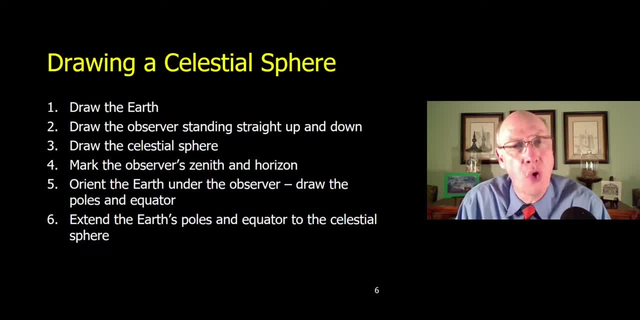 Mark the observer's zenith and horizon, Orient the Earth under the observer, Draw the poles and the equator And then extend the Earth's poles and equator to the celestial sphere. And if you always draw the celestial sphere in this order, you'll always be careful never to forget anything. 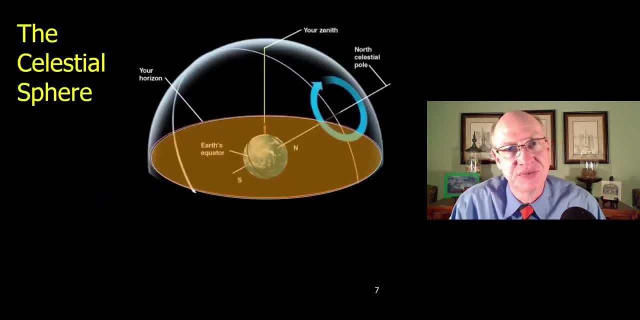 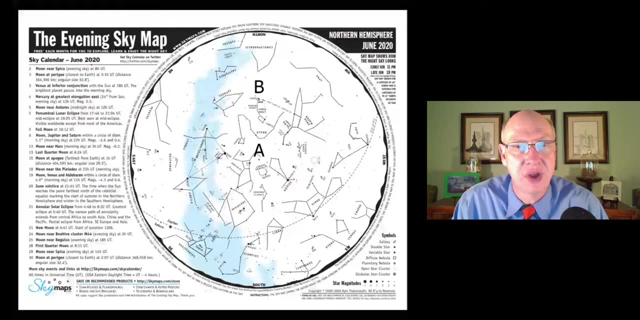 So that is how we draw that two-dimensional celestial sphere. Now I want to take this and generalize this a little bit and think about that star map that we talked about a few weeks ago. I want you to go into learning catalytics right now and I want you to tell me: 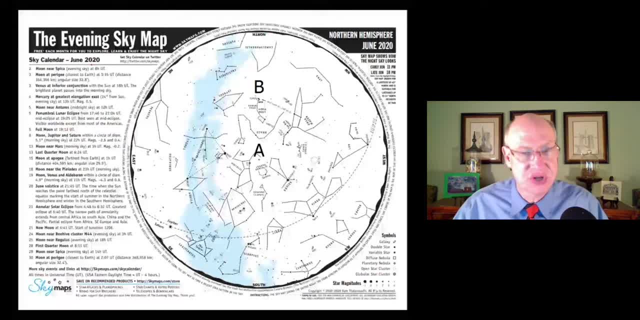 what the points A and B represent on this star chart. So when we looked at the star chart the other day, we talked about using the star chart to observe the night sky And I mentioned, or at least hinted at the time, that there were two points. 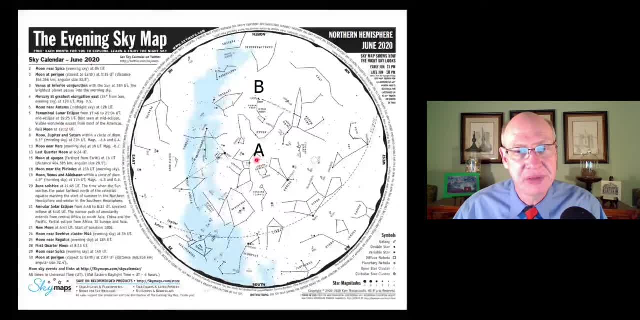 What is this point A that's marked by a little plus sign right here in the middle of the map, And what is this point B right here? So in learning catalytics, take a moment to answer that question. Point A represents what? 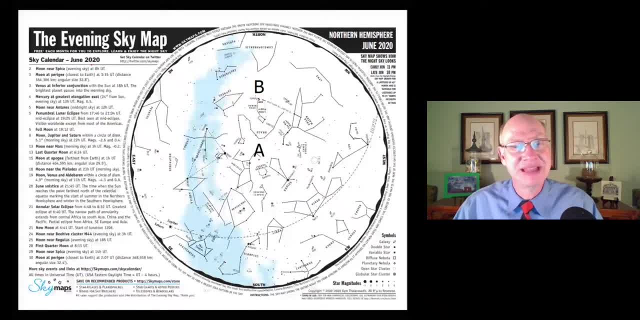 And point B represents what, And you can just type in the answers to those in words in learning catalytics. All right, welcome back from learning catalytics. So those two points on the celestial sphere. point A, of course, represents the zenith. 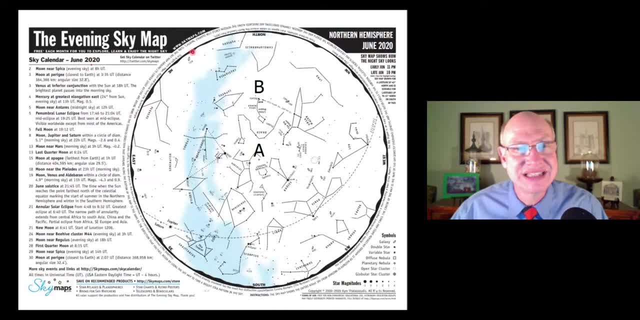 which is the point straight overhead. That is why it is at the center of the map. You will notice your horizon stretching all the way around the map, right here. Your zenith, the point straight overhead, is right here at the center of the map. 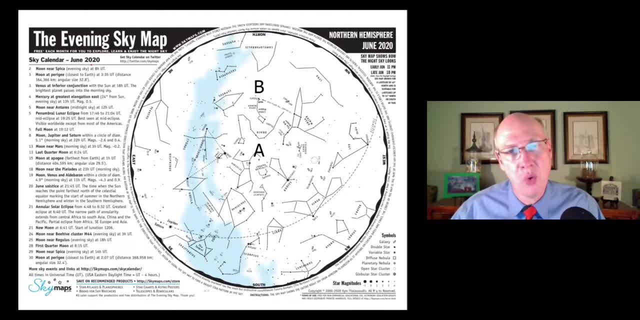 And point B right here represents the north celestial pole up there in the sky, And the important thing to realize is that the north star Polaris is not straight overhead, Because we're at 38 degrees north latitude. it is about 38 degrees above the northern horizon. 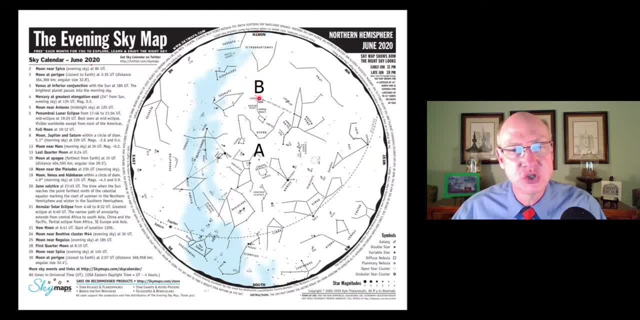 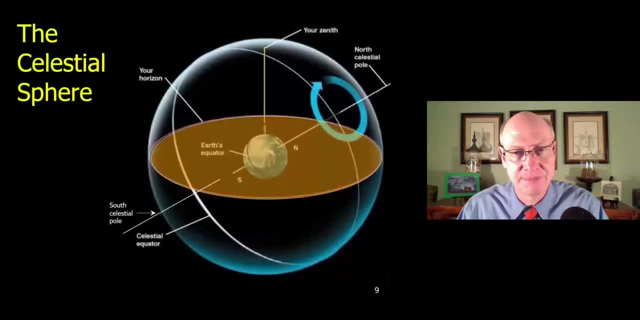 So the angle from the northern horizon to the north celestial pole right here here in Charlottesville is about 38 degrees. That's how high up the pole is in the sky. Another way to put that for our celestial sphere right here is: here's the north pole on the earth. 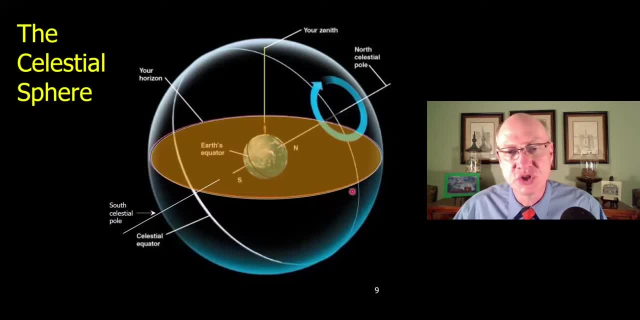 the south pole, the north celestial pole, the south celestial pole, This angle, right here, the altitude of the north celestial pole. that is sorry. here's this angle, right here, the altitude of the north celestial pole. that angle right there is 38 degrees. 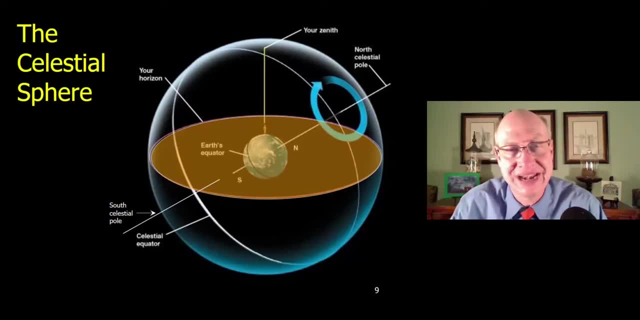 That is how high up the north pole appears in our sky. And you'll remember when we talked about measuring angles, that at out-at-arms length this is about 20 degrees. So if you do that, twice, start on your horizon. 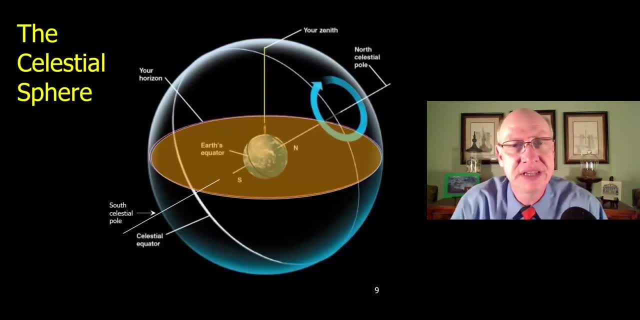 do it once, do it a second time. that gets you up to 40 degrees. So the north pole is just a little bit lower than that in the sky. Just to test some of your knowledge: that came out of watching lecture 05 on drawing the celestial sphere. 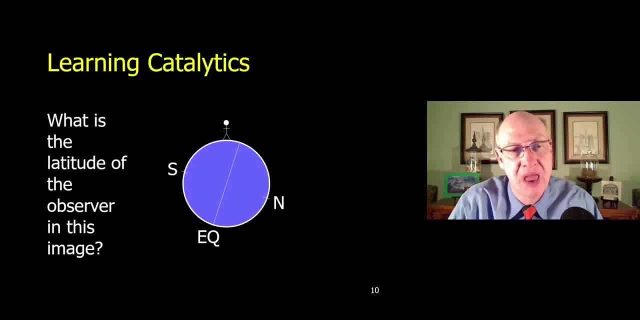 I want you to take a second to answer this learning catalytics question. What is the latitude of the observer in this image? So here we see an observer standing on top of the Earth. We see the poles and the equator drawn in. 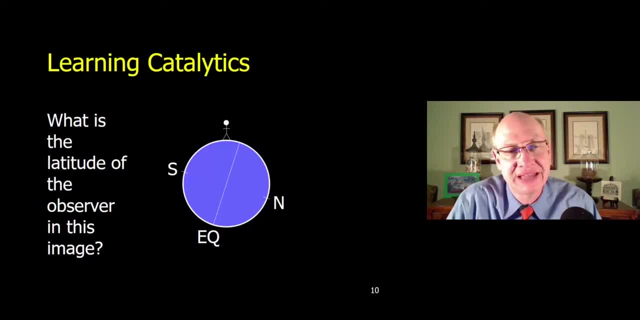 So I want you to take a second to answer that question. in learning catalytics, What is the latitude of the observer in this image? Okay, now that you're back from learning catalytics, just as a quick answer to this one, 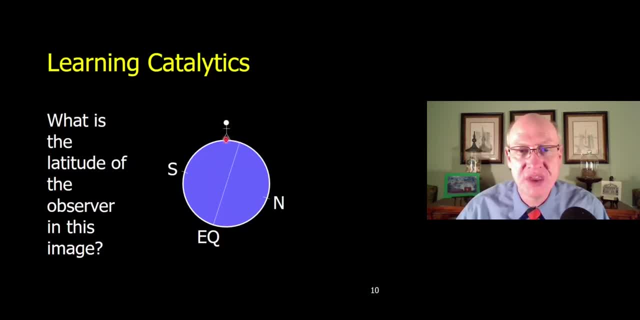 So our observer here is clearly standing south of the equator. That is because if I start on the equator, I have to walk towards the south to get to them, And they are closer to the equator than they are to the south pole. 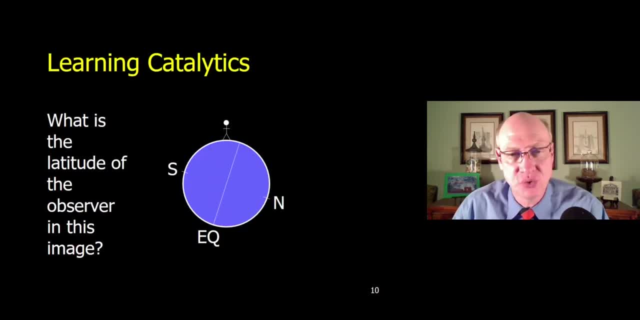 So, of the choices that you were given about 20 degrees south latitude is the best match to the location for this observer: 20 degrees south latitude. So just to go back and remind you, to refresh you on something that you learned in the lecture, 05 supplement. 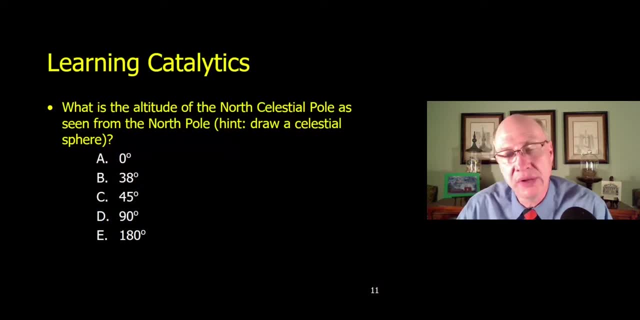 What is the altitude of the north celestial pole as seen from the north pole? So go ahead and take a second and answer this in learning catalytics. Imagine that you're standing on the north pole of the earth and you look up in the sky. 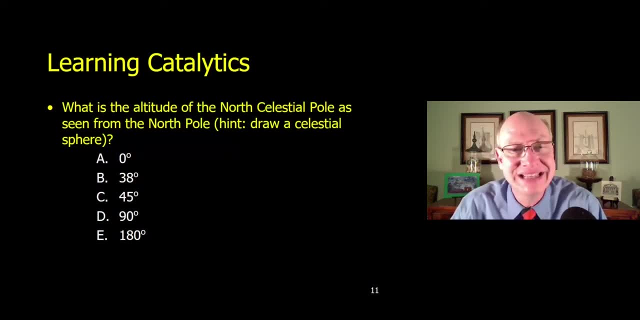 and you see the north celestial pole straight overhead. What is its altitude at that point? Okay, now that you've had the chance to answer the question, to go over the answer to this one. the answer is 90 degrees If I'm standing on the north pole. 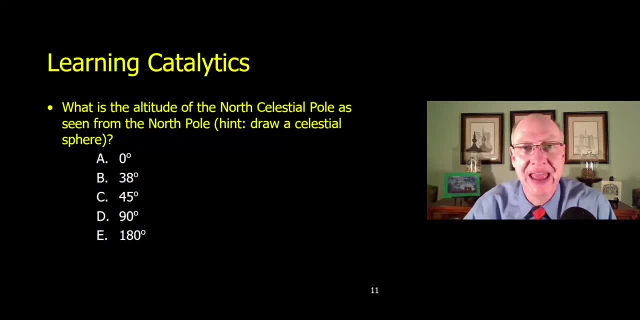 the north celestial pole is straight over my head. An altitude is a measure of how high something is above the horizon. I start on the horizon, which has an altitude of 0 degrees, and I go to the point straight overhead, which has an altitude of 90 degrees. 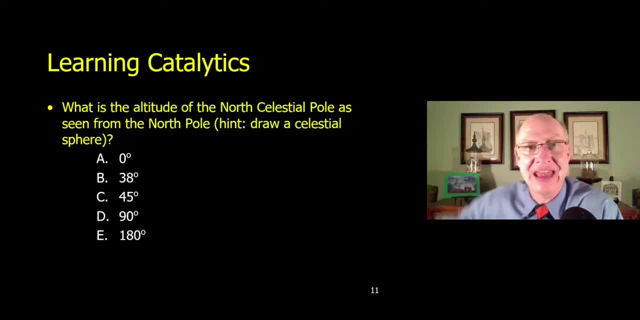 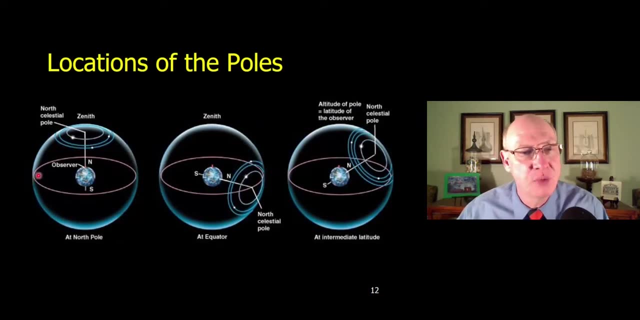 If the north pole is straight overhead, it has an altitude of 90 degrees. Here's another way to see that in this diagram. So here is a celestial sphere, And we're going to look at this celestial sphere on the left hand side, right here. 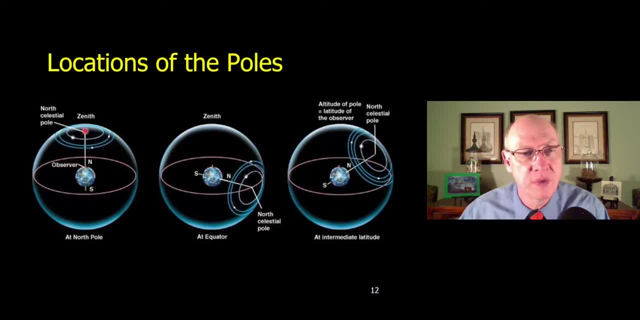 So the observer is standing on the north pole of the earth, So the north celestial pole is straight overhead. If I draw my horizon in here, that means that the altitude of the pole starting on the horizon and measuring up to the pole is 90 degrees. 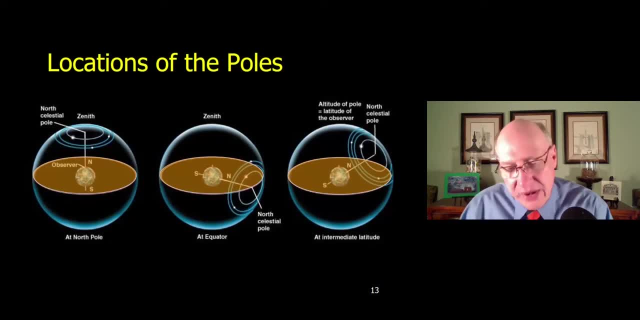 The altitude of the pole is 90 degrees. Well, when I'm standing on the north pole, my latitude is 90 degrees And the altitude of the pole is 90 degrees And, as we saw in lecture 5, supplement the altitude. 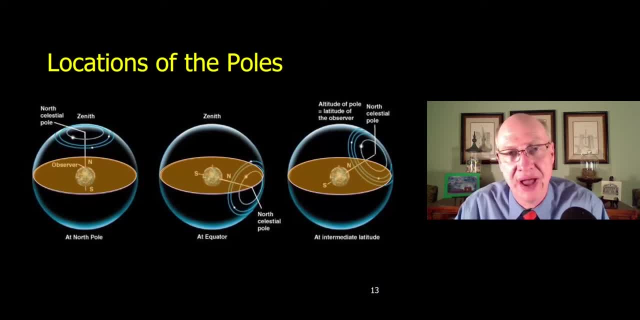 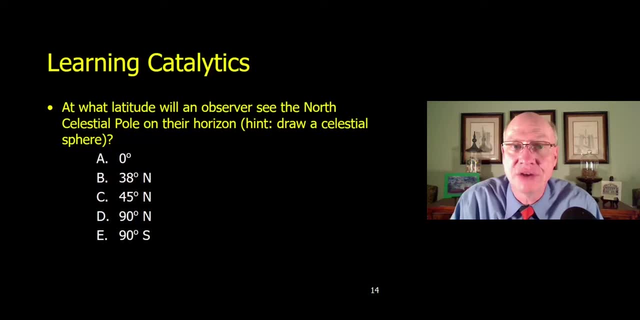 of your celestial pole is equivalent to your latitude on earth. Now I want you to think about this learning catalytics question for a second. At what latitude will an observer see the north celestial pole on their horizon? Draw a celestial sphere? So this is another great question. 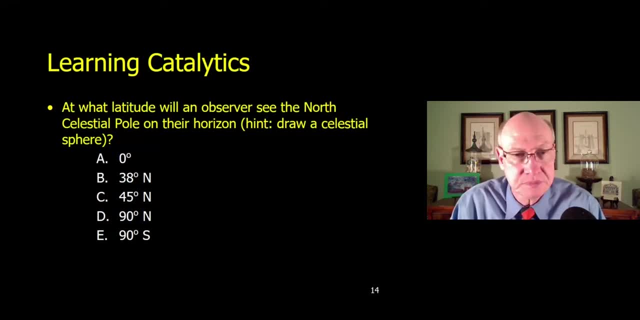 What latitude will an observer see the north celestial pole on their horizon? It's an interesting question, because to draw a celestial sphere you normally think of needing to know your latitude on the surface of the earth. But here I haven't given it to you. 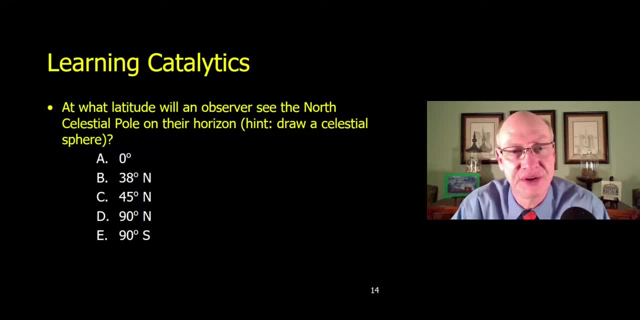 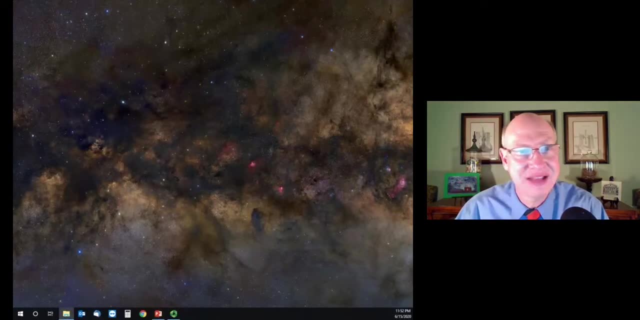 So, in this case, let me go ahead and play a video for you that shows you how to answer this question: How to determine your latitude on the surface of the earth. Okay, So for this learning, catalytic question, I'm going to go ahead. 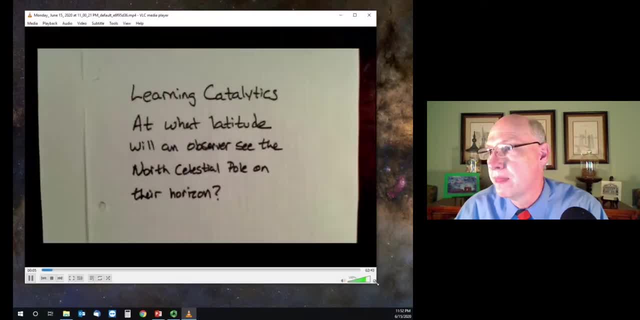 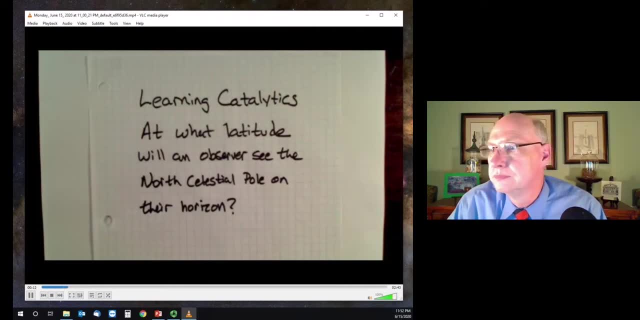 and ask you a question. The question is: at what latitude will an observer see the north celestial pole on their horizon? And the hint is: draw a celestial sphere. So let's draw a celestial sphere for this situation where an observer sees the north celestial pole. 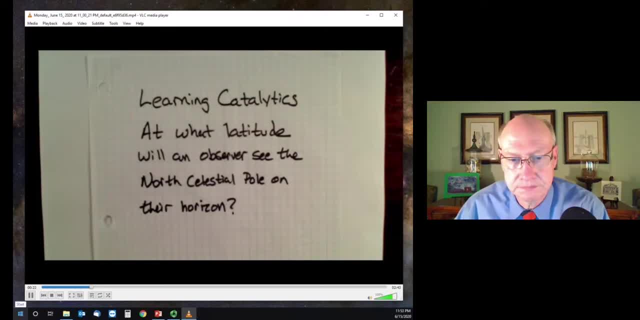 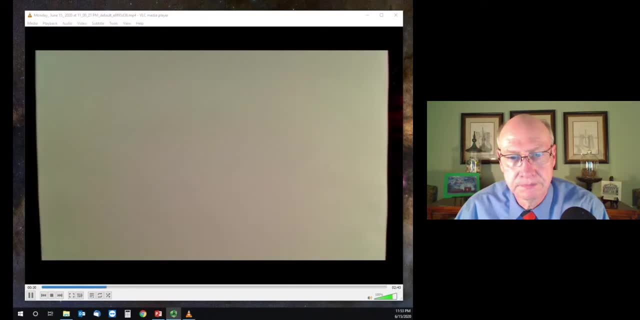 on their horizon and from that determine their latitude. This is a really interesting problem, because we don't know their latitude on earth, so we don't know how to orient the celestial sphere. But let's go ahead and stick to our steps and draw a celestial sphere. 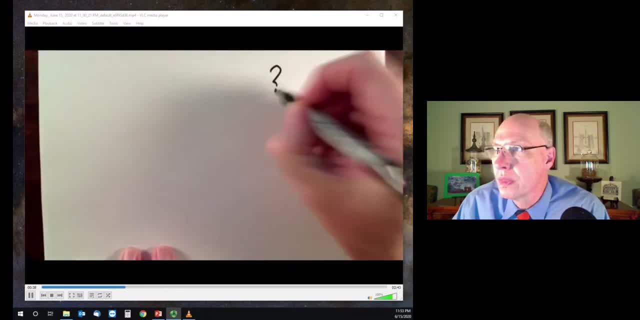 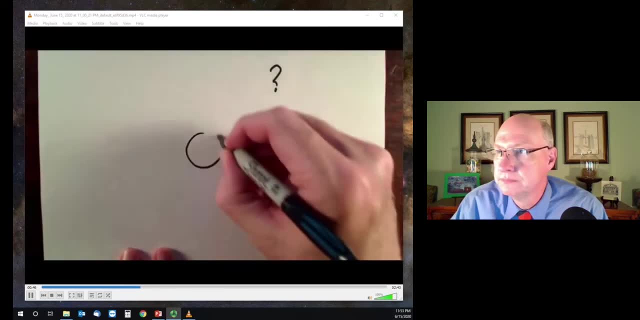 and see if we can figure it out. So the problem with this one is their latitude, is we don't know. But let's draw the celestial sphere anyhow, because there are certain things we can do. So we start by drawing the earth. Step one: we draw the earth. 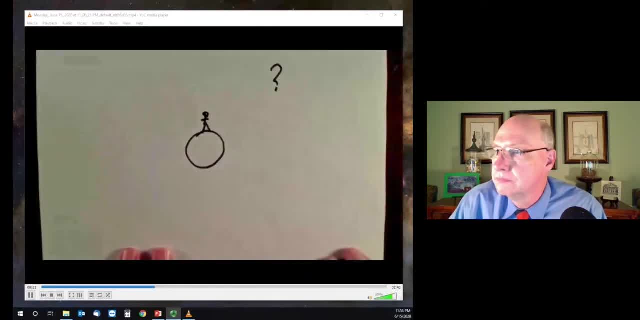 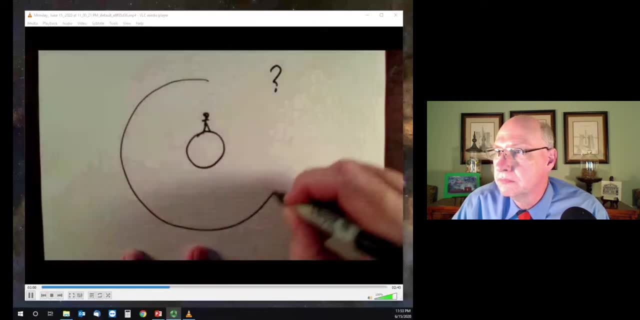 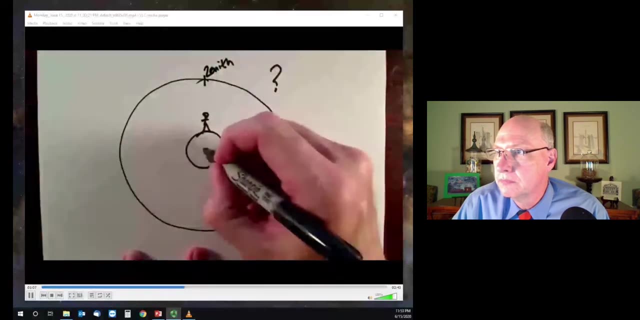 Step two: we draw our observer standing straight up and down on top of the earth. Step number three: we draw the celestial sphere around the observer and the earth. Step number four: we label the zenith, which is straight overhead, and the observer's horizon. 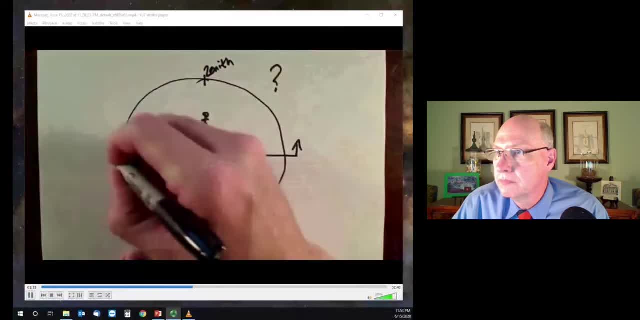 right here. Now step number five is where we run into trouble. Step number five is where we're supposed to orient the earth underneath the observer knowing their latitude on the surface of the earth. But we don't know the latitude. so how do we orient the earth? 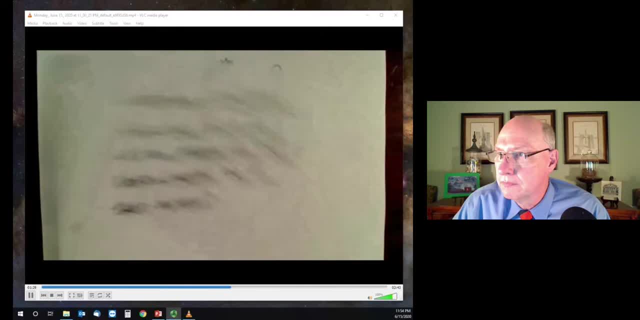 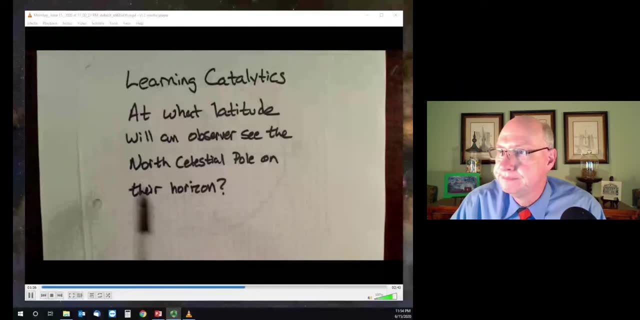 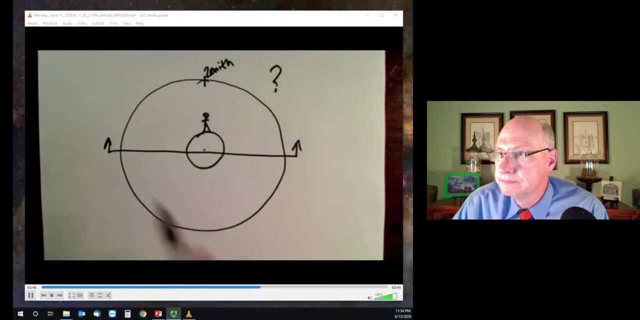 Well, the question gives us a hint. The question says: at what latitude will an observer see the north celestial pole on their horizon? So the hint is that the north celestial pole is on their horizon. So let's draw that. Here's the observer's horizon. 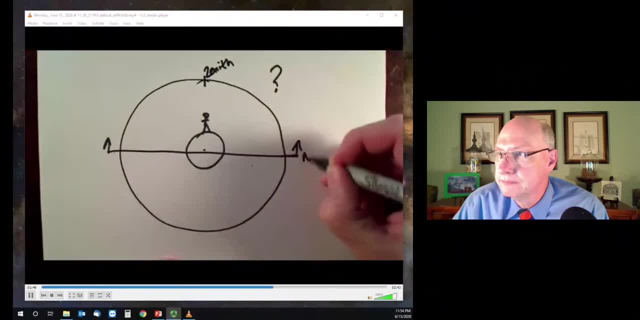 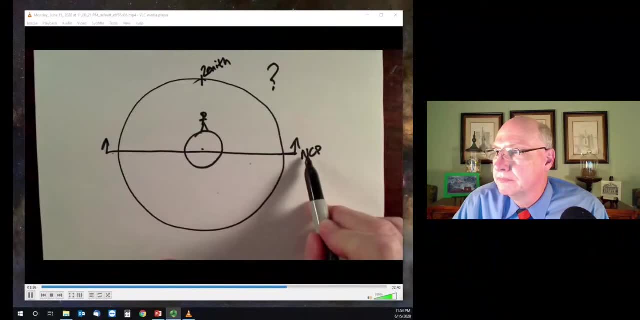 The north celestial pole is on the horizon, which means that this is the north celestial pole. I could have put it over here as well, Doesn't matter, I'll get the same answer either way. If that's the north celestial pole, that means that this is the south celestial pole. 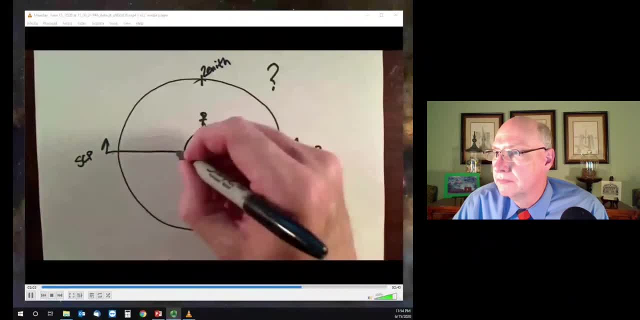 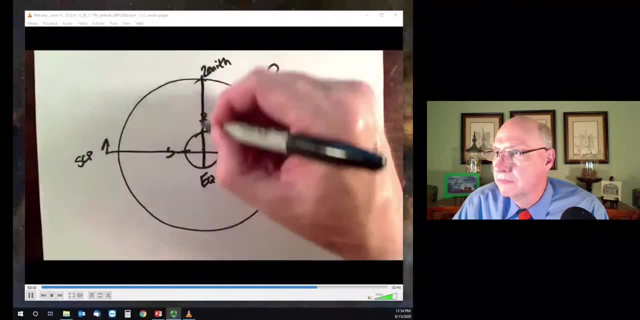 which means that this is the earth's north pole and that is the earth's south pole, And at a right angle to the earth's poles, we have the equator, and that means that this, of course, is the celestial equator, And that means that for 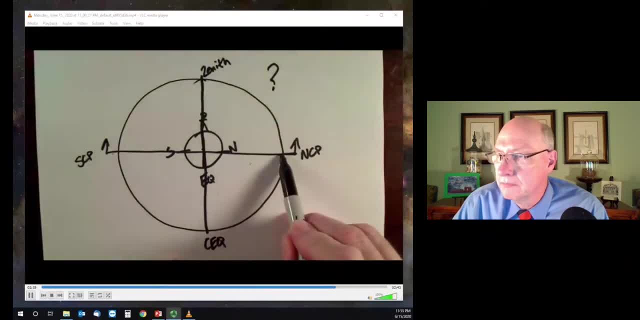 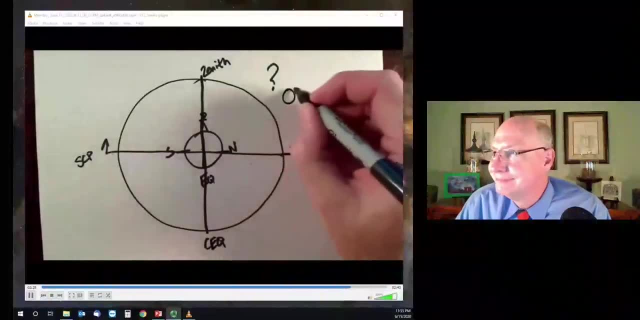 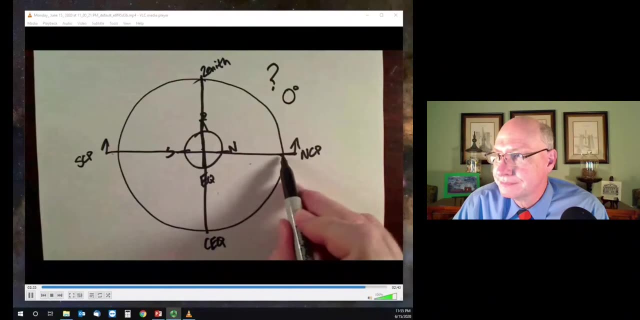 an observer to see the north pole on their horizon, they must be on the earth's equator, and to be on the earth's equator, you have a latitude of zero degrees. And so the answer to this one is: at what latitude will an observer see the north celestial pole? 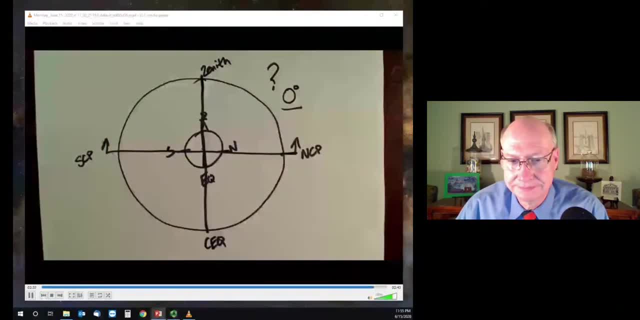 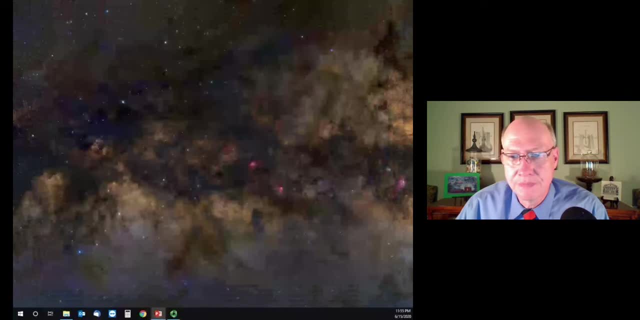 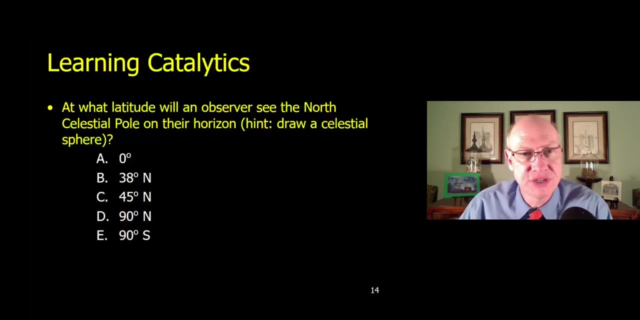 on their horizon. The answer is zero degrees on the equator. Excellent. So the answer to that learning catalytics question is: at what latitude will an observer see the north celestial pole on the horizon? It is zero degrees And that is depicted in this case. 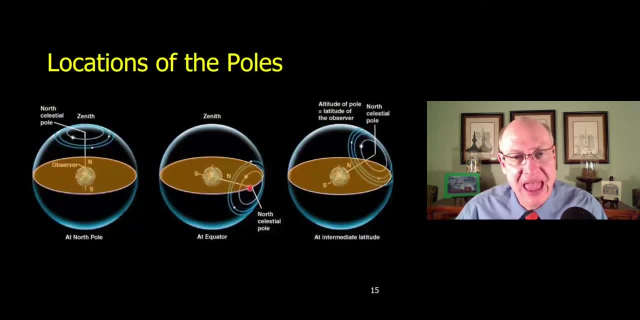 right here. So here is an observer standing on the equator, and you'll notice that the observer is again depicted straight up and down. The zenith is straight overhead. The orange circle represents their horizon. They can see everything above the horizon, but they can't. 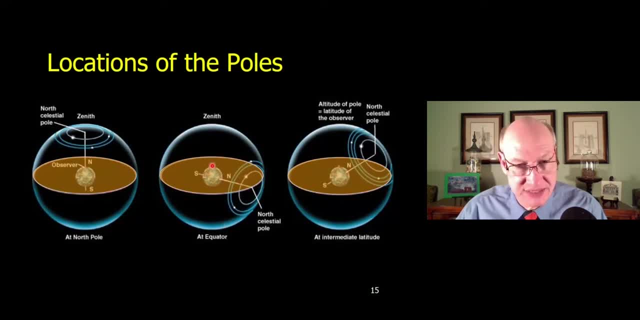 see anything down here below the horizon. But in this case, because they are standing on the equator, the north celestial pole is right there on their horizon, And so what happens here at an intermediate latitude? For example, what happens here in Charlottesville? So what is? 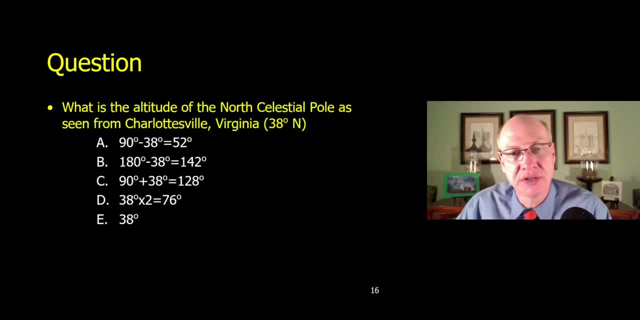 the altitude of the north celestial pole as seen from Charlottesville at a latitude of 38 degrees north. Now that you've watched the Lecture 5 supplement, you should be able to answer this one, So let me give you a second to answer it. But what is the? 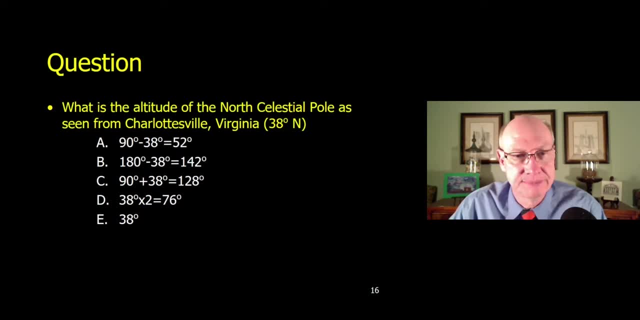 altitude of the north celestial pole as seen from Charlottesville. Okay, Hopefully you got this one fairly quickly, having seen Lecture 5 supplement, And the answer to this is 38 degrees. The altitude of the celestial pole in your sky is equivalent to the latitude on Earth, And 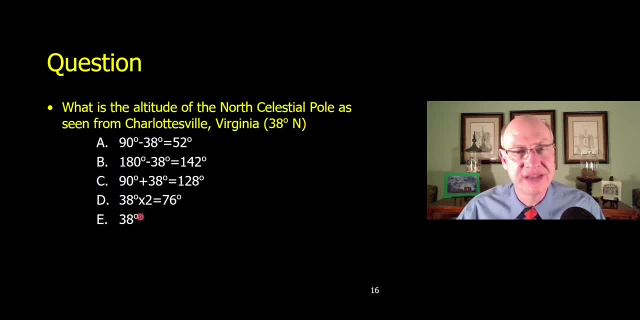 because we are at 38 degrees north. the pole is 38 degrees up in our sky. Also in Lecture 5 supplement we covered what is the altitude of the celestial equator as seen from Charlottesville. So I'm not talking about how high the pole is, but 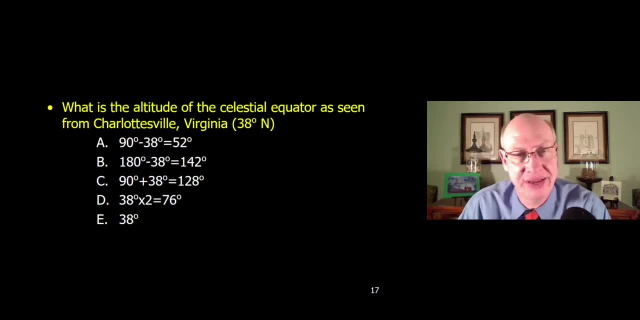 on the other side of the sky. I'm asking how high the celestial equator is, And so you might remember from Lecture 5, supplement to calculate that We go up to the pole. We know that the angle from the pole to the equator is. 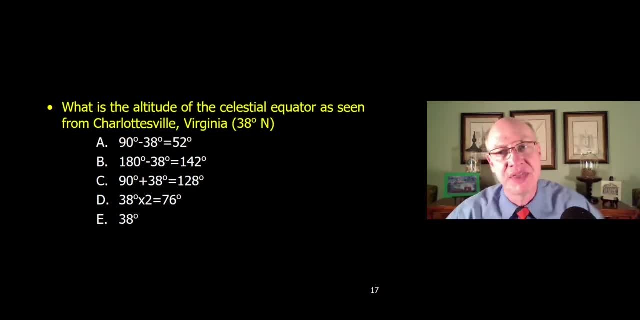 90 degrees, and that allows us to calculate how high up the equator is in the sky. So take a second to answer this one. What is the altitude of the? And sorry, this is in Learning Catalytics, I'm missing the words right there, but this is. 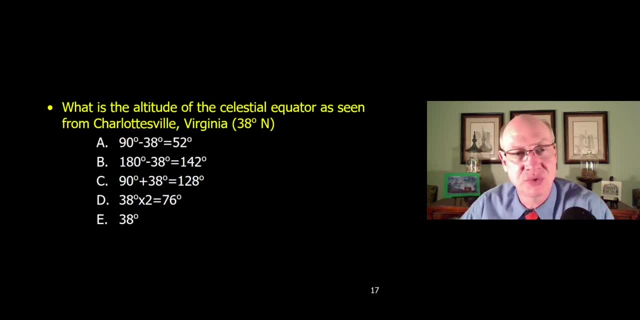 another Learning Catalytics question. Please answer this one in Learning Catalytics right now. What is the altitude of the celestial equator as seen from Charlottesville? And the answer to this one is, of course, A. It is 52 degrees. 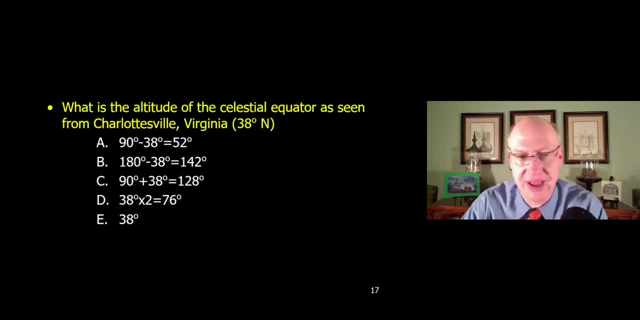 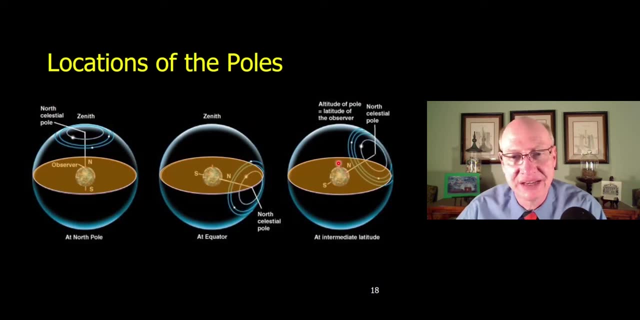 up in the sky. The celestial equator is 52 degrees up, And this is the depiction of what's going on. So here we are in an intermediate latitude. Here we are standing straight up and down. The zenith is straight overhead. There is the north. 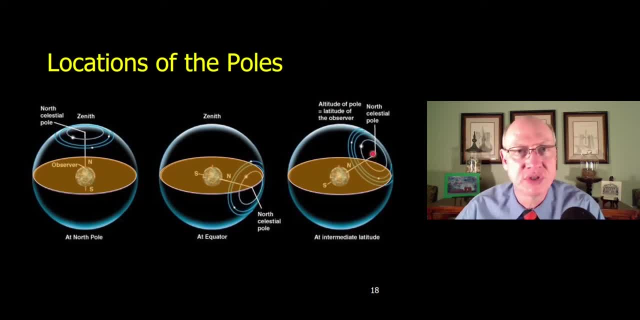 celestial pole in the sky, And here in Charlottesville the north pole is 38 degrees up. The celestial equator runs from over here in the east across the sky, sets over there in the west. So the equator is running across the sky like this. 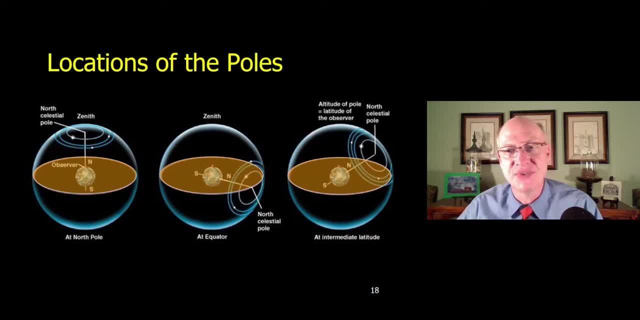 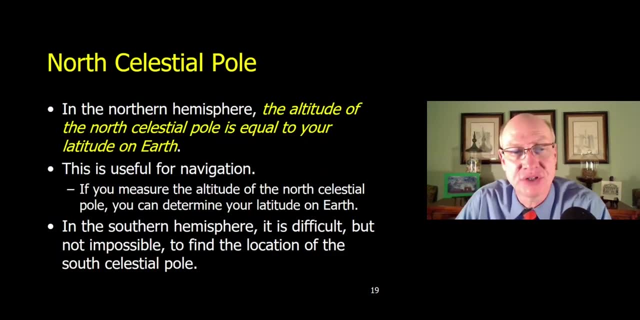 and the maximum altitude of the equator right there is 52 degrees. So in the northern hemisphere, in the northern hemisphere, the altitude of the north celestial pole is equal to your latitude on Earth, And this is extremely useful for navigation If 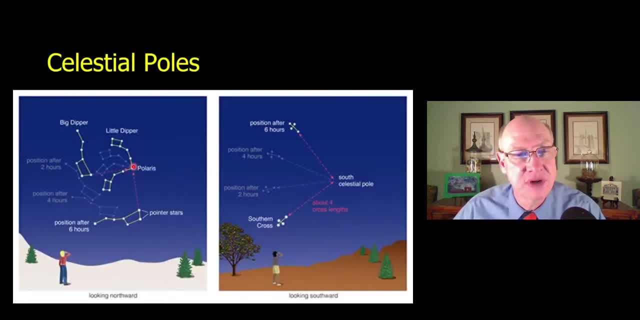 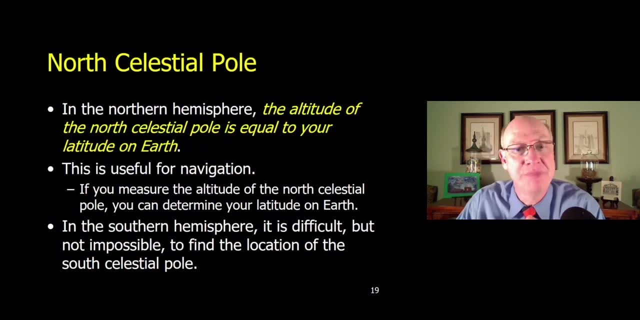 you can go out in the sky and you can find the north star Polaris and you can measure how high the north star Polaris is in the sky. you will be able to measure your latitude quite accurately on the surface of the Earth. 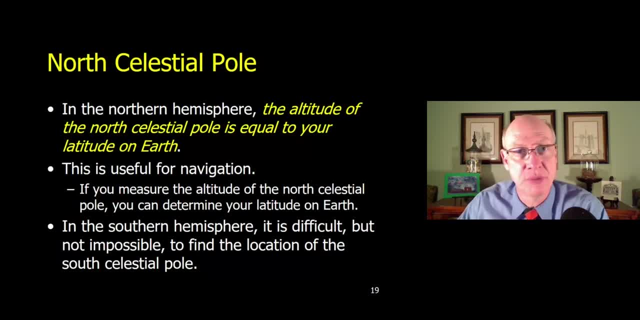 You can use something like a sex tent to measure the altitude of the pole. A sex tent is simply a device for measuring very accurate angles in the sky. It's used by navigators all the time. You can think of it as simply a very accurate compass. 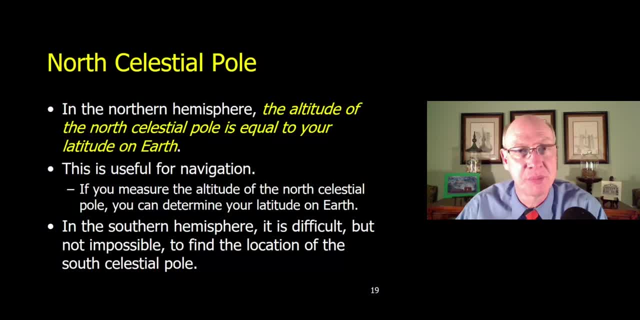 that you might have used, or protractor- sorry, a very accurate protractor that you might have used in high school geometry class. There are older devices: Sex tents use a low-power telescope with them. There are older devices called quadrants, for example, that. 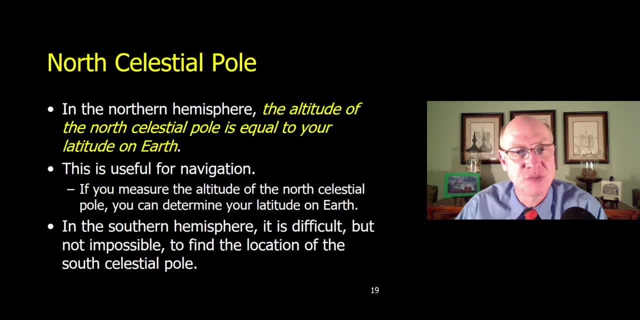 didn't use telescopes for doing this, But this is a fact that has been known in navigation for a very long time: that if you measure the altitude of the pole in your sky, it tells you your latitude on Earth. By the way, you can do exactly the same. 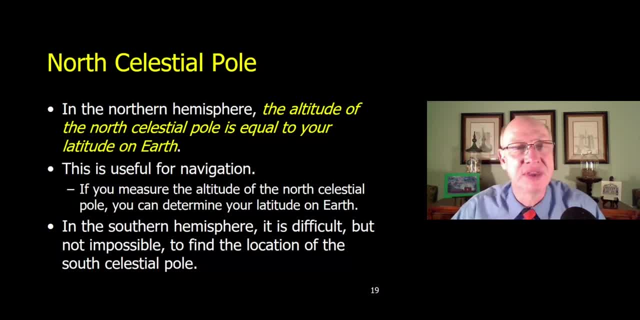 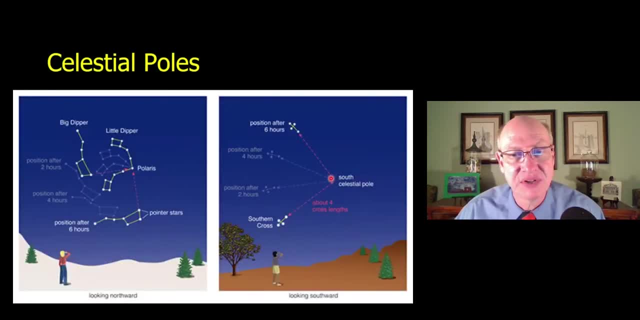 thing in the southern hemisphere. If you measure the altitude of the south celestial pole in the sky, it is the same as your latitude. As we saw in the last lecture, it's a little bit difficult to find the south celestial pole in the sky because there is 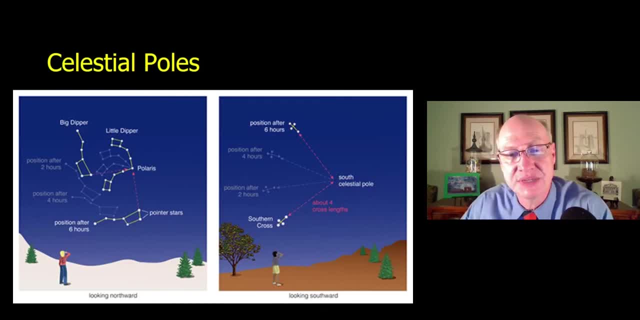 not a moderately bright star there like there is in the northern hemisphere, But you can find it and with a little bit of work or a telescope you can locate some of the stars close to the south celestial pole, or you can use the movement. 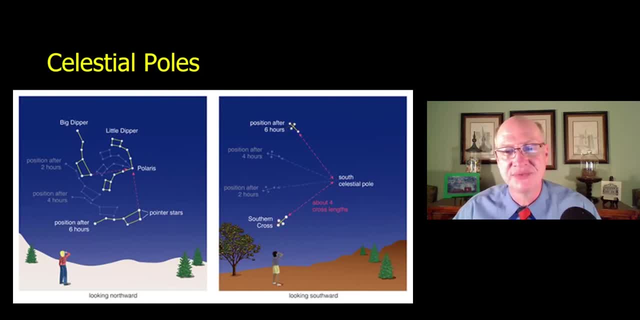 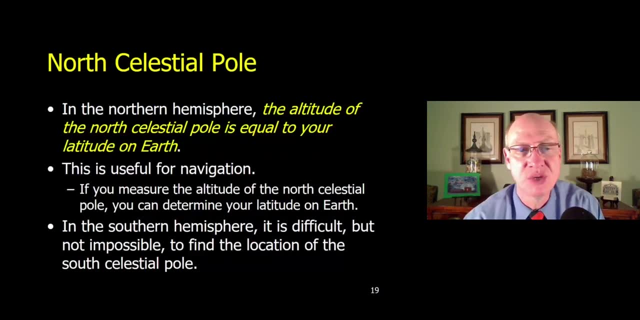 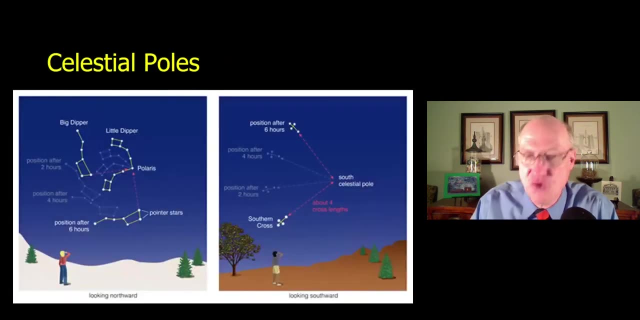 of the southern cross over a period of about six hours to identify where the south pole is. This feature- that the altitude of the north celestial pole is equal to your latitude on Earth- actually explains something really interesting about old maps of the Earth You've probably seen. 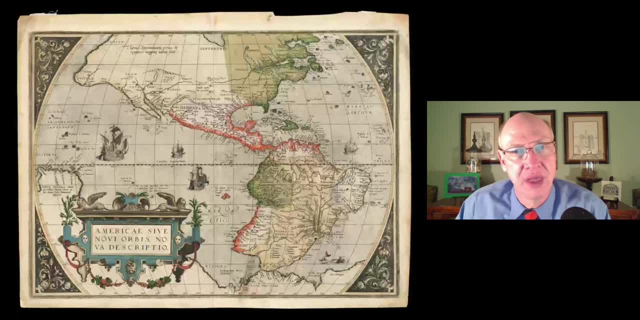 in history class these old maps of the New World. when navigators first started setting sail for the New World, the first thing they wanted to do is map the New World, And these maps are sometimes almost hilariously in error If you look at. 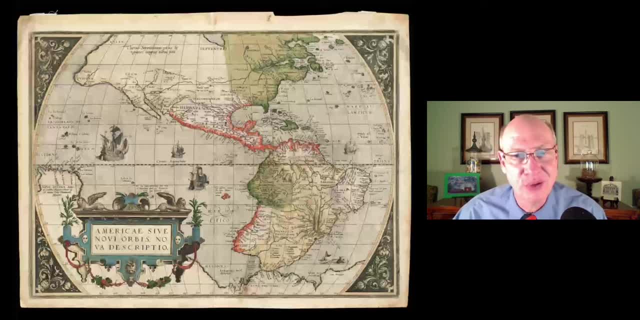 the distortions of North America right there. you can see how small Florida is right there, how big Baja California is, just how grossly distorted South America is down there. It looks initially at a first glance that all the content are grossly 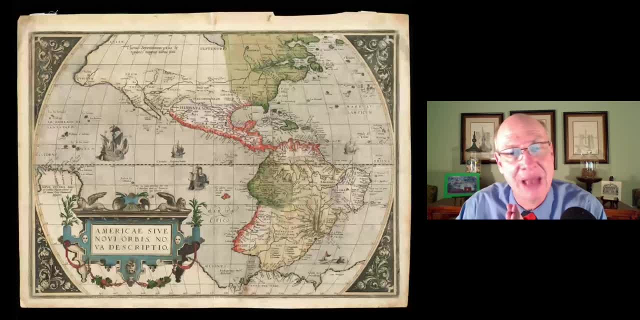 misshapen. But there's an interesting thing about these maps: If you look very carefully, the latitudes of everything are exactly right. It's the longitudes that are wrong And the latitudes are right because ancient navigators all 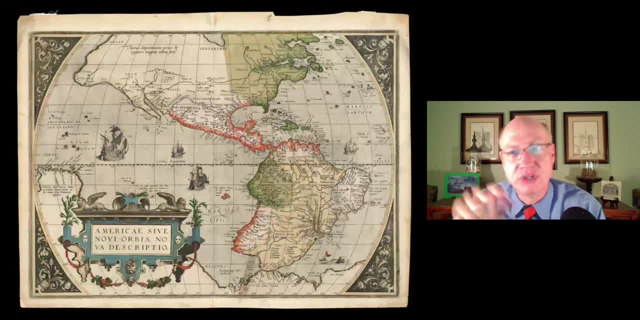 they had to do when they were standing on the deck of their ship was measure the altitude of the north pole in the sky, measure from the horizon up to the north celestial pole, and that would tell them their latitude on the surface of the earth very, very. 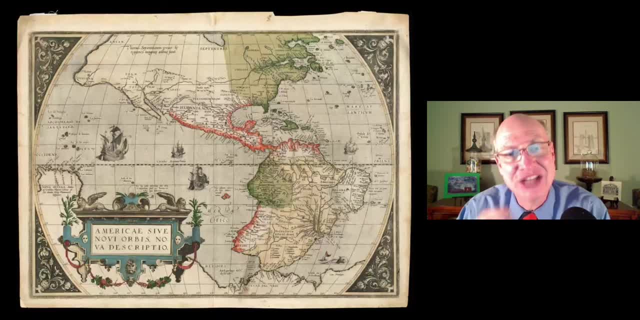 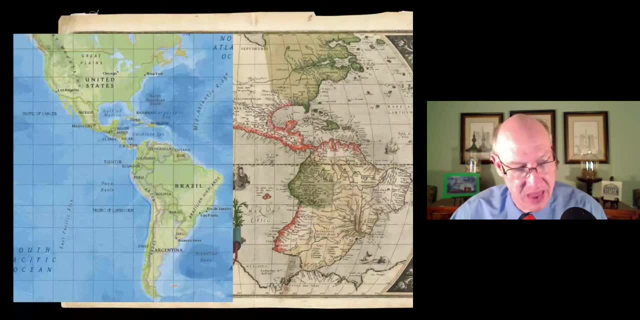 accurately. So if we look at this map for a second, it's remarkable how accurate the latitudes are. To show you, let's compare it to a modern day map. So, for example, notice that on this map right here, so here's the equator, here's 10 degrees north. 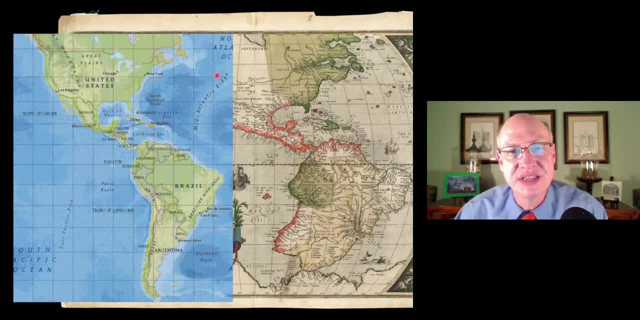 20 degrees north, 30 degrees north, 40 degrees north. So these are the lines of latitude. right here Let's look at the northern coast of the Gulf of Mexico. So the northern coast of the Gulf of Mexico is at a latitude of about 30 degrees. 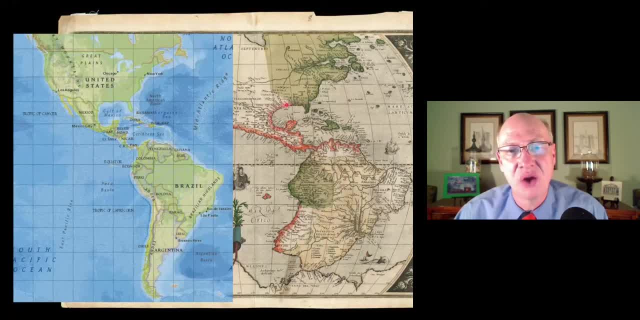 north latitude and you'll see on this map they got it right at about 30 degrees north latitude. The southern tip of Florida is at about a latitude of 25 degrees and if you look here, the southern tip of Florida is at a latitude of 25. 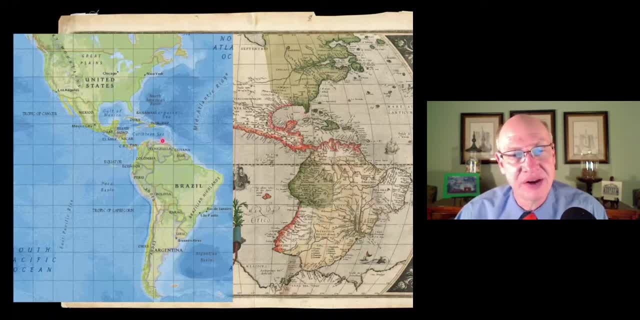 degrees, The north coast of South America. right there is a latitude of about 12 degrees or so, a little more than 10 degrees, and they got it in exactly the right place. Even if we go far north on the globe up here, we can see that they got the. 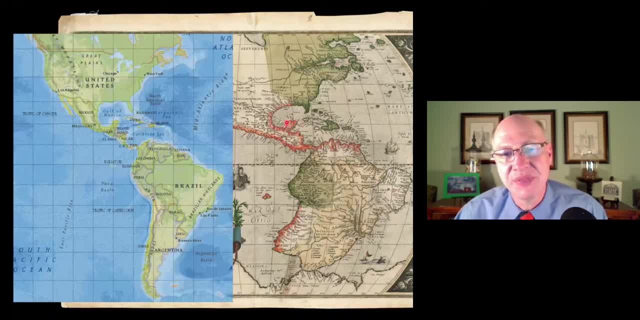 latitudes of everything correct. Even, for example, the Yucatan Peninsula is at the correct latitude. They got the latitudes correct because all they had to do was find the north pole in the sky, measure its altitude. and when they were, 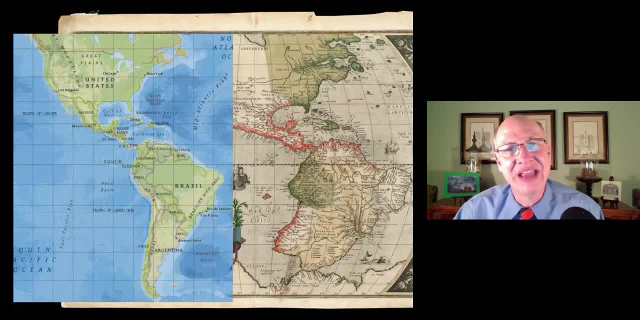 sitting off the coast of South America. here they could very accurately measure their latitude. What they couldn't measure was their longitude, Because the Earth is turning. in order to measure longitude, you need to know the time very, very accurately, And these early 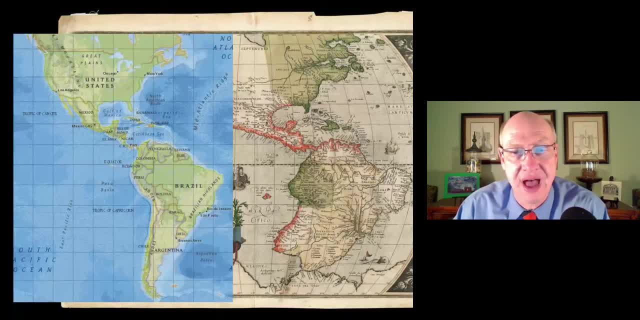 navigators did not have access to good clocks, And because they didn't have access to a good clock, they could only use very, very crude methods for measuring their longitudes on Earth. So I think these maps are fascinating, and they're fascinating because the 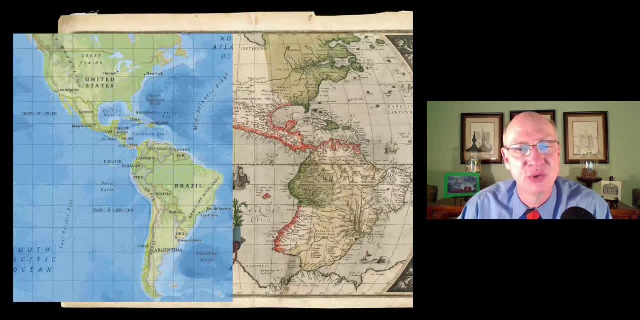 latitudes are almost exactly correct, but it is the longitudes that are off. and the longitudes are off because they didn't have a good way to measure them. So that ends Lecture 5, and you've learned all about the celestial sphere. now In the 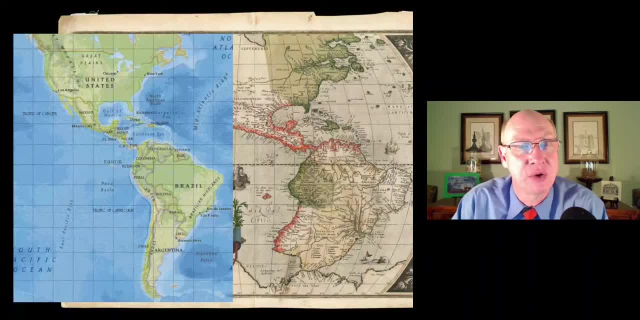 next lecture we're going to talk about what happens as the Earth turns, As the world turns and the stars move across the sky. we will see what the movement of those stars look like and how that varies with your latitude on Earth. So thank you for joining me for Lecture 5..